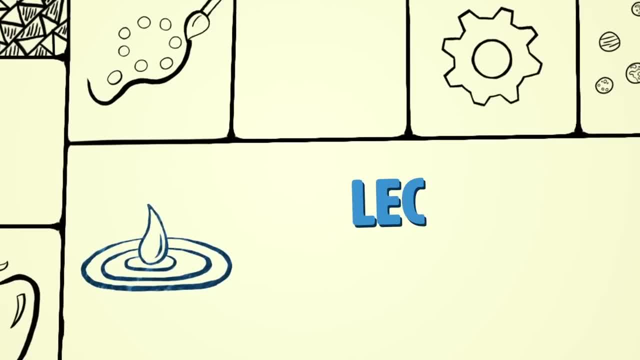 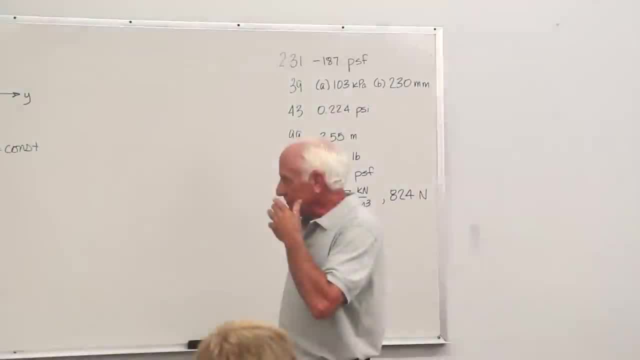 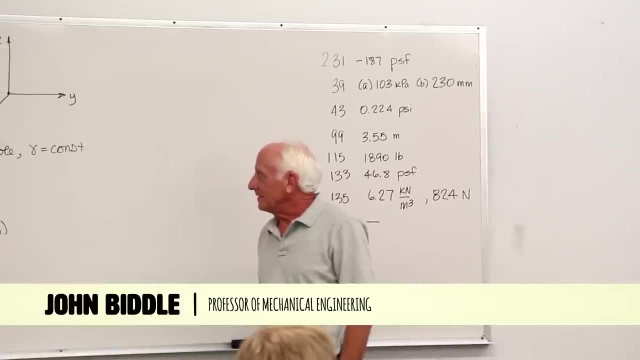 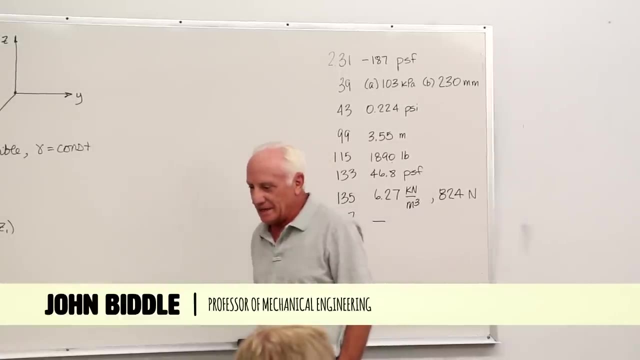 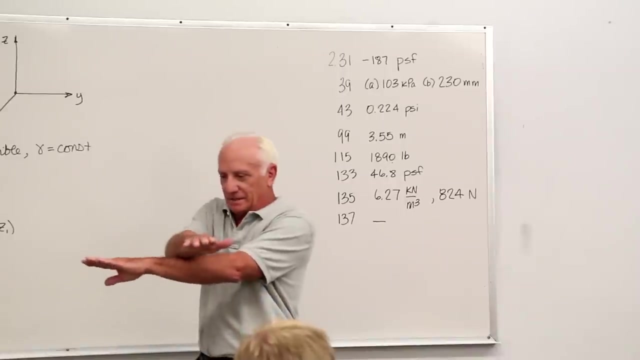 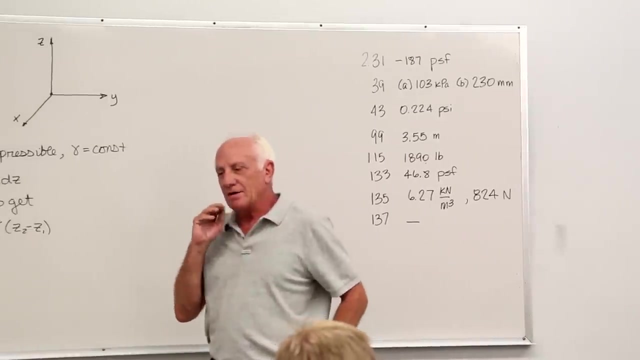 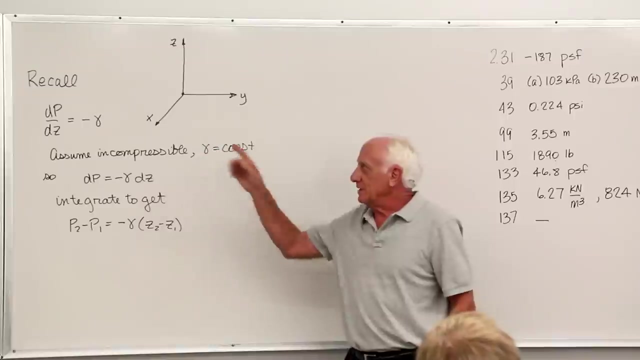 I want to go back to our last lecture and go back and emphasize this a little more. We were looking at how the pressure varied in a static fluid and we said it doesn't vary in horizontal planes, Which are x and y planes. here One direction is x, one direction is y. So the pressure doesn't vary in horizontal planes. But we found out that the pressure did vary in the vertical direction, which is the z direction. So there was the equation that we derived in class last time. We're going to integrate that, assuming that it's an incompressible fluid. So gamma is constant, doesn't vary. 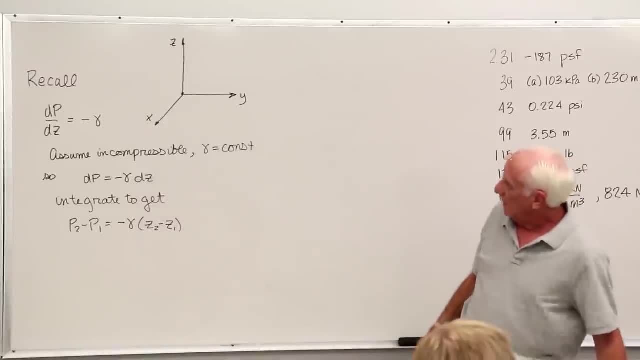 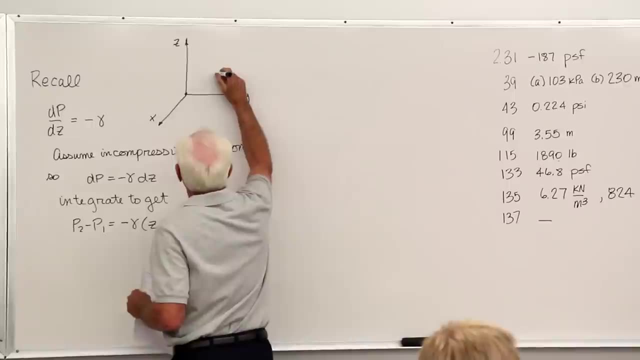 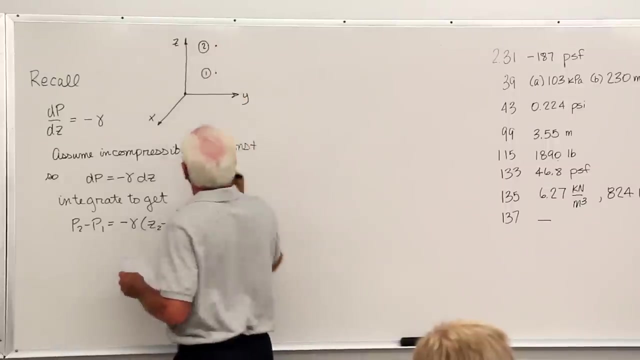 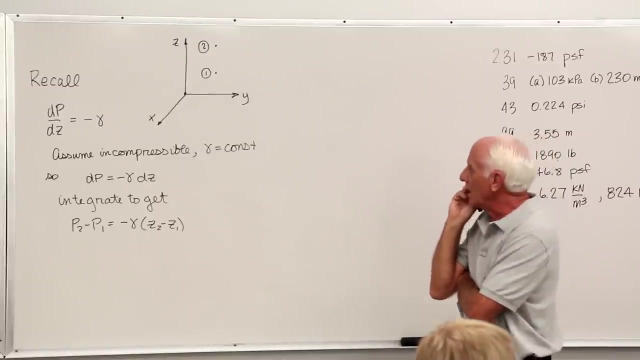 Here's the setup, Here's the integration. We're going to take our point one, For instance, take point one here And then take point two up there. So p2 minus p1 minus gamma, z2 minus z1.. Now z2 minus z1, we're going to call that. 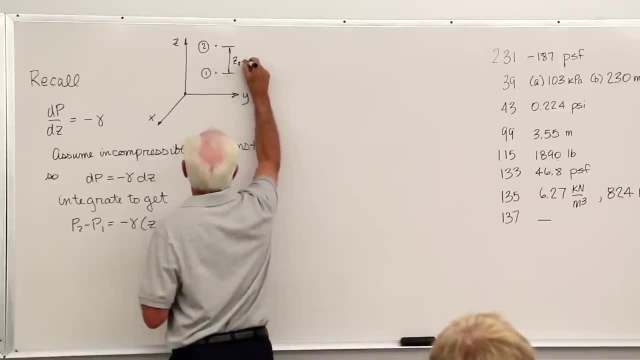 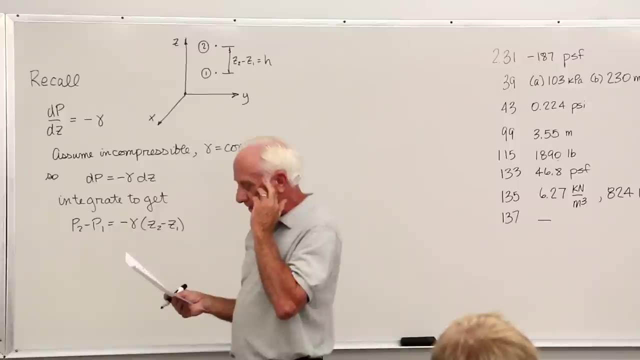 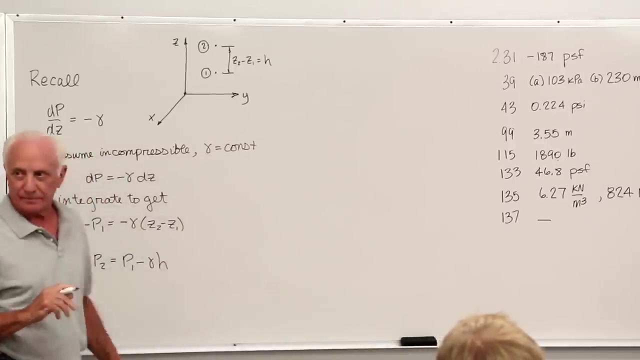 h. So z2 minus z1 equals h. Okay, I think that's all we need. So wherever you see a z2 minus z1, put an h in there. So p2 equals p1 minus gamma h. Grab that, Dorothea, Will you pardon me? 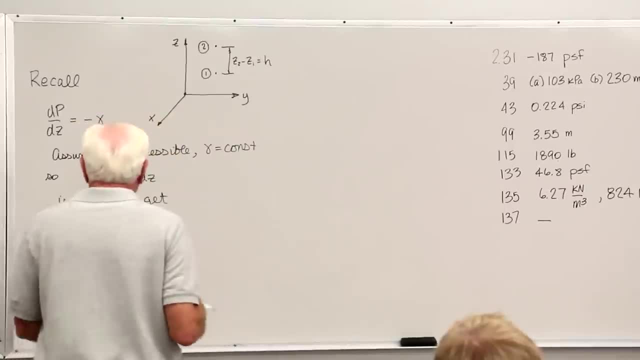 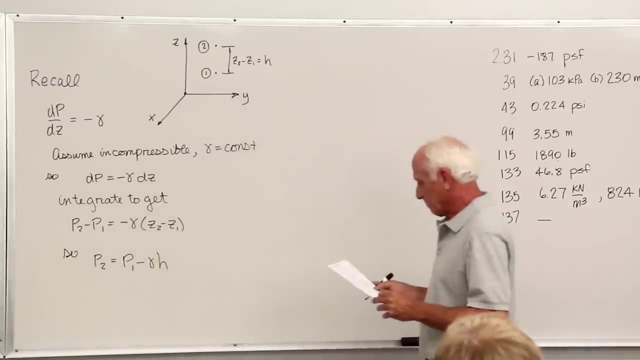 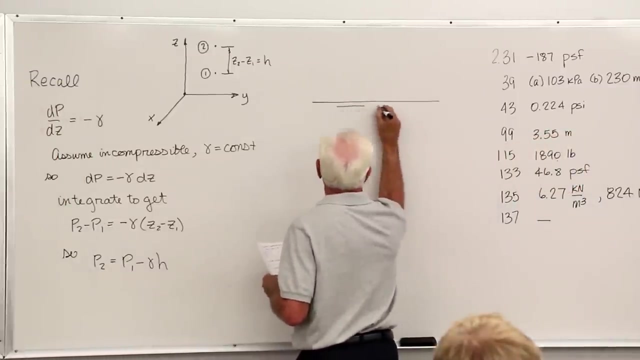 Close that. Oh, close it for me. Okay. So I left p2 over here, I put p1 over here, minus gamma and that's h. So here's two pictures. Here's the free surface of liquid air up there, or gas up there, called air. 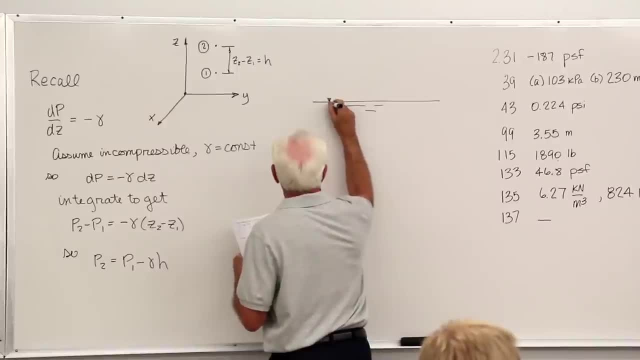 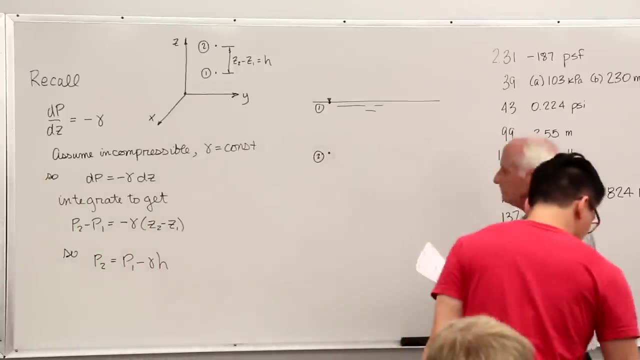 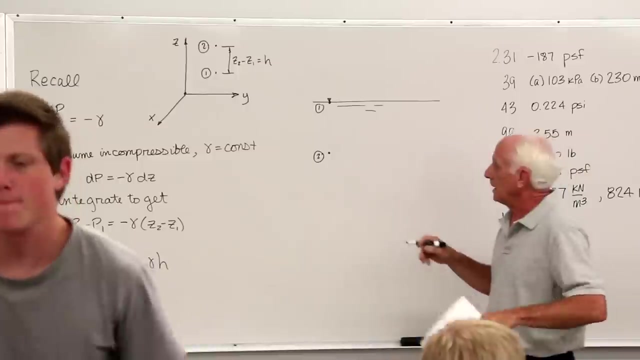 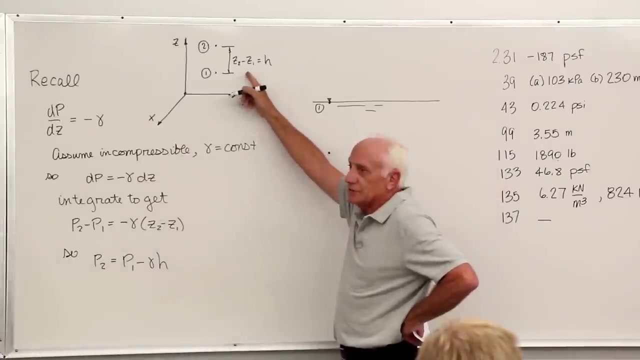 I'm going to call this point one. I'm going to call this point two. Now we know, as we go down in the fluid, that the pressure should go up. Okay, Look at what h is. h is z2 minus z1.. 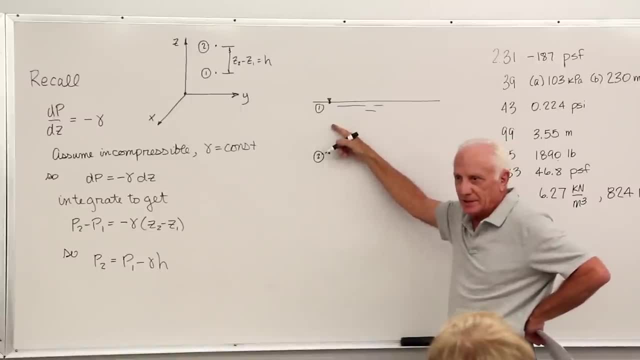 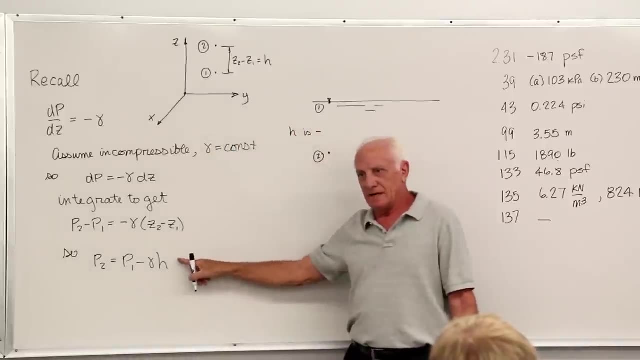 z2 minus z1.. h is negative, h is negative. Put a negative. h is negative. So we're going to put a negative sign for h here. p2 equals p1 plus gamma times the absolute value of h. So yes, it does get bigger. 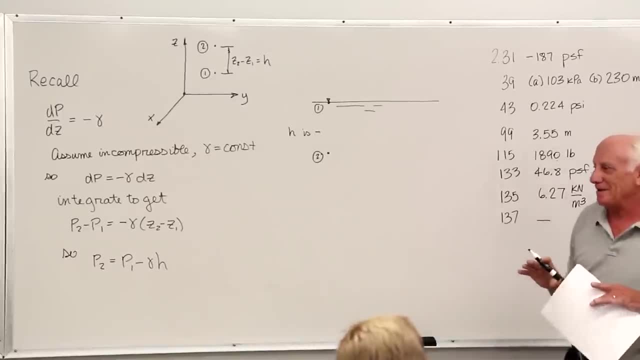 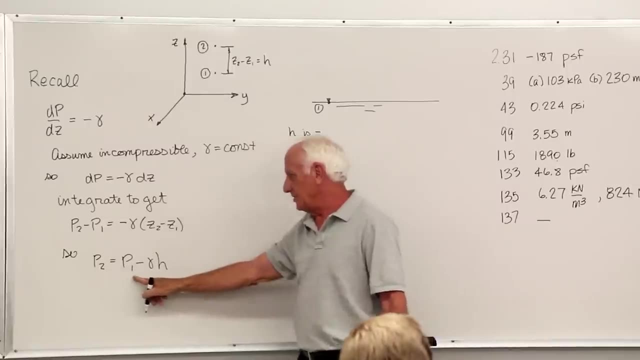 I'm trying to say this. It's a little bit tricky in a way, or you have to kind of pay attention to the ones and the twos here. That minus sign might confuse some people, But down here the equation you use. well, take one here. 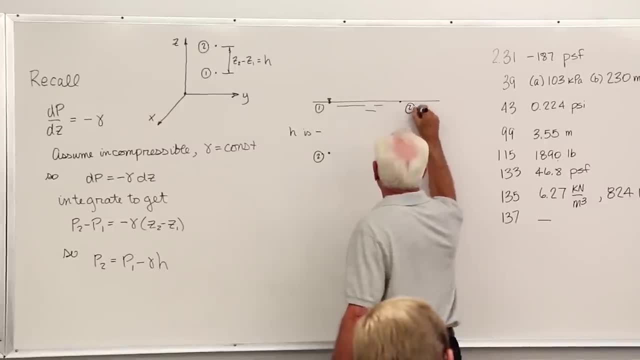 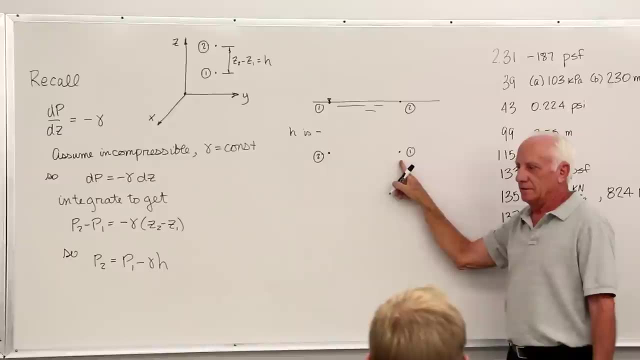 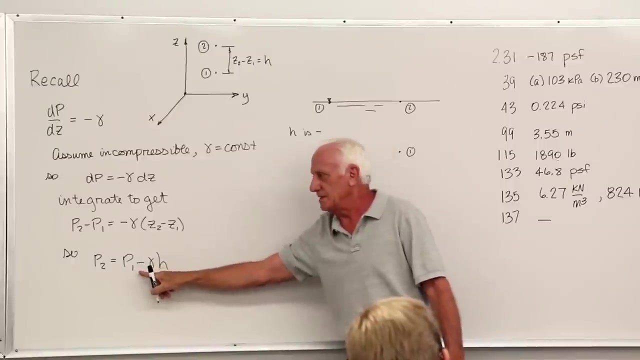 Take two here: z2 minus z1, z2, zero, z1 minus something, z2 minus z1, a positive number, but a positive number for h. What happens? The pressure goes down from p1.. Sure, here's p1.. 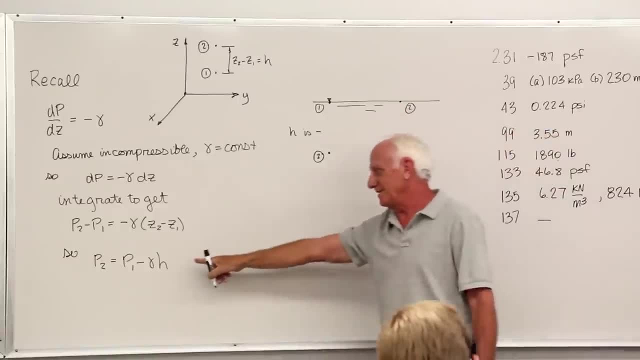 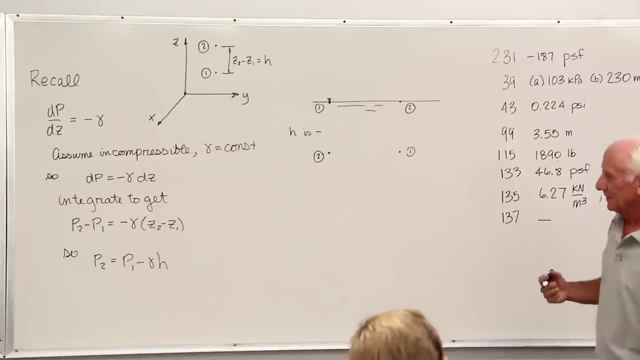 If we go up here, the pressure goes down. So this equation does make sense. but if you do it mathematically, watch out for the ones and the twos and things like that. Okay, so we just kind of plop this equation down from here. 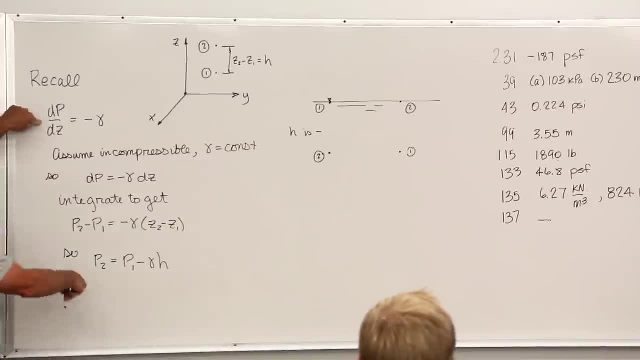 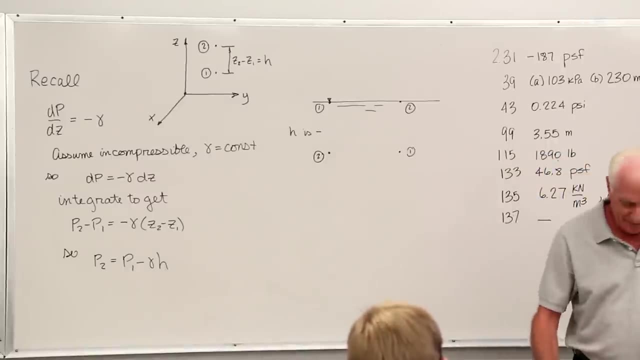 And down from here to here. last time I didn't go through all the gory details, so there are all the gory details with these animals All right now. as I said last time, that pretty much is the first half of chapter two. 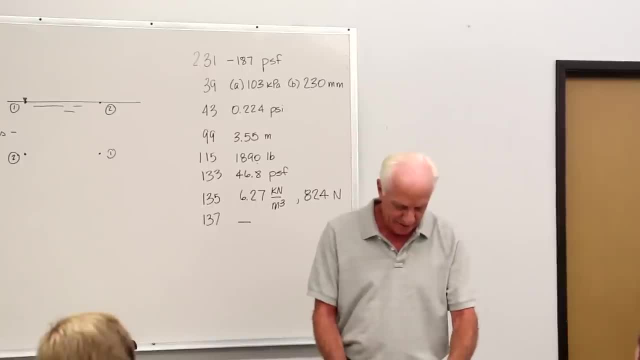 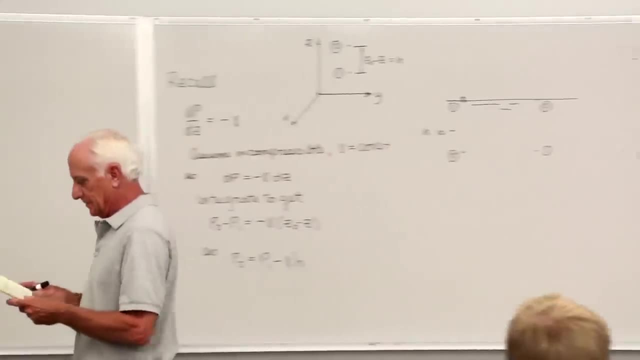 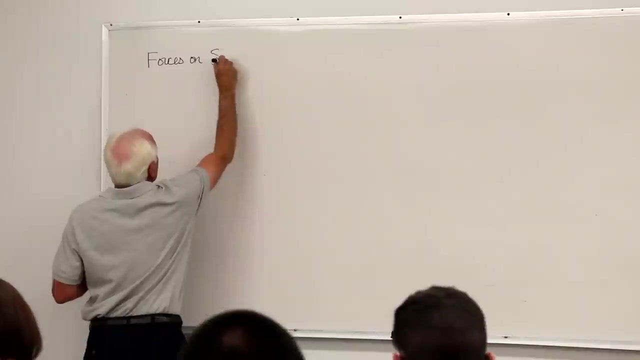 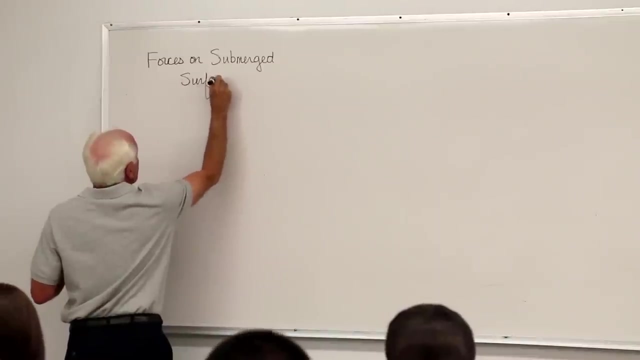 So now we're going to look at the second half of chapter two, which is forces on submerged plane surfaces. There's a real good picture in the book. I'm going to draw it up here on the board, but it's very similar to what's in the textbook. 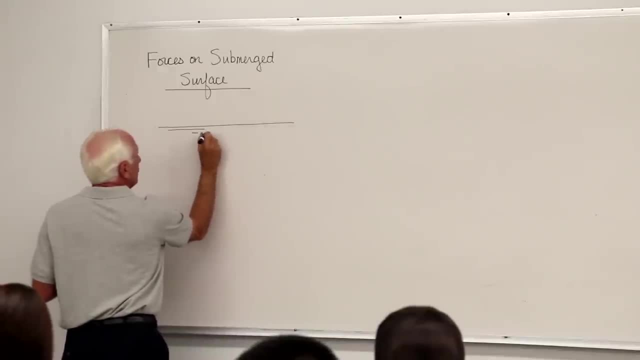 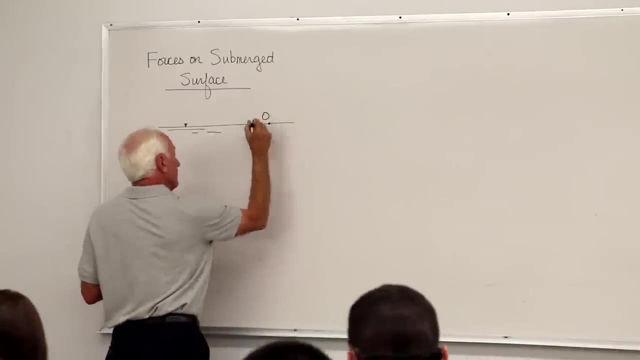 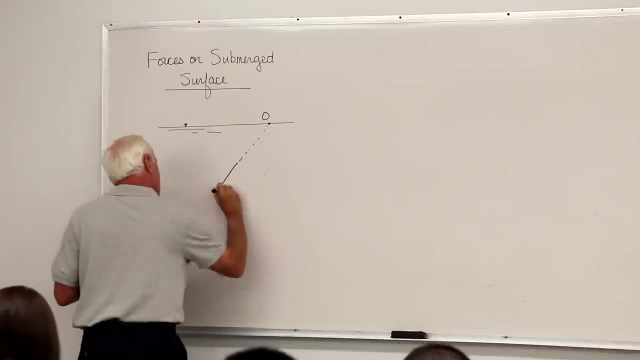 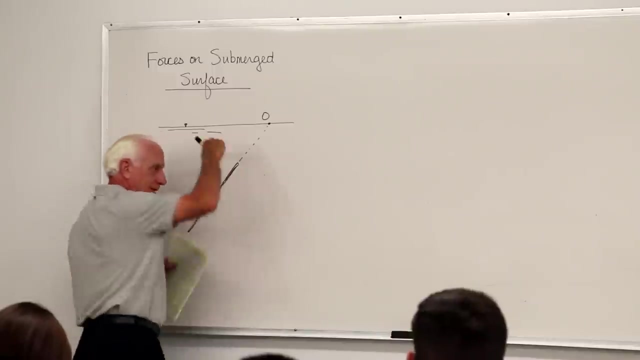 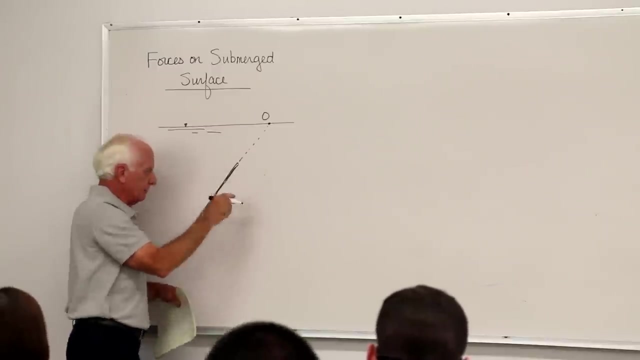 Again, here's some liquid with a free surface. We're going to call that point zero coordinate system axis All right Down here. this is the surface. It's a submerged surface And if you look at it from above- normal to the surface, look down on the surface from above normal to the surface- it might have a shape. 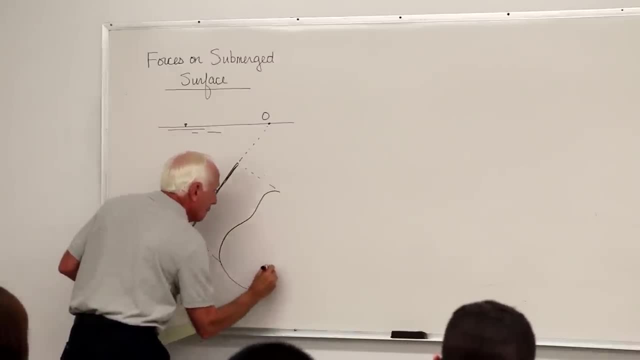 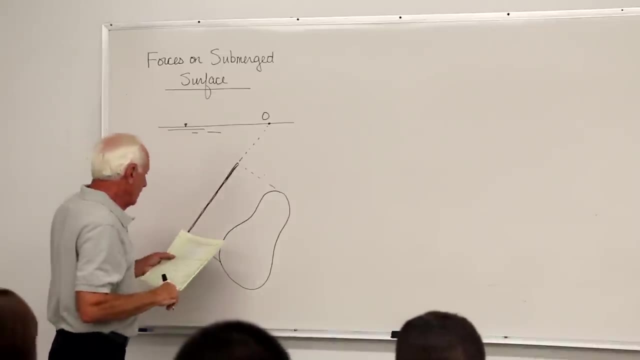 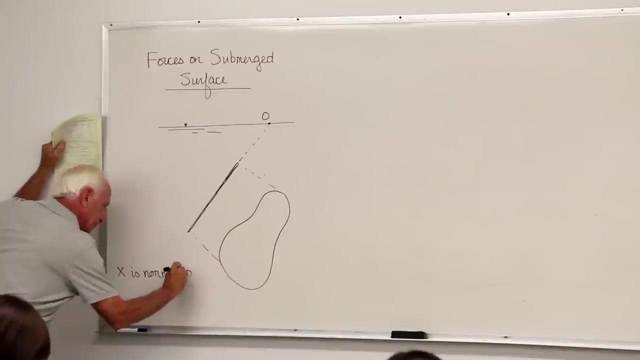 Something like this Arbitrary shape Looking down from above. From above, We call the x-axis into the blackboard. X normal to board. The y-axis: we measure down to the blackboard. The y-axis: we measure down to the blackboard. 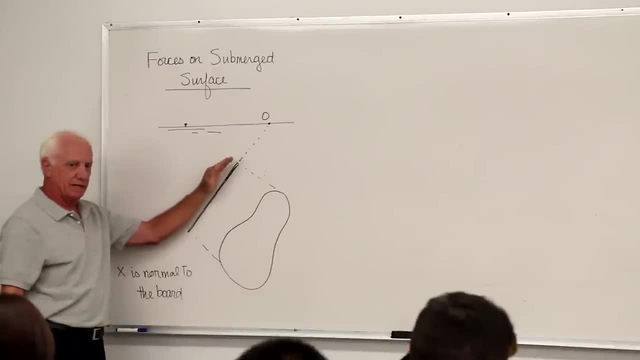 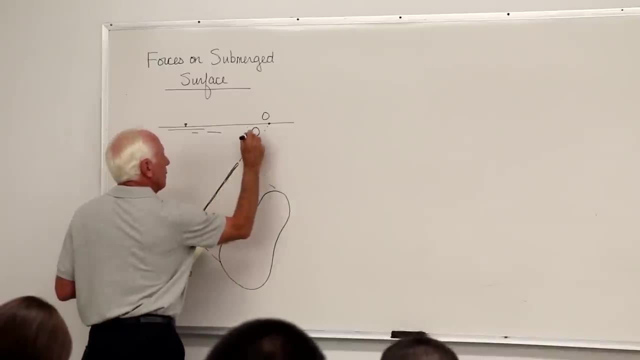 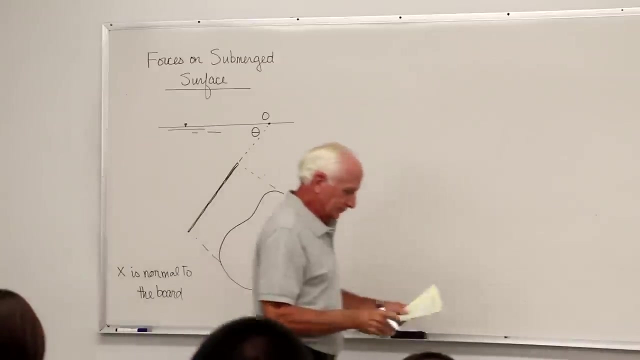 The y-axis we measure down along the plane of the surface. Here's the plane of the surface. We measure y down this way: the incline. We call this angle here theta. This is not an arbitrary surface, but here's a surface, right here. 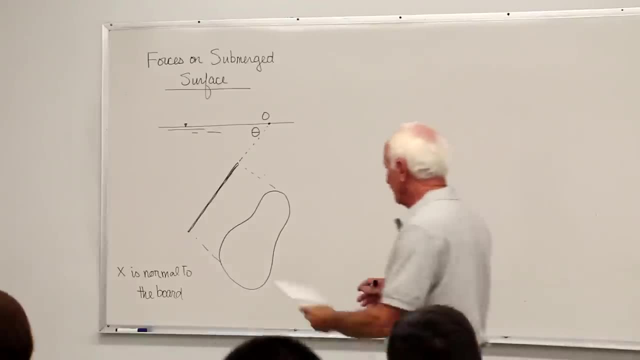 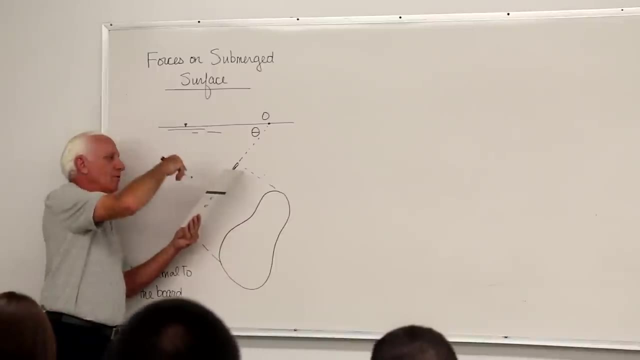 Okay, This is a cardboard. So here's the surface like that. Look at from above, Normal to the surface. What do I see? I see a rectangle. So this is the edge view. This is a head-on view. The one picture here shows both of these. 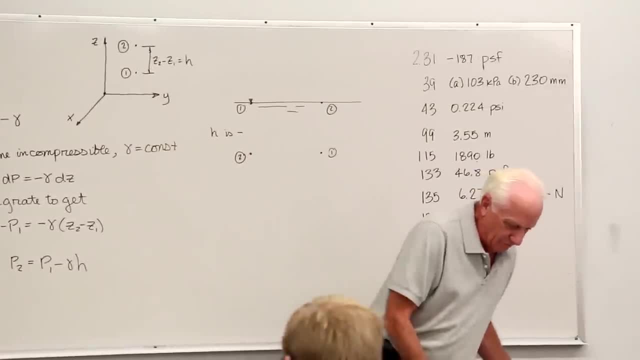 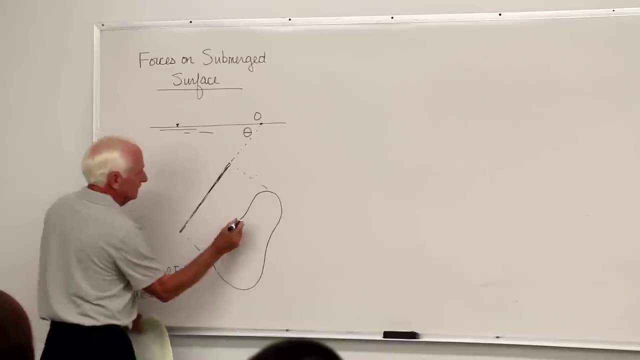 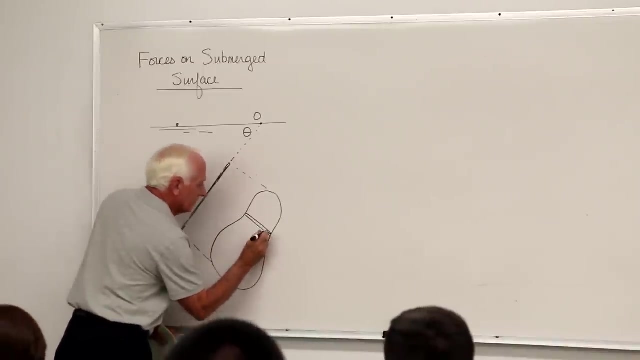 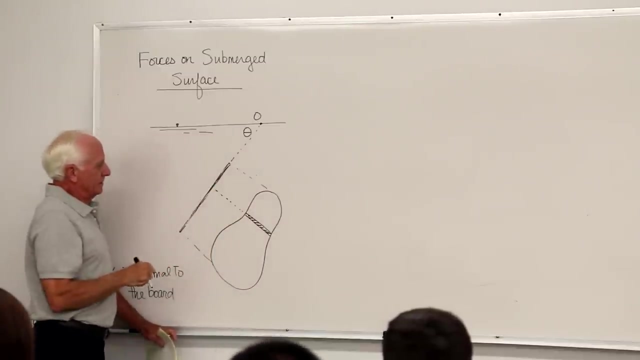 Okay. Now, if we draw A line like this across here, That line is right here Along here. At that point the pressure is everywhere the same between my two fingertips, Because it's at the same depth down from the free surface. 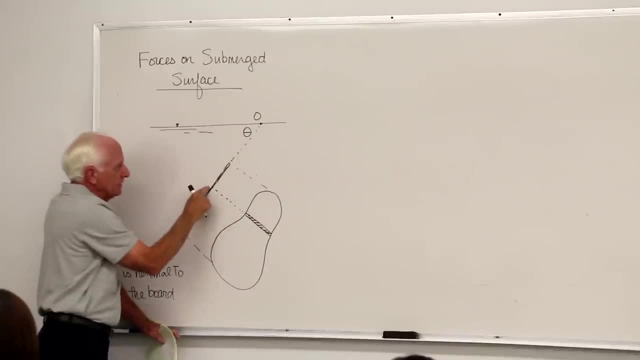 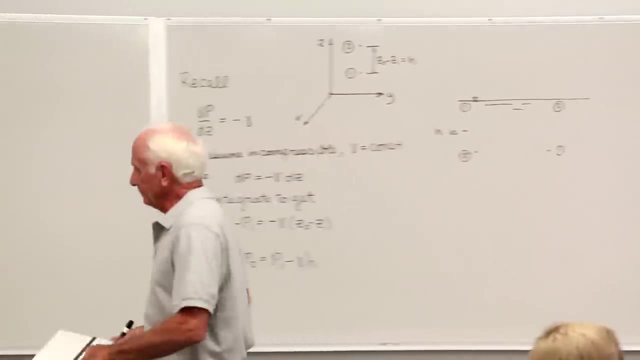 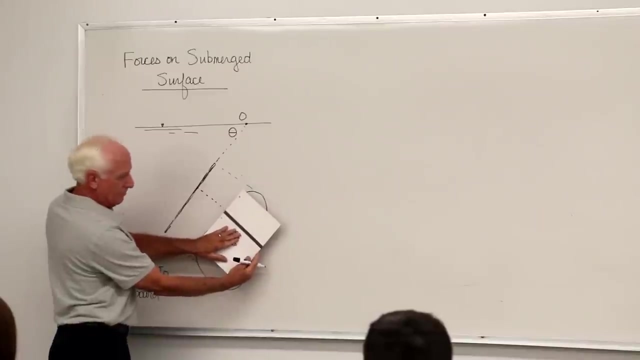 It comes down from the free surface to this point. I'll show you again on the paper. Okay, I turn it this way. There's that big dark line. When I turn it this way, how far is the dark line from the free surface? 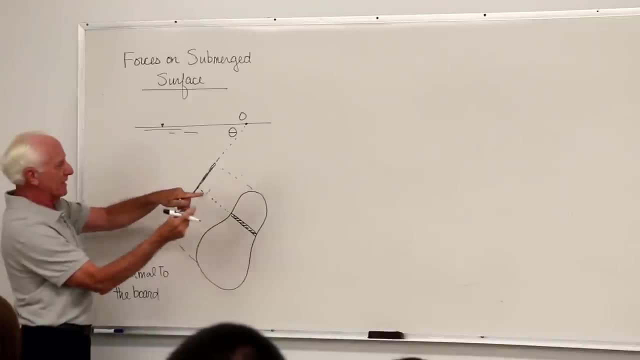 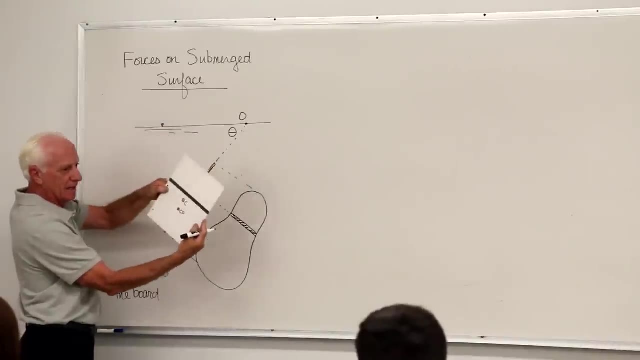 From here down to here, No matter where I go- left side, right side, left side, right side, left side, right side- it's still the same depth from the free surface to that black line. So I know along that black line the pressure is constant. 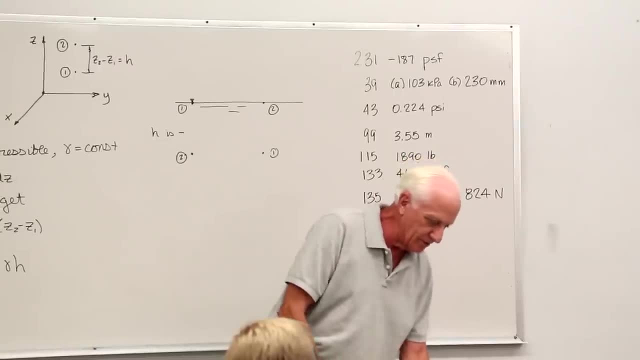 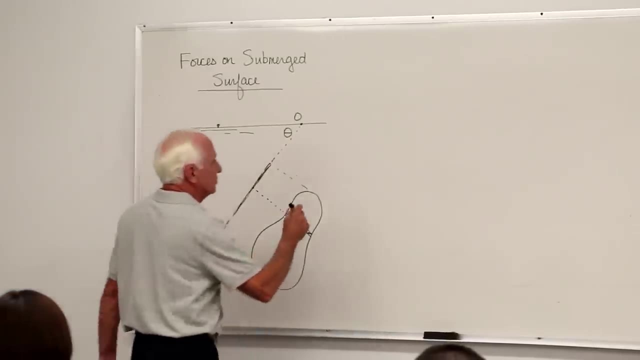 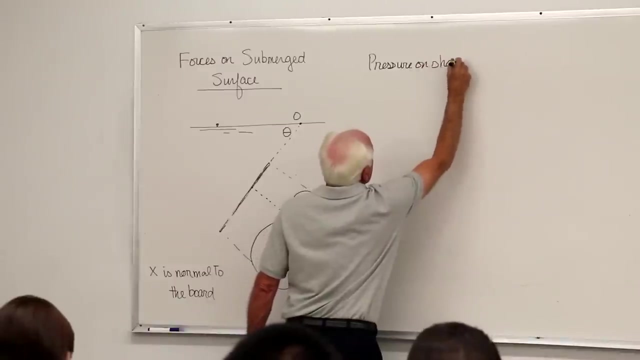 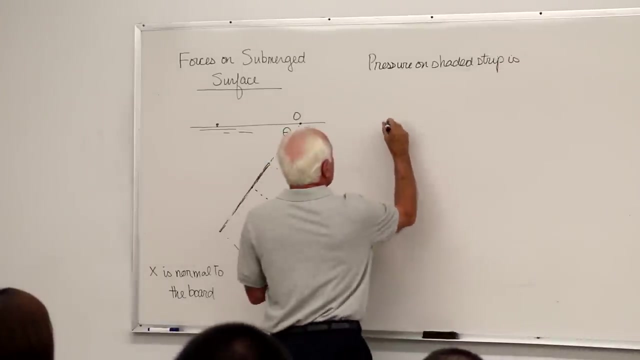 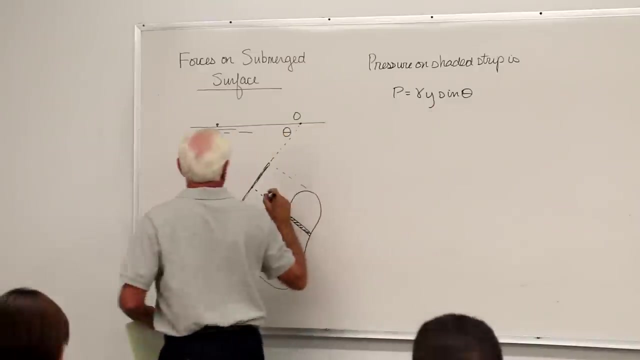 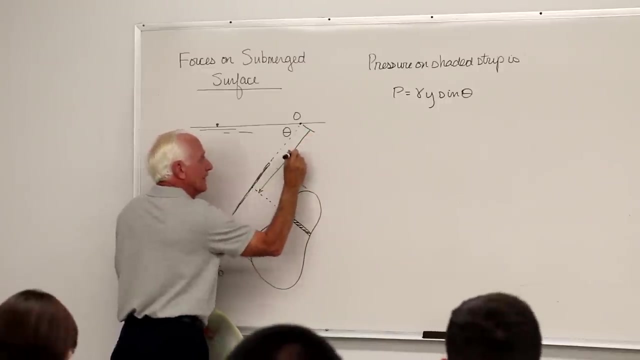 That's how you, That's the key, how you start out. The pressure is constant along that line. The pressure at the shaded strip is Now: here's the distance y: From here measured down to there, That's the distance y. 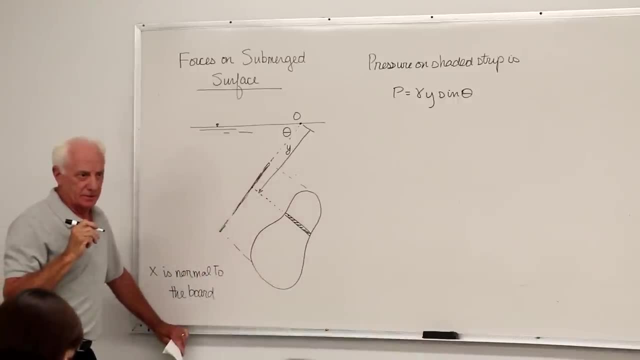 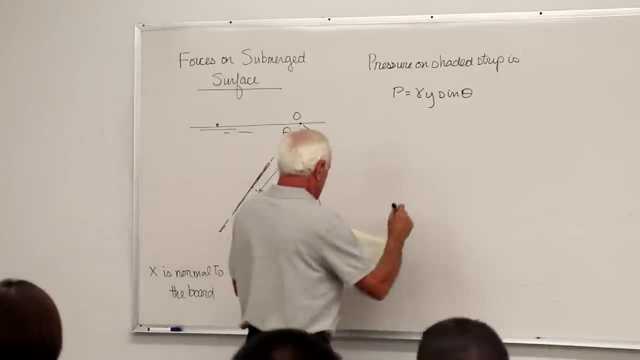 It's on the incline, It's not the vertical distance, It's the incline distance. So the pressure on that strip, again The differential force is pressure times area. So the differential force on that little strip, that very thin strip, 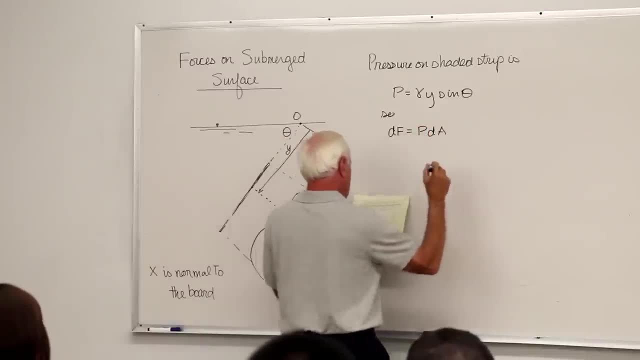 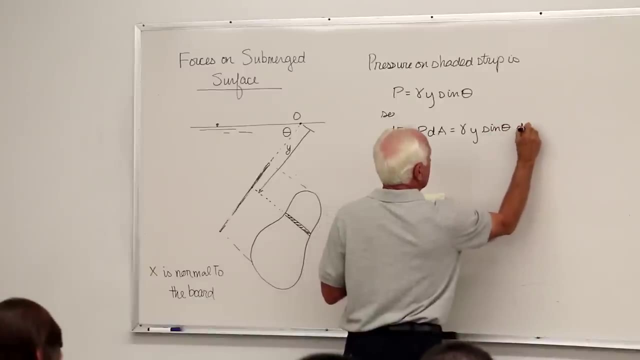 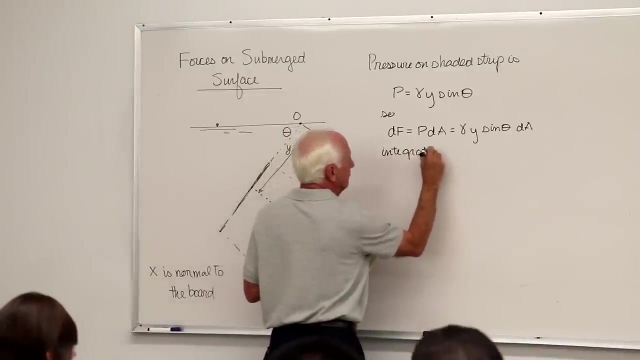 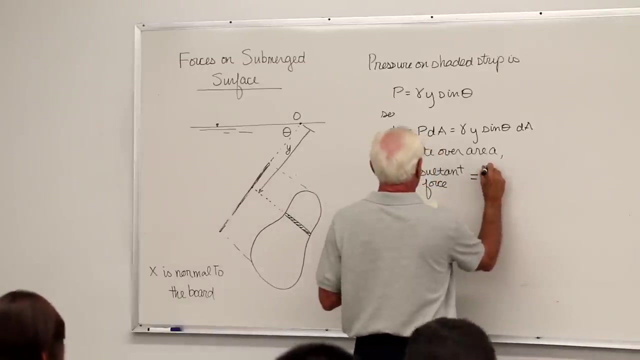 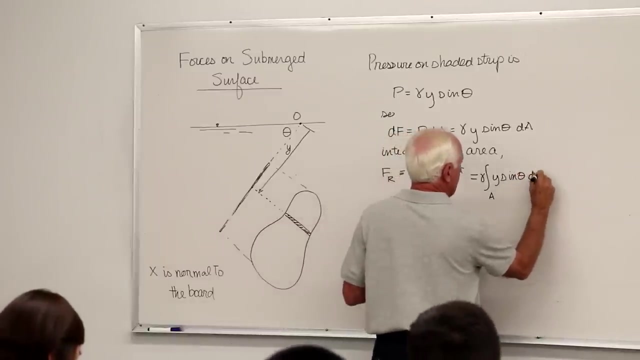 is PDA Gamma y sine theta b? a Integrate over the area. That gives us something called the resulting force. There's a gamma in there y sine theta. dA Gamma comes outside. it's constant Sine theta. 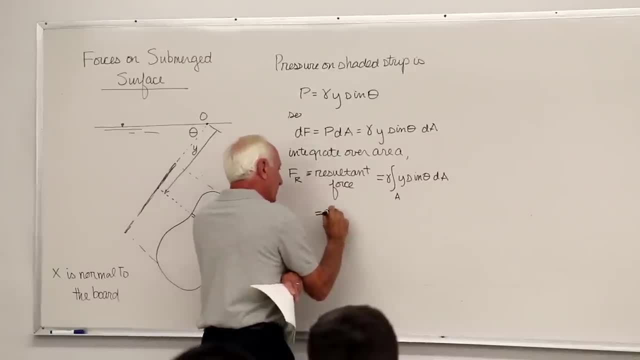 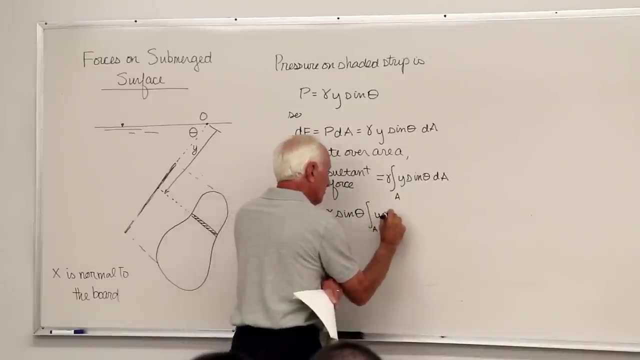 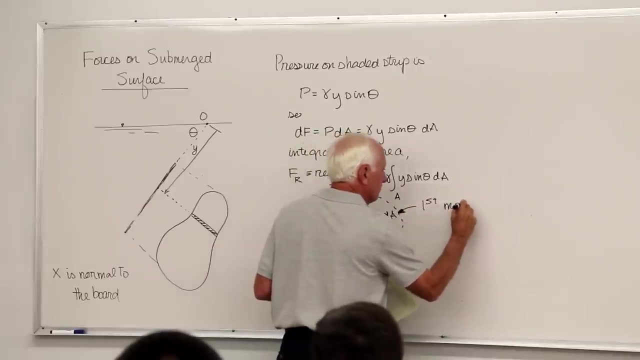 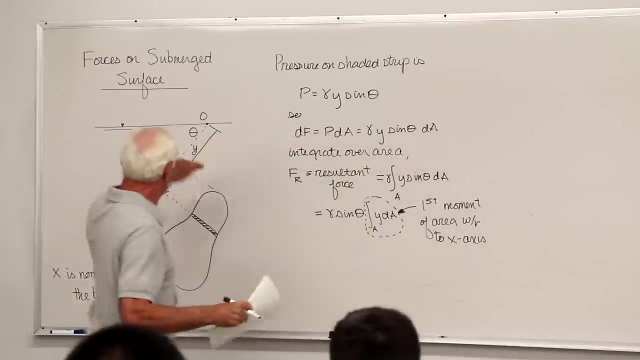 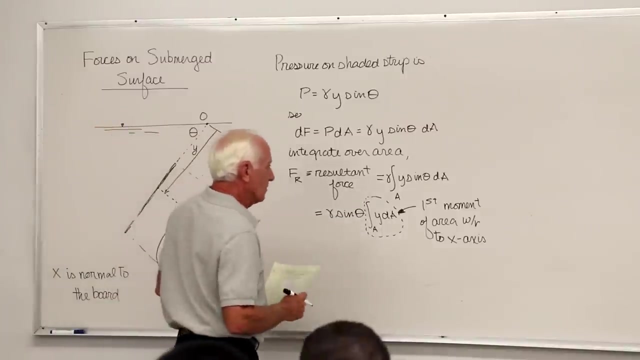 comes outside. it's a constant. That guy is the first moment of an area With respect to the x-axis, the axis that goes into the blackboard. So y dA first moment of the area with respect to the x-axis, And then recall that the location of the centroid 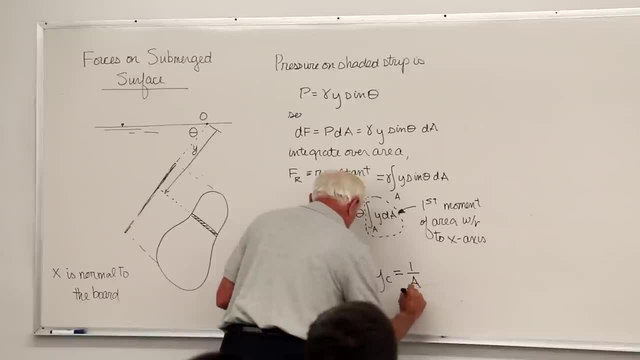 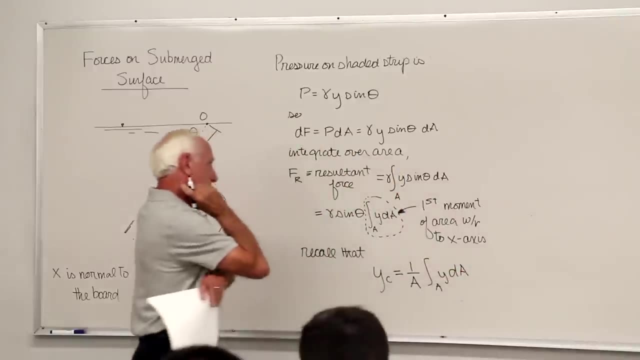 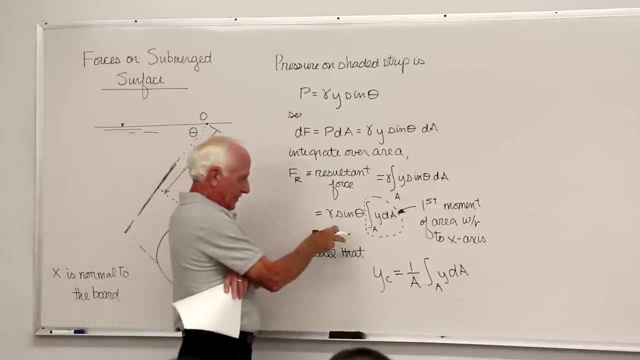 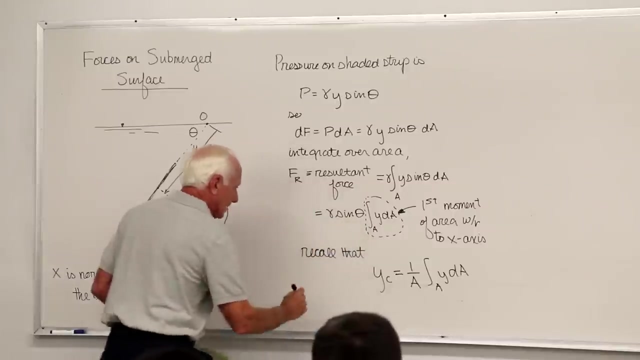 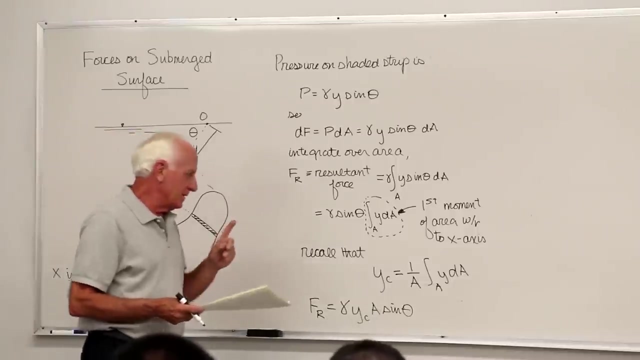 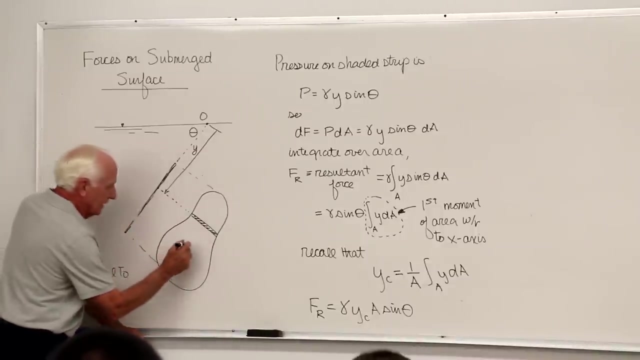 of an area in the y direction. is that? So if I multiply and divide the right side equation by the area, what I'm going to get then is F sub r, Gamma y sub c, A sine theta. But then now, what is y sub c? y sub c is the location of the centroid. so if this is, 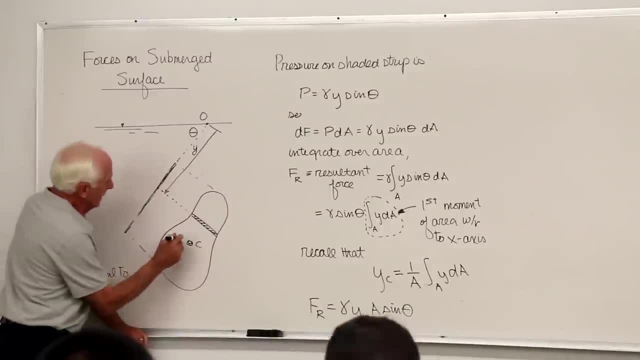 the centroid. call it c, then y sub c is this distance down. So this distance is the situation of the centroid. call it c, and then y sub c is this distance down? Gamma y sub c, A sine theta. but then, all right now, what is y sub c? Y sub c is the 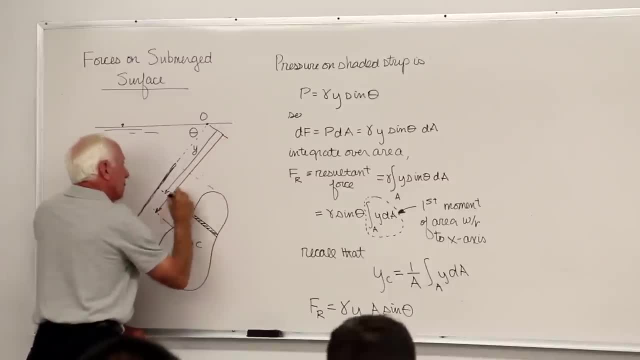 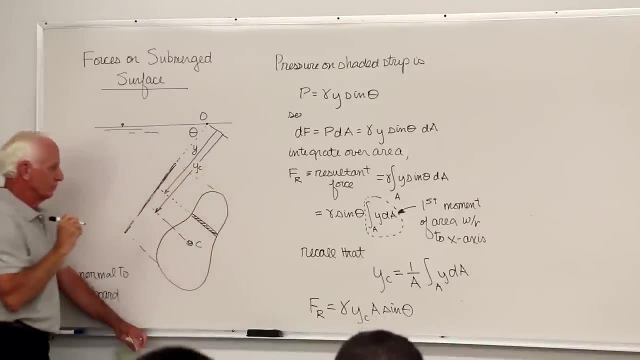 down here. Here's y sub c. Okay, so y sub c, sine theta. Here's the right triangle. Down to here, up to here right triangle, The sine is the distance from here up to here. We call that h sub c. 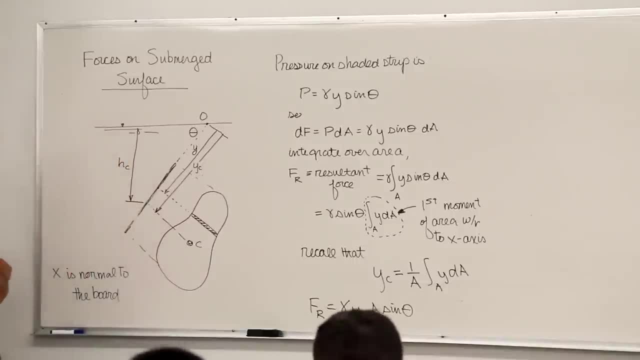 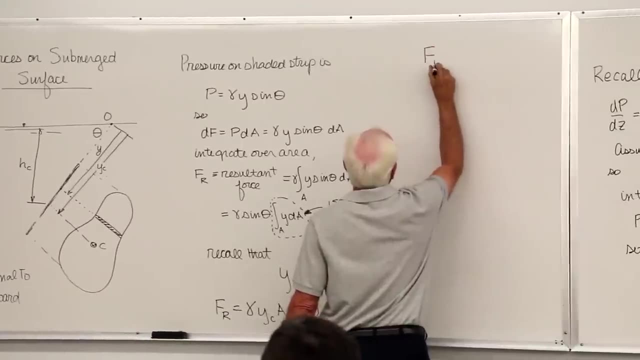 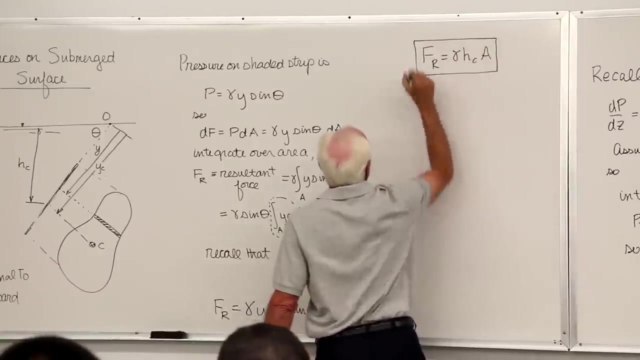 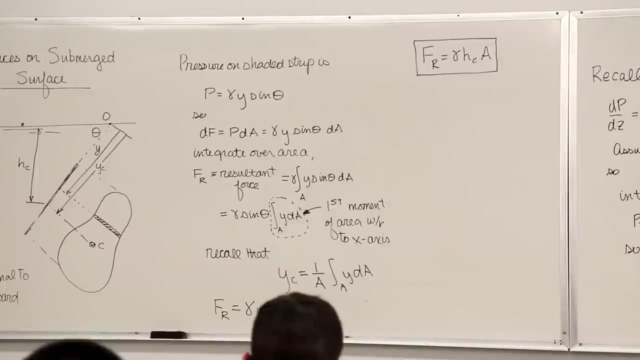 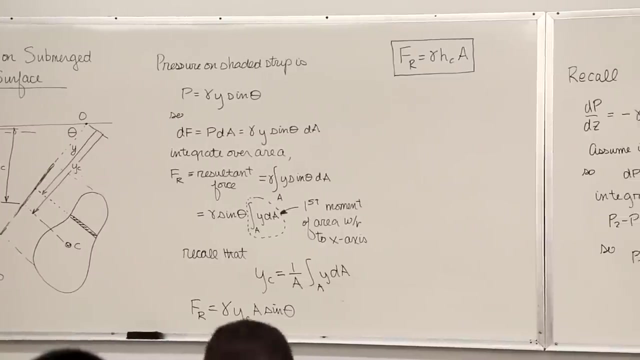 h being the vertical distance. So f sub r is then gamma h sub c, a. A very simple, straightforward equation: Gamma specific weight of the fluid, h sub c, the vertical distance down from the free surface to the centroid of the inclined plane surface. 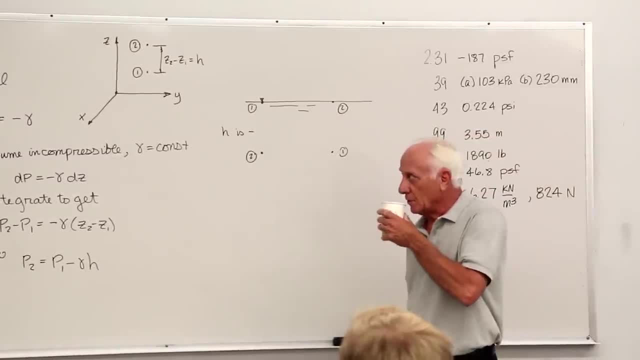 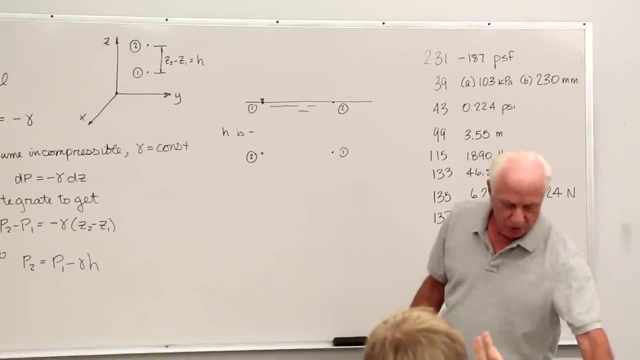 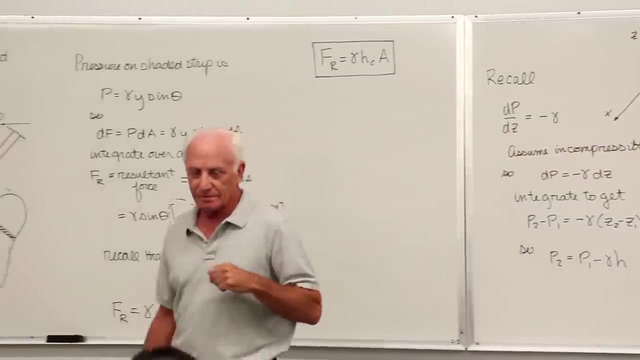 A, the area of the inclined plane surface. Check the units: Gamma newtons per cubic meter. Multiply it by a meter. Multiply it by a meter squared, You get newtons. Okay, so right in this Force in newtons. 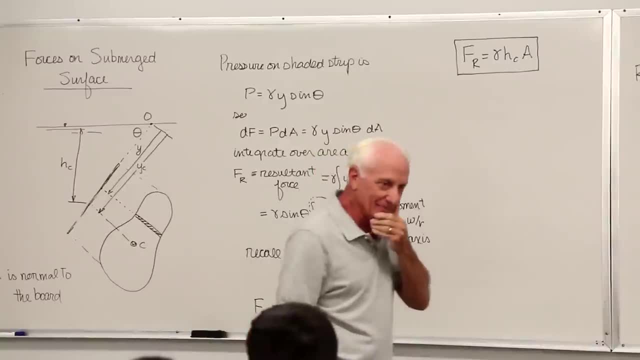 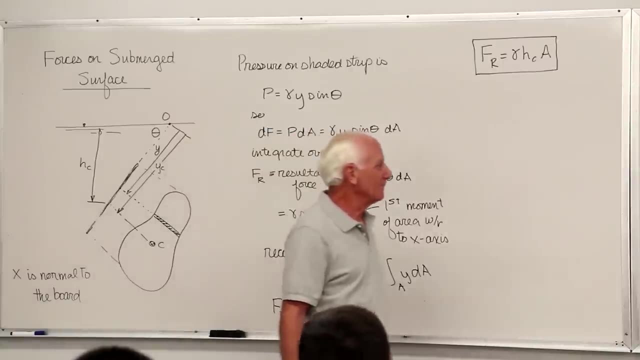 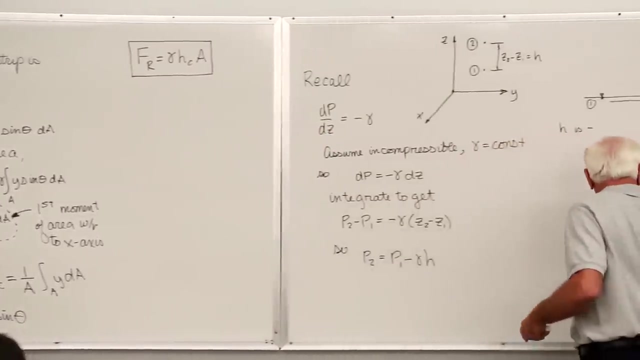 Question, That's the force over the entire area. You got it Because, here it is, we integrate it over the entire area. Okay, so that's the first thing. How do we find the resultant force on a submerged plane surface? 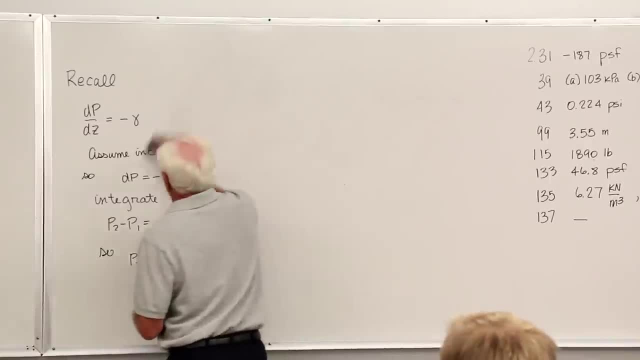 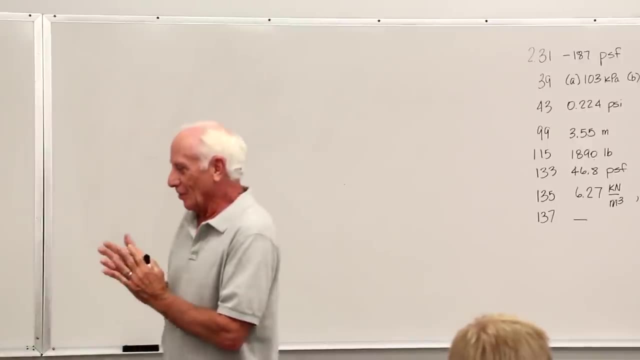 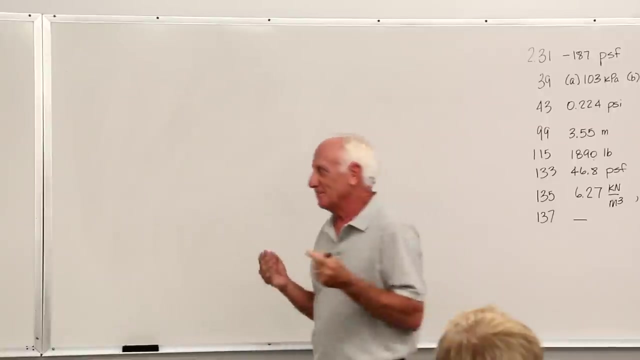 Now, of course, it's like in statics: You got some loading diagram. You want to know what's the equivalent of force number one. Number two is: where does it act? That's important. And now, where does this force act? 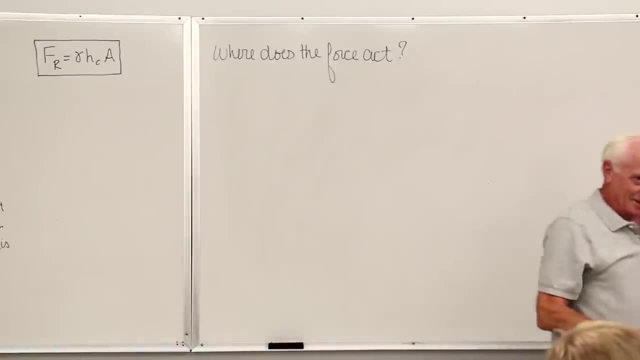 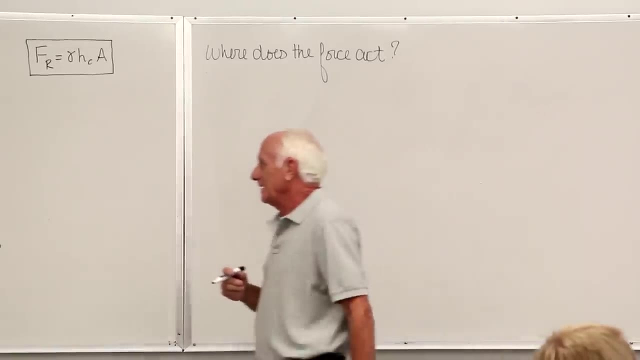 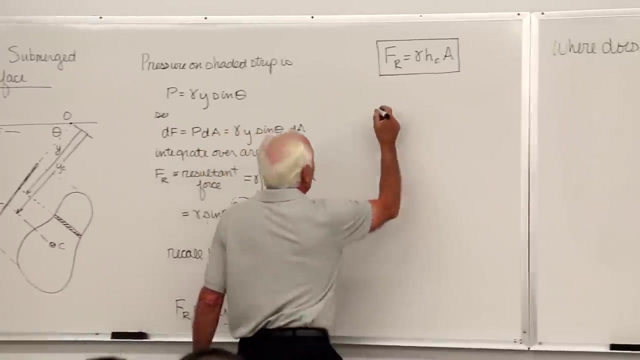 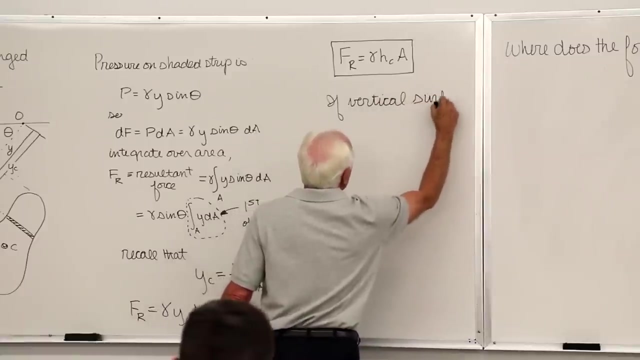 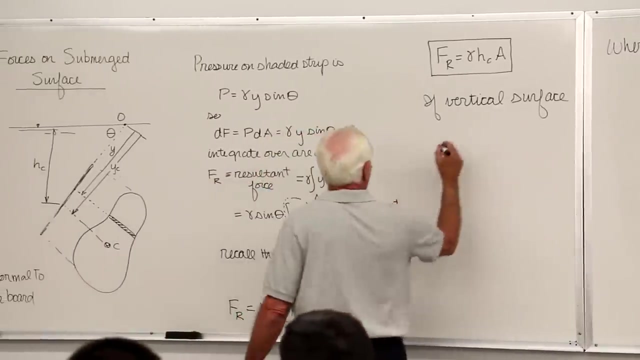 Okay, it's a tougher one now. That was the easy part. Let's just do two simple things here. first of all, I'll add to this: If vertical surface- Look at the picture- If it's vertical, y is equal to h. 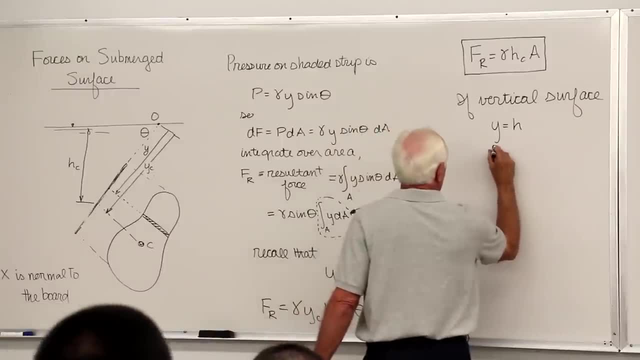 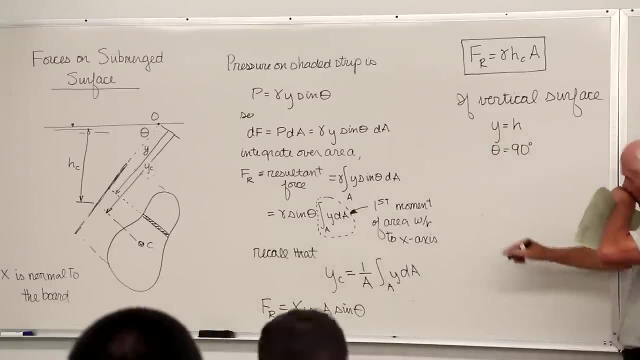 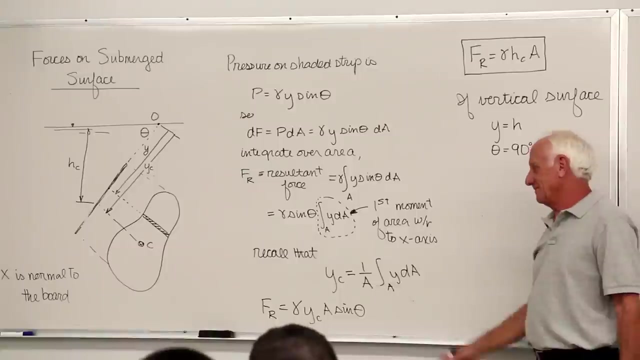 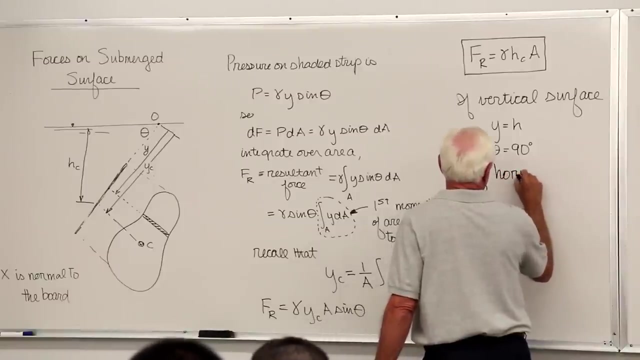 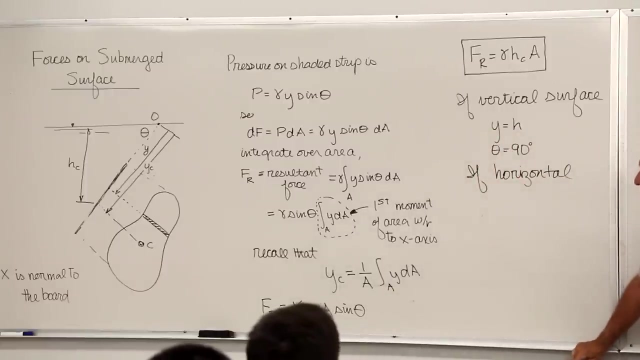 The angle of theta is 90 degrees. Sine of 90 is 1.. So vertical surface, h and y the same thing. If horizontal- Gotta be careful here- Theta is 0 degrees. Horizontal, Here's theta: 0 degrees. 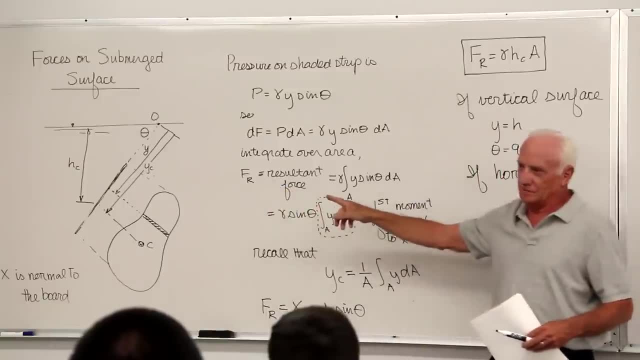 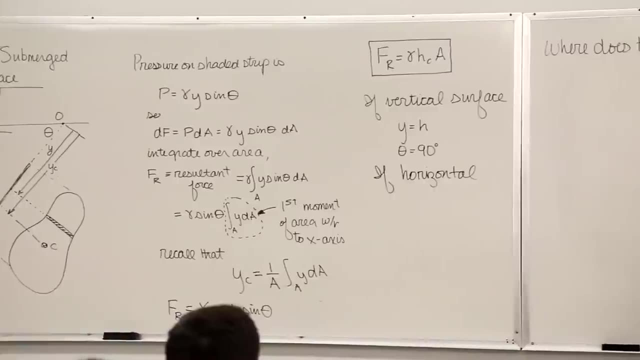 Put a 0 in there, The resultant force on the bottom of the swimming pool is sine of 0. 0? I don't think so. No, you can't do that. You can't do it that way. Okay, You take this guy up here. 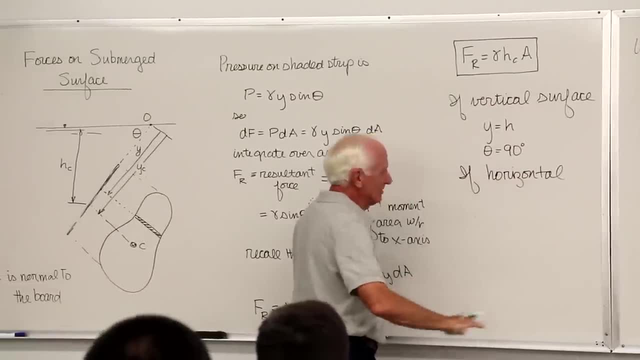 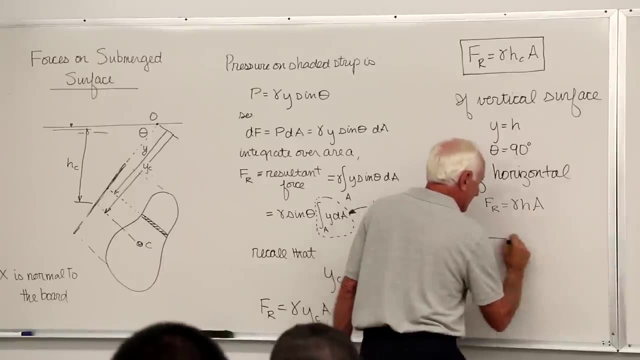 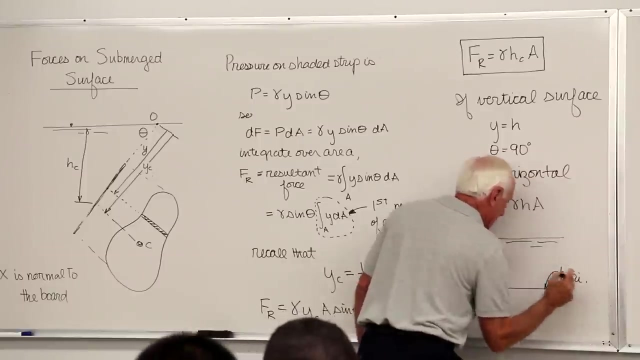 And h then is the distance down to the horizontal surface. So f, sub r, gamma, h a, Where here's the free surface, Here's the horizontal surface, And this is h Because the pressure's constant along the whole bottom of that. 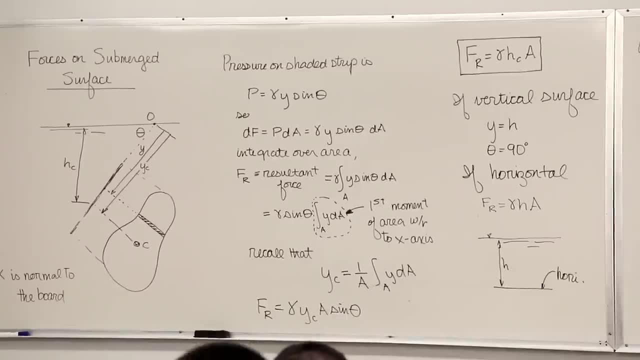 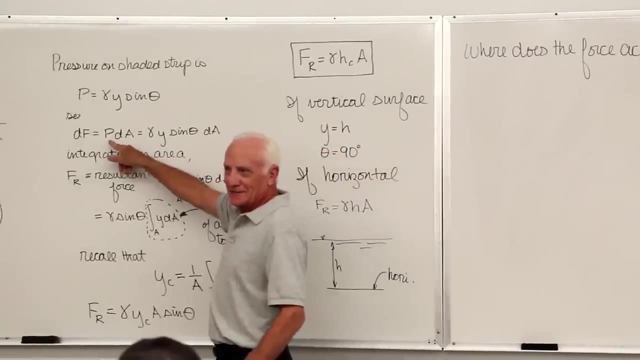 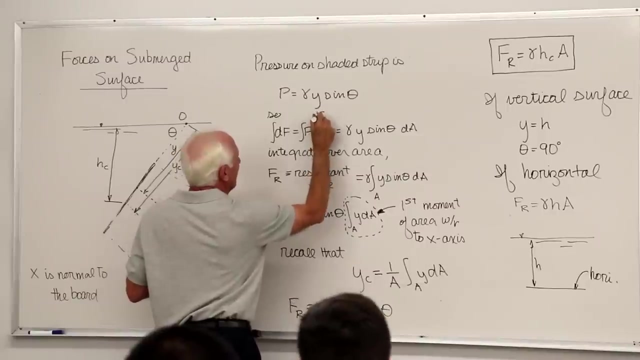 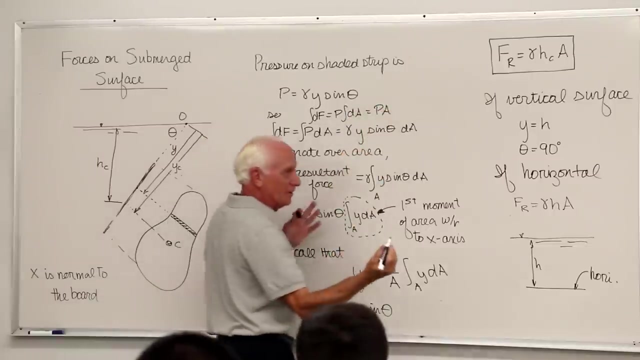 Of that surface. The pressure's constant. So all you do is you pull the p outside the integral sign here. Integrate both sides of this guy right here. Pull the p outside What's this? equal to p times a. So if you want to, what can you do in here? 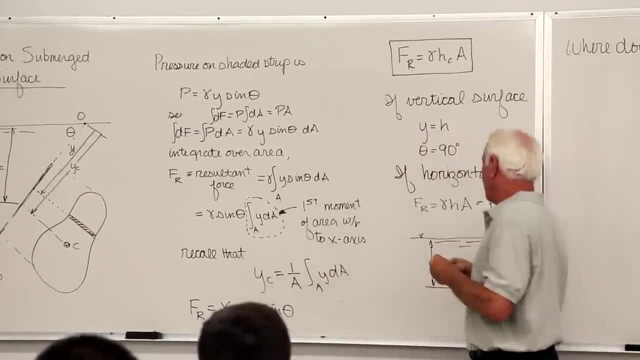 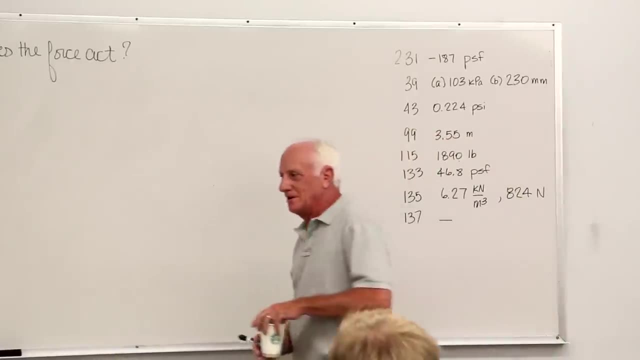 You just say p times a, The pressure at the bottom times a. The pressure is gamma times h. So that's how you tackle a horizontal surface. So now you've got what you do for a vertical surface, A horizontal surface. 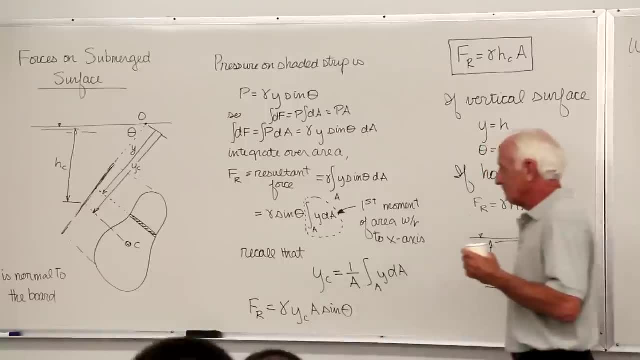 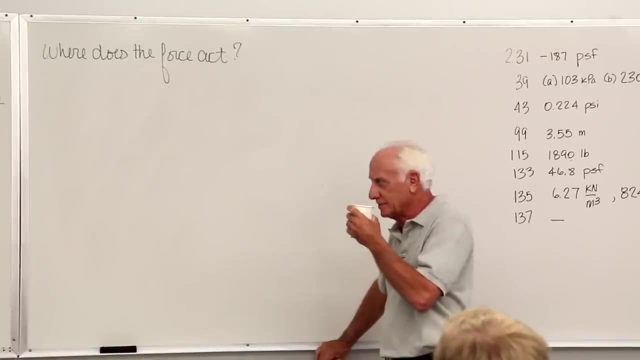 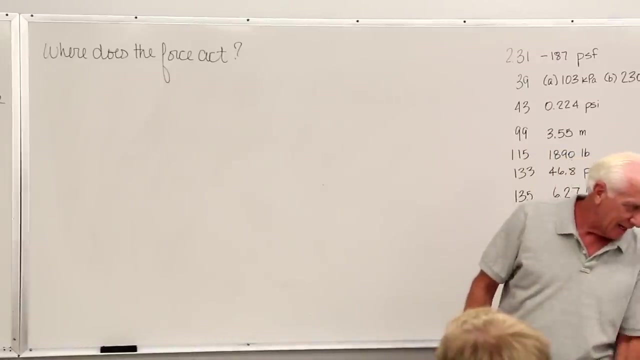 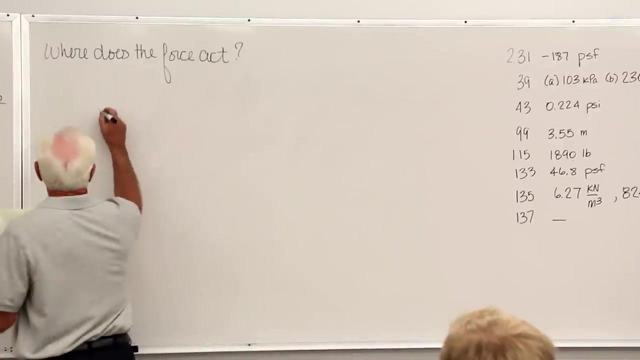 And an inclined surface. Okay, Restriction, Incompressible, And it's a plane surface. It's not a curved surface, It's a plane surface. Okay, back to the other question now. Where does it act? Okay, This is from statics. 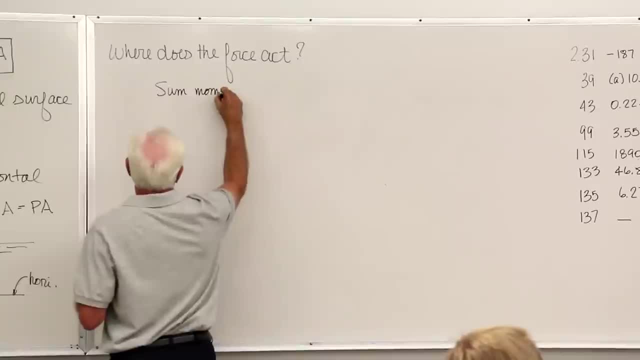 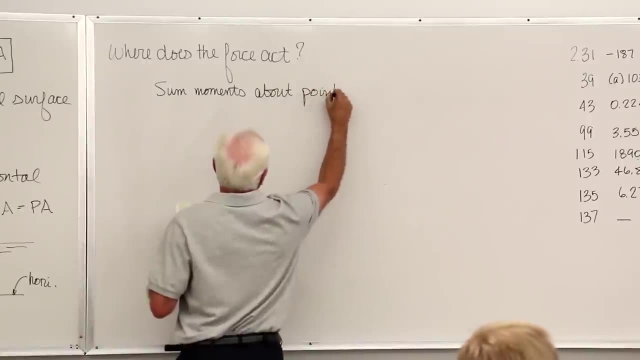 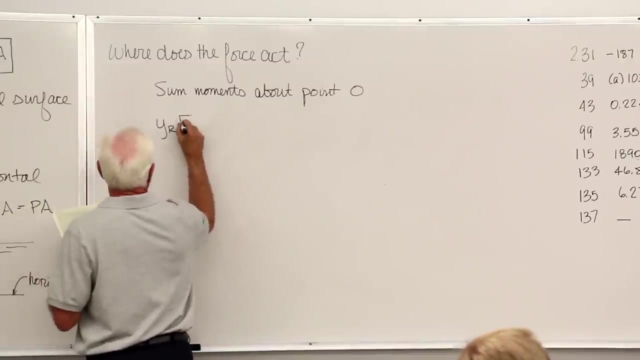 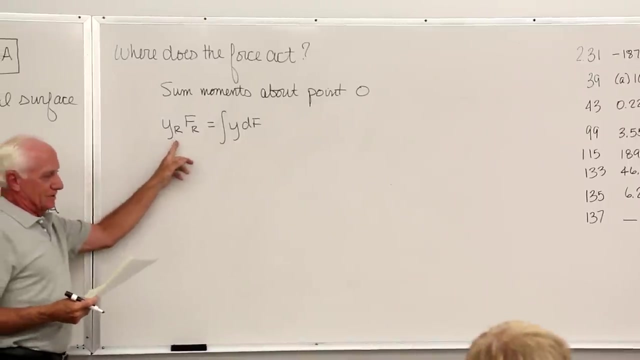 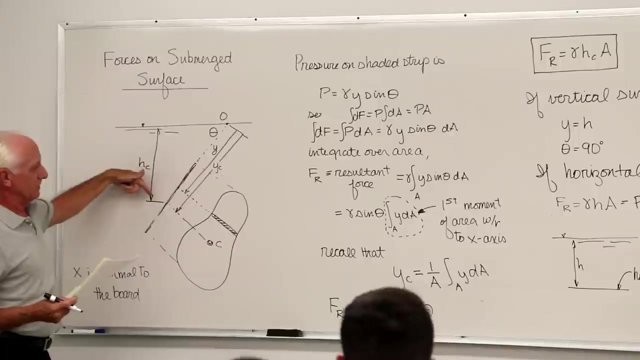 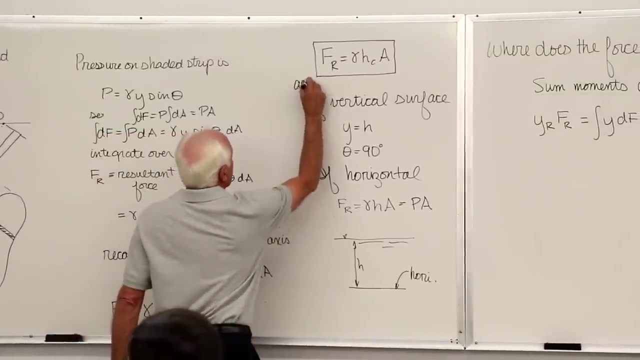 Some moments about point O. I'll describe this in a minute. Y sub r and F sub r. We know what F sub r is. Y sub r is the distance from point O down to where the resultant force acts And, by the way the resultant force acts, normal to surface. 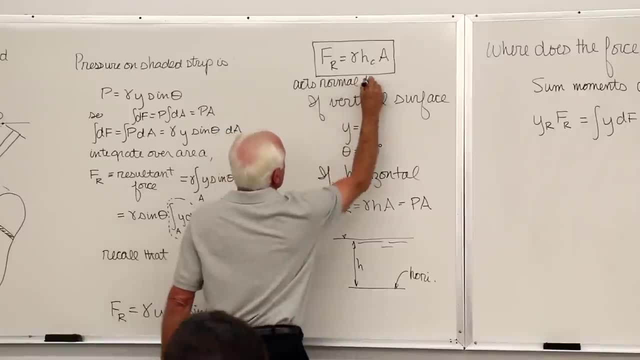 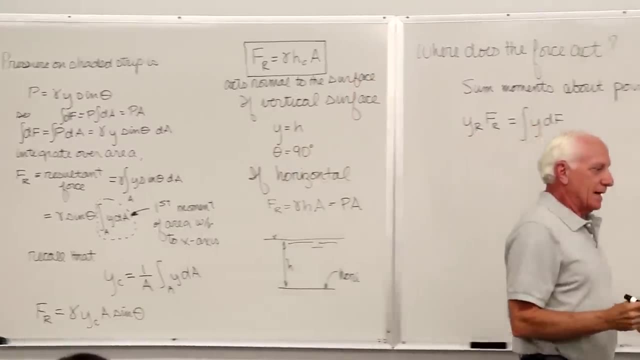 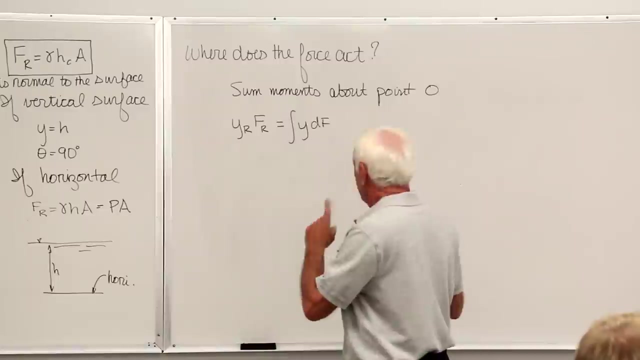 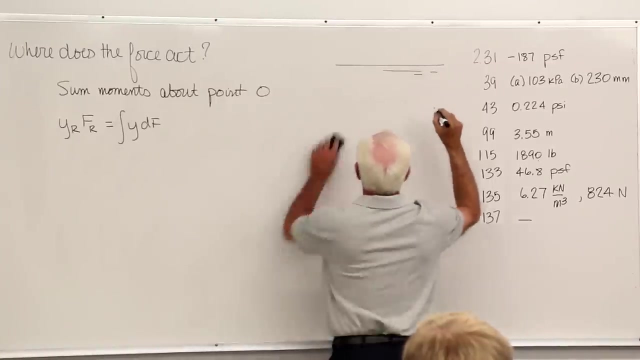 Okay. So what does it do? It acts normal to the surface. Why does it act normal to the surface? Well, let's go back. I'll draw one more picture. I'm going to put it just temporarily right here. Okay, 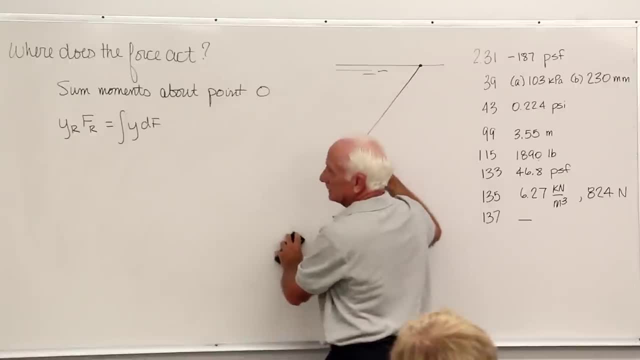 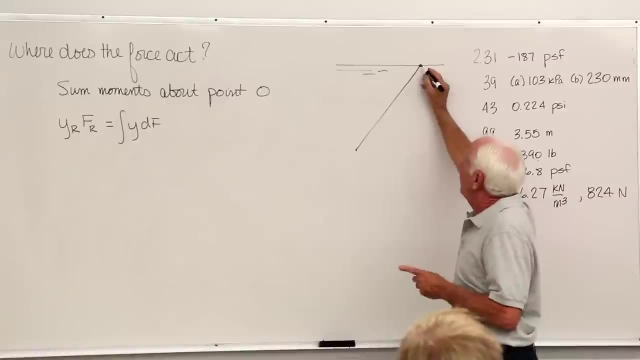 Here's the surface. Okay, This is the surface At this point, where my black marking pen is, the pressure is zero gauge, Zero gauge. The pressure increases linearly as we go down along the surface, Increases linearly, Why? Well, I just showed you that the delta P equals gamma delta Z. 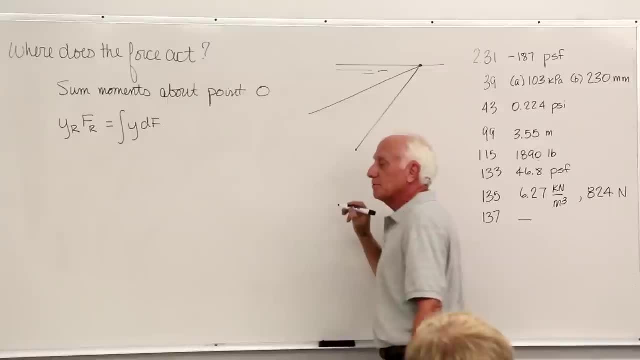 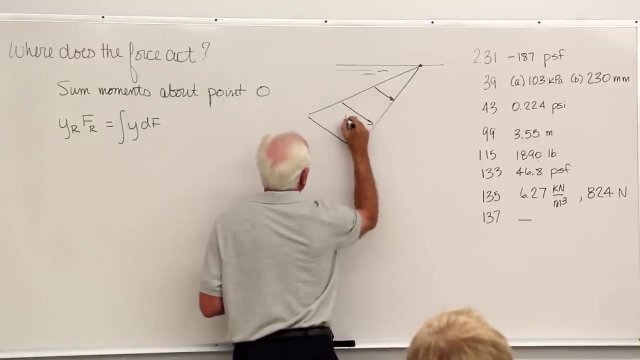 Linear, Linear. If I go down, the pressure increases linearly. How does pressure act on the surface? Well, here's the rule: Pressure is a normal stress, Therefore the pressure force acts normal. Okay, So all these pressure arrows act like this. 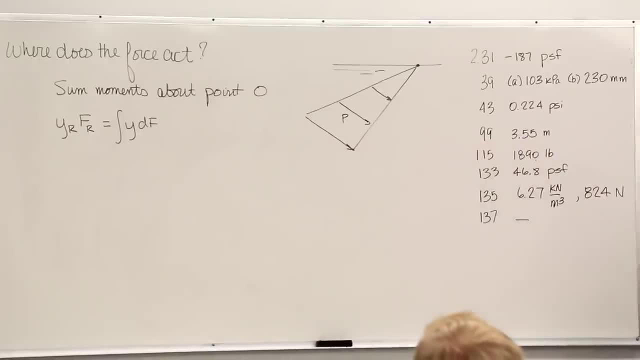 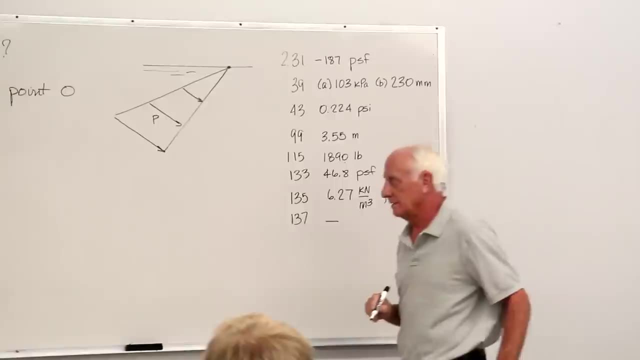 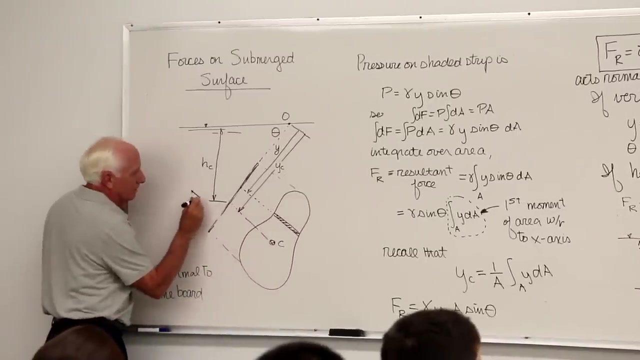 That's the pressure. So which way would you think the resultant force would act? Well, it's pretty clear from that that the resultant force acts normal to the surface. Okay, so the resultant force acts normal to the surface. there it is, over there I. 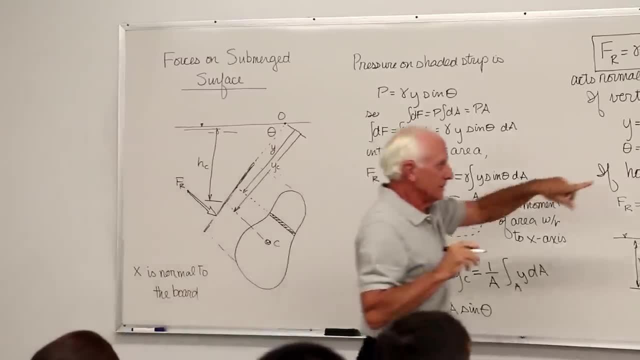 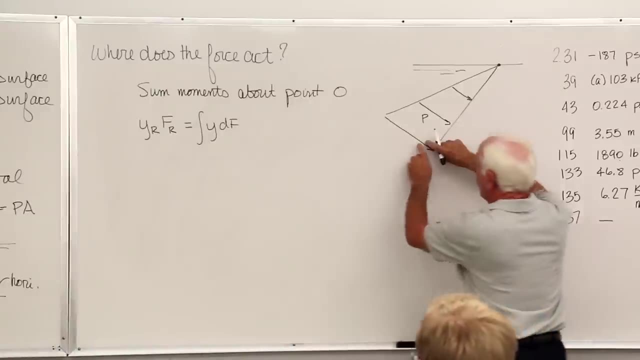 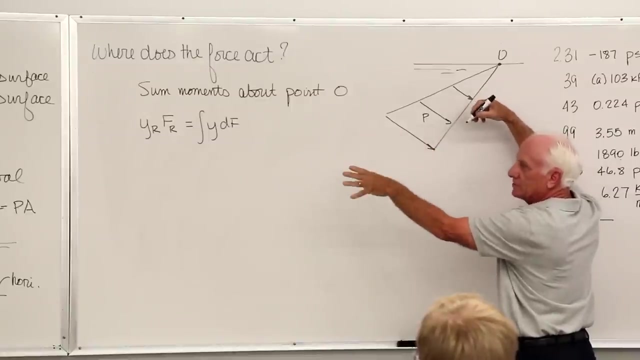 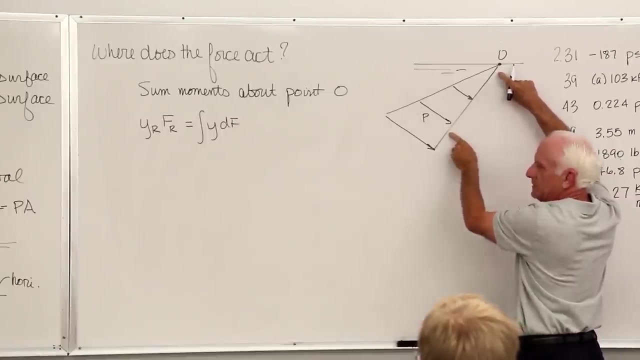 don't know where you find out right here. so static says: if I add a moment of all these little individual forces about 0.0, then that should be equivalent to the resultant force multiplied by the distance to where it acts. the resultant force might act from that fingertip is. take the moment about that. the moment is. 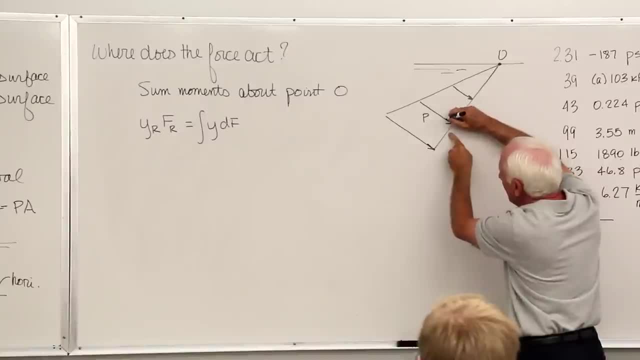 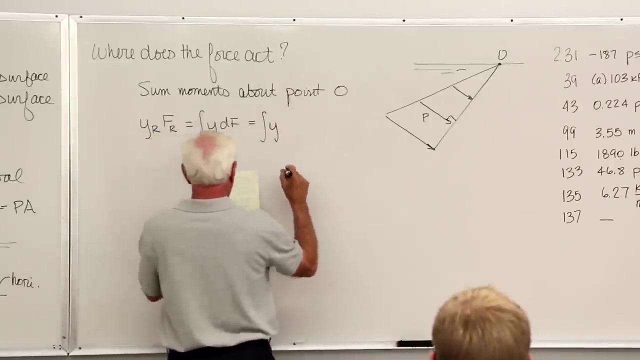 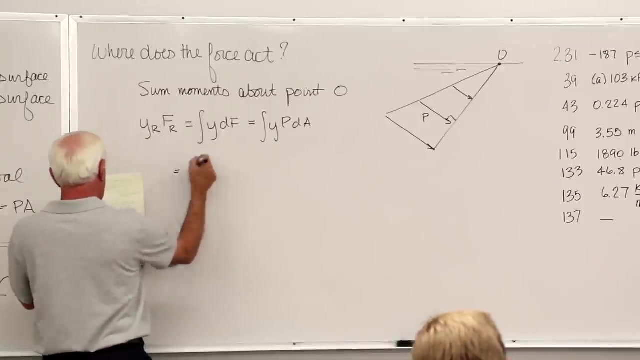 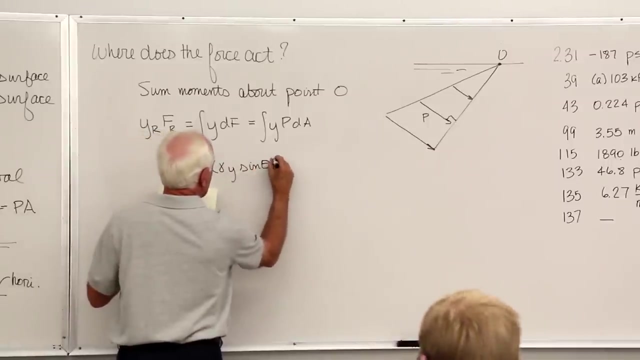 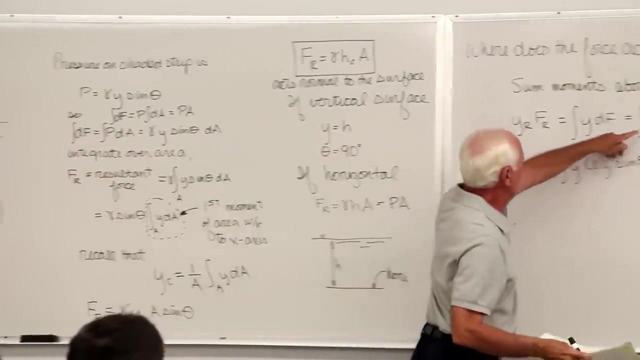 the wide distance times. of course these guys are all normal. that's the definition of a moment. okay, now let's replace the force with pressure. so integral Y and pressure, it forces. PDA carry out one step more of the. replace the pressure in there. integral Y, the pressure, it's up here. okay, our pressure, gamma Y, gamma times H and H is: 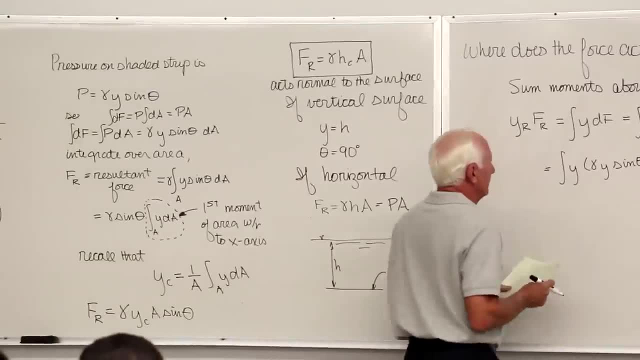 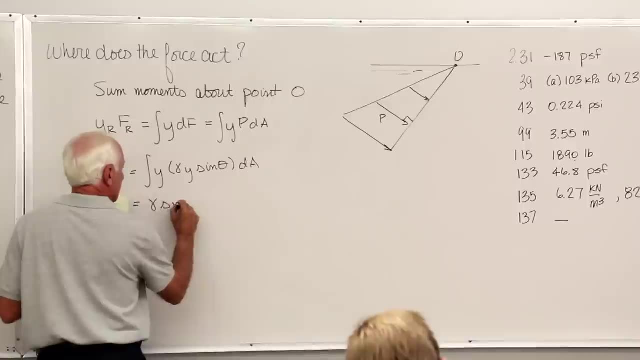 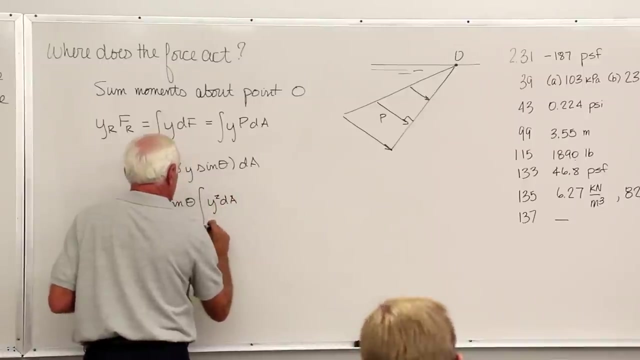 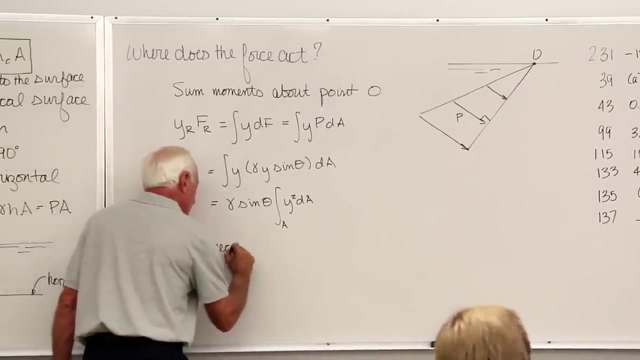 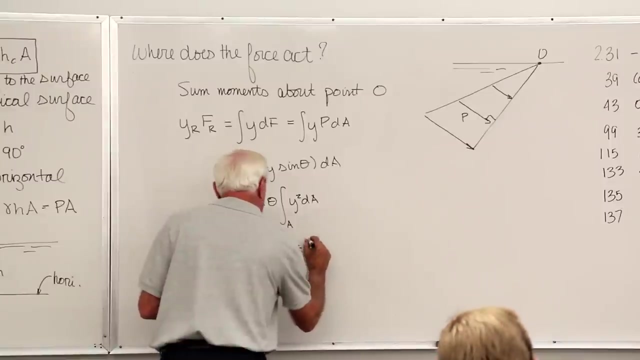 Y sine theta. okay, keep going equal. to bring out gamma constant. to bring out sine theta constant integral y times Y. Y squared VA over the area. recall an inertia about X axis, defined as Instantcy, at anhigh angle at least, road y square da. so that's the second moment of inertia, this guy is the first. 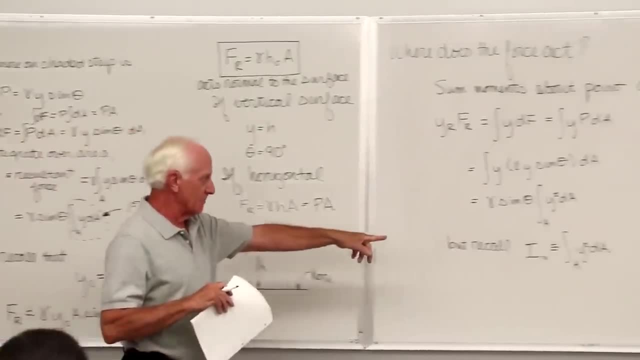 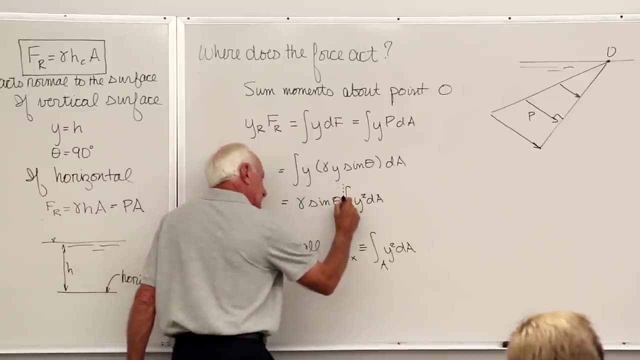 moment of inertia: y da. this guy's the second moment. y square da. okay, there he is right here. I see that guy in there, okay, so I'm going to put him in there. but also we recall that the moment of inertia about any x-axis moment of 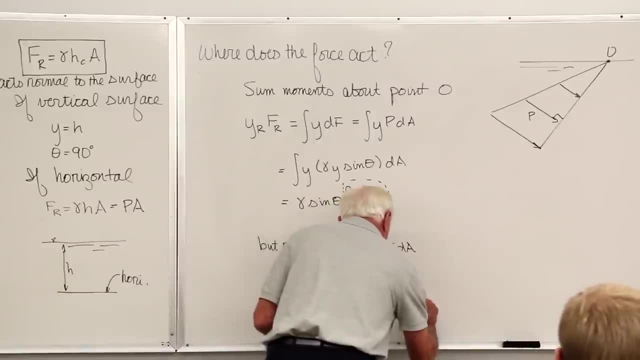 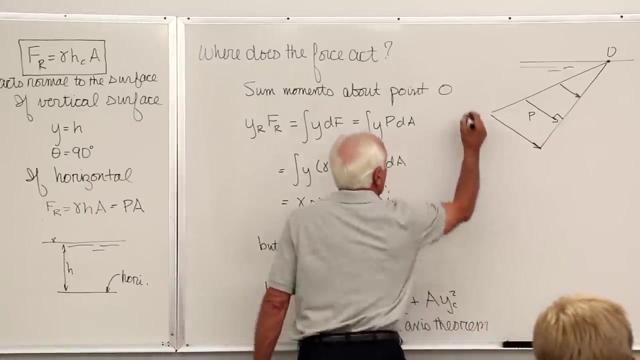 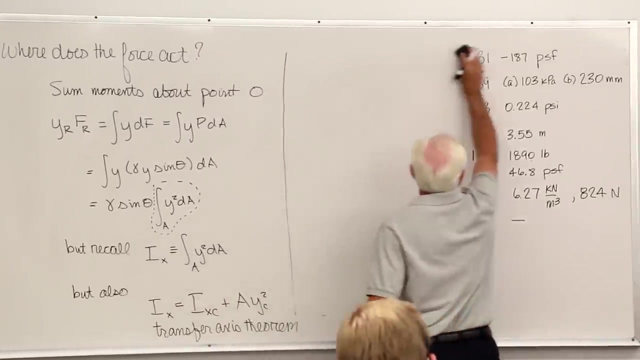 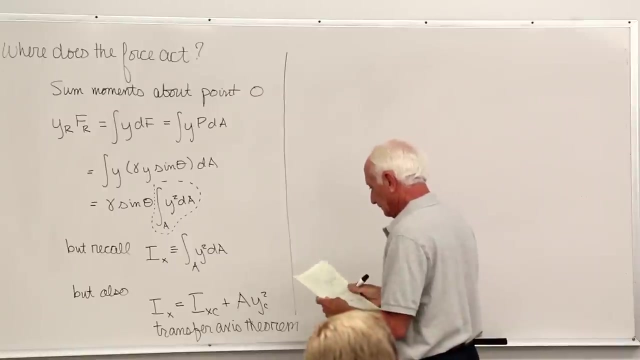 inertia about the x-axis of the centroid plus a, y sub C squared transfer axis theorem. okay, now all that stuff in there. so y sub R, F sub R equal gamma sine beta quantity. I XC plus y squared where C times the area comes from down here. 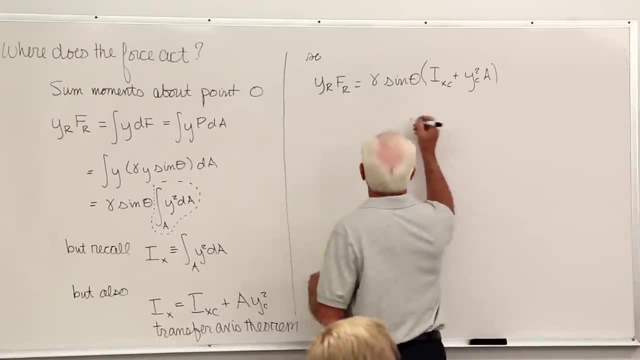 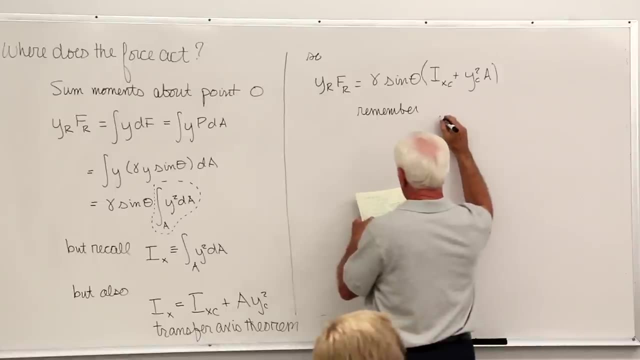 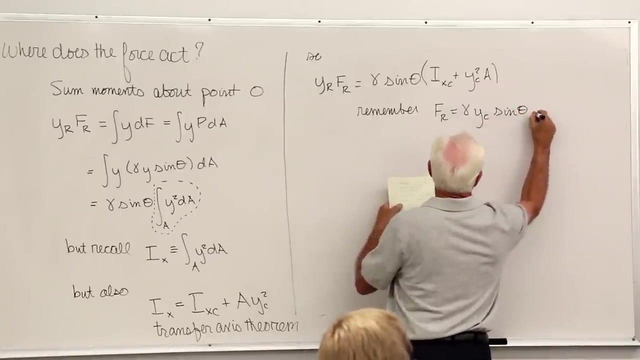 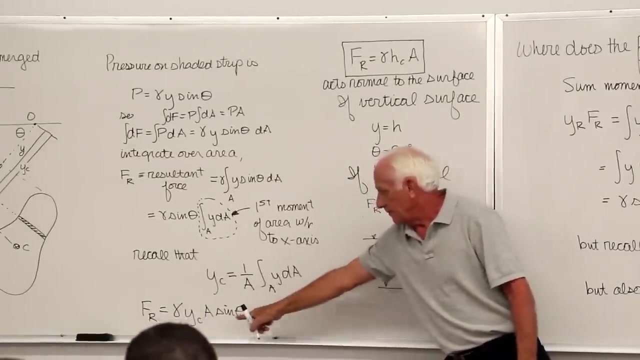 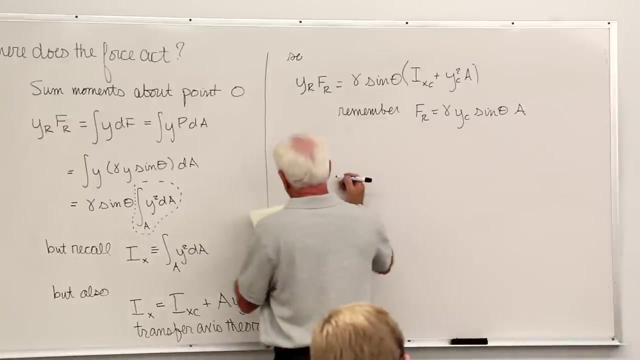 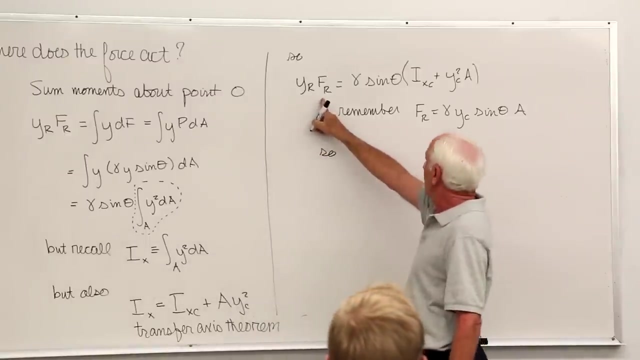 And let's see. I think then we're going to recall that F sub R That's over there. So our Y sub R now remember you see F sub R, See F sub R here. Put that guy in Gamma, gamma cancels. 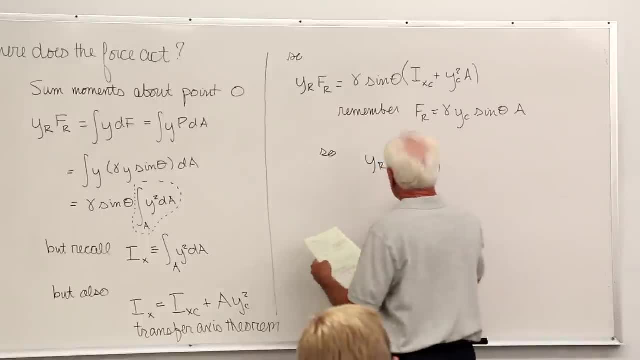 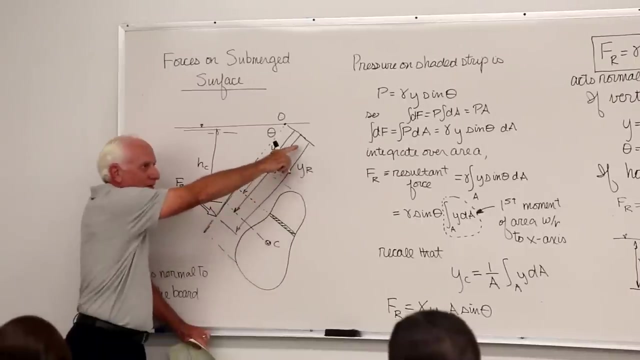 Sine theta. sine theta cancels Keep going. So Y sub R equals Y sub C, plus I sub XC divided by YC times A. Okay, so here's Y sub R. Y sub R is the distance down from point O. 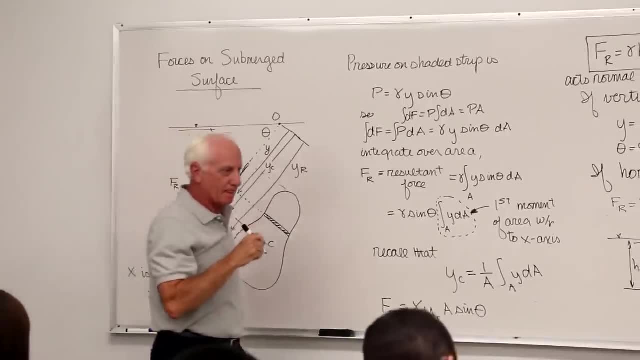 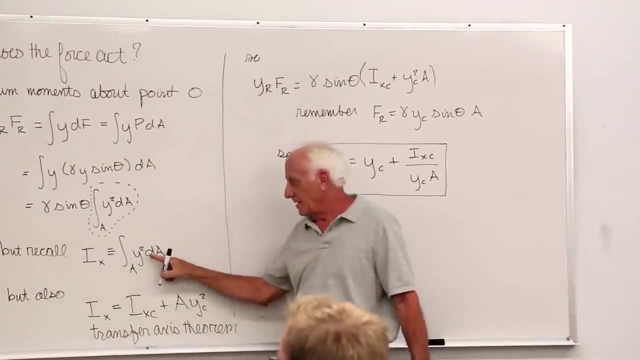 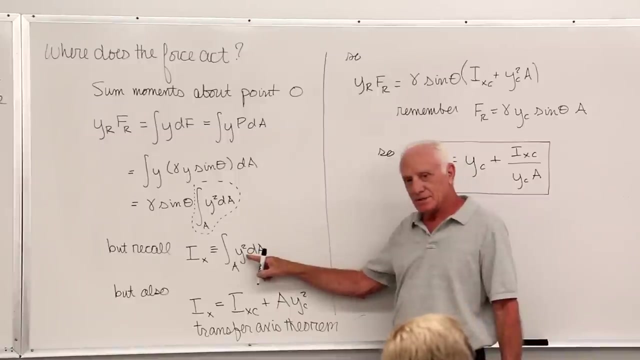 to where the resultant force acts. I sub XC. Look at it right here. Second moment: here is always positive. Why? Because it's a square. Y square, always positive, Area is always positive. Therefore, I sub: X is always positive. 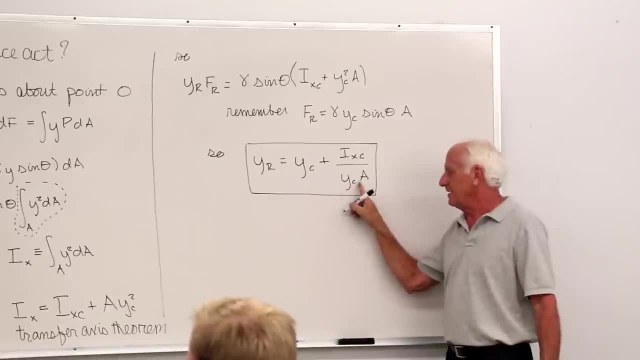 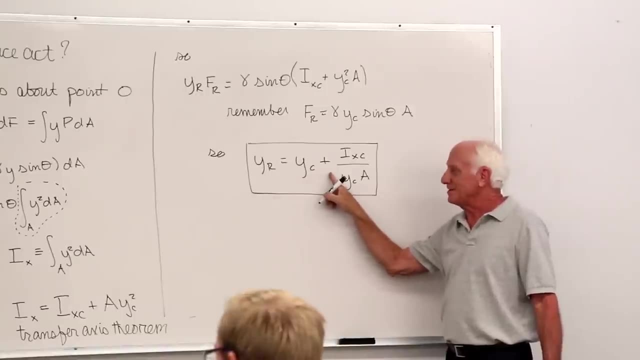 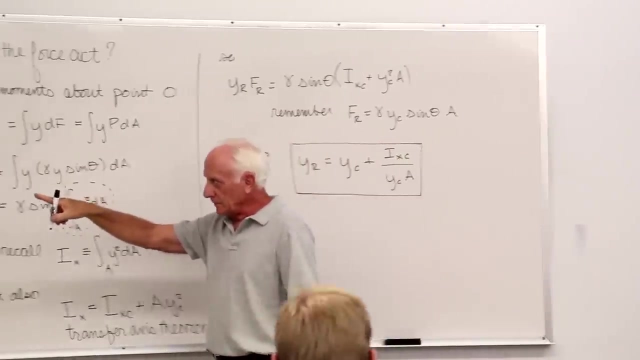 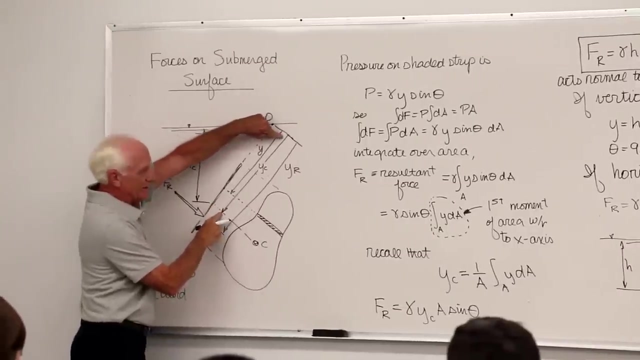 Y sub C is always positive. The area is always positive. Conclusion: Y sub R is Y sub C, always plus a little bit more, Always plus a little bit more, Which means, if this is where Y sub C is, to the centroid of the area. 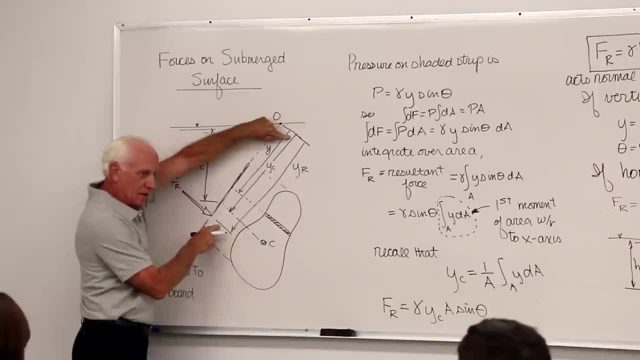 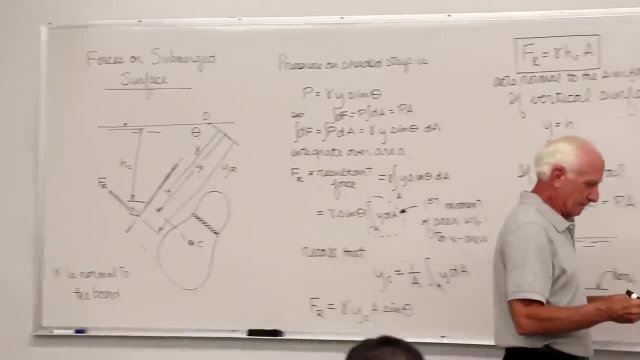 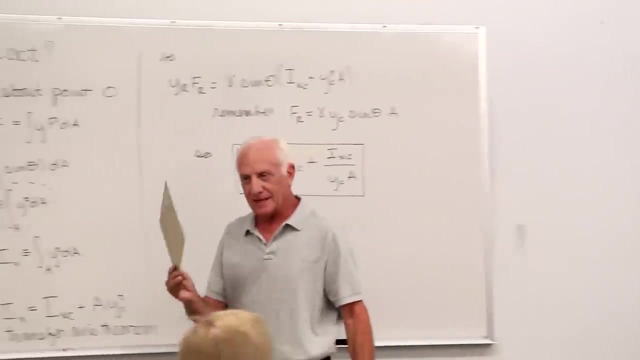 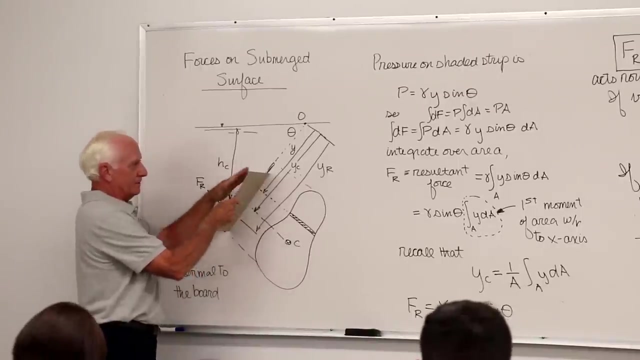 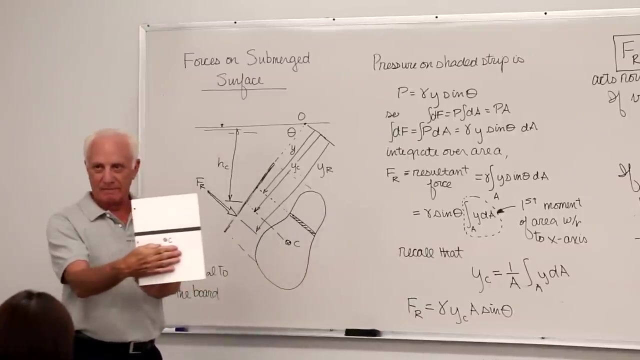 where the resultant force acts is a little bit more Down here. That's where F sub R acts. Big conclusion: Rectangular gate. Here it is Edge view. Okay, Where's the centroid? In the exact middle, The exact middle of the rectangular gate. 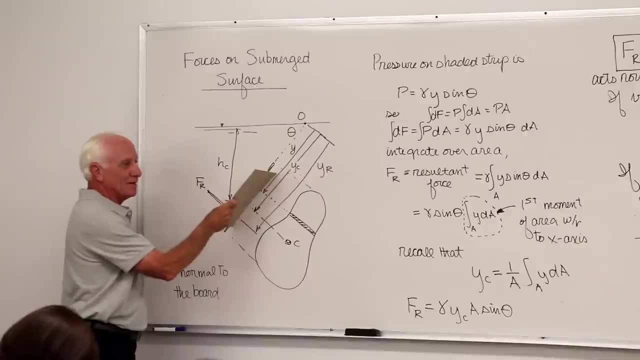 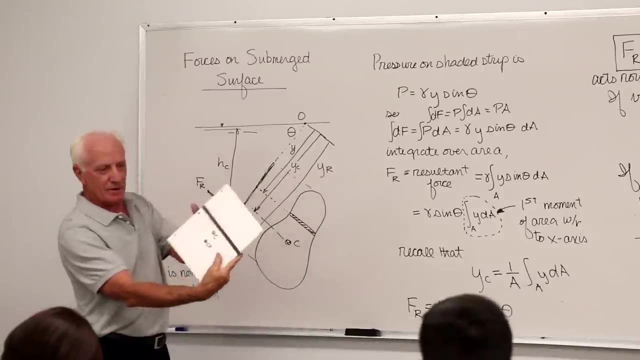 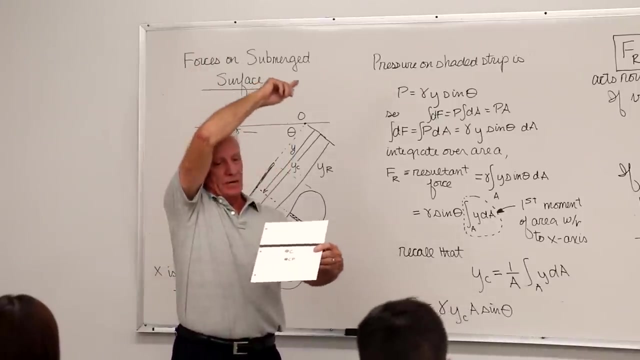 Where is it? Y sub R, Sometimes called center of pressure, CP Down further. Yeah, There it is. So here's the incline surface. Now the water's up there at the ceiling If you measure down from the ceiling on this plane. 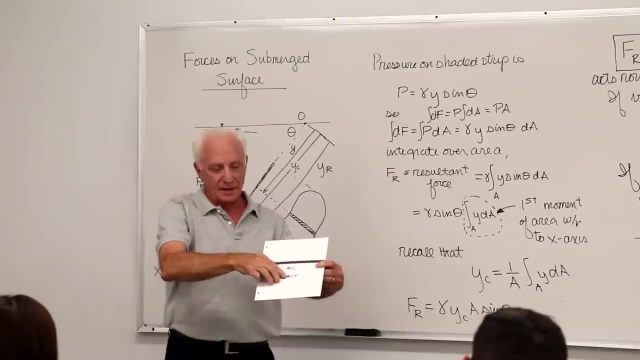 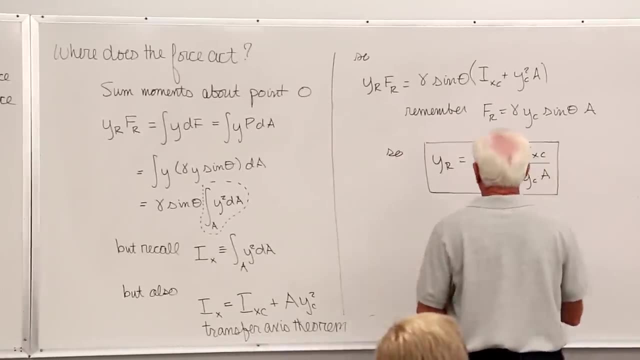 that's the distance down to the centroid, And add a little bit more And that's the distance to the center of pressure. So this is sometimes called the center of pressure. So let's do that in reverse. Let's do that in reverse. 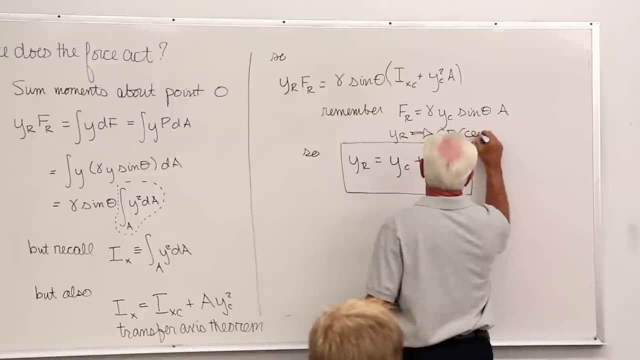 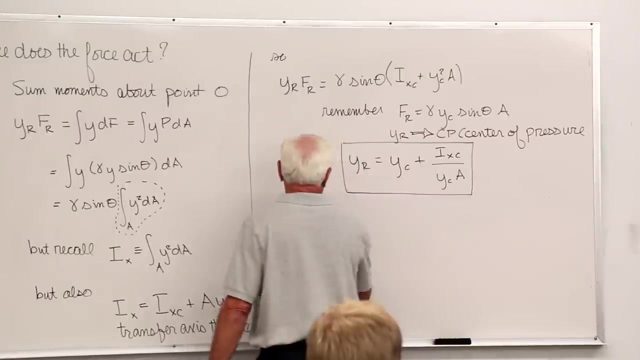 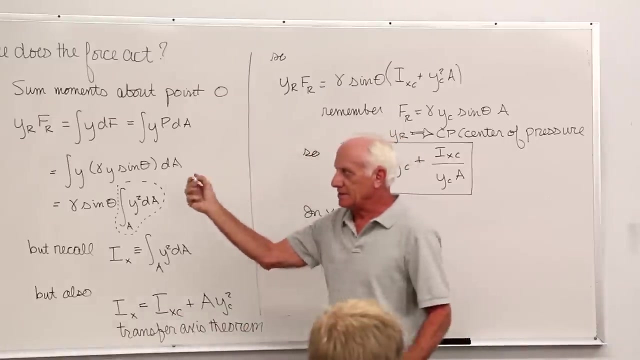 OK, Now we can do the same thing in the X direction, Which is out of the blackboard. Out of the blackboard Because the centroid- there's a word in there. It's called the centroid, Centroid. There's a value of Y for the centroid and there's a value of X for the centroid. 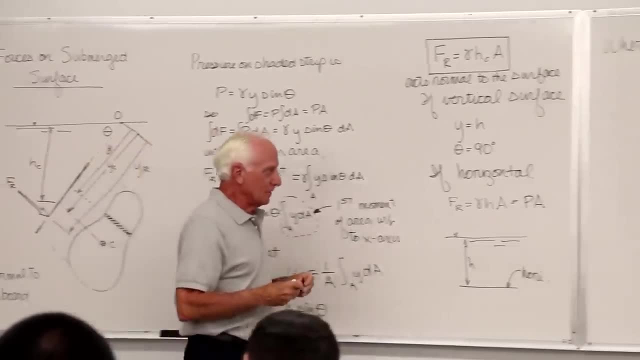 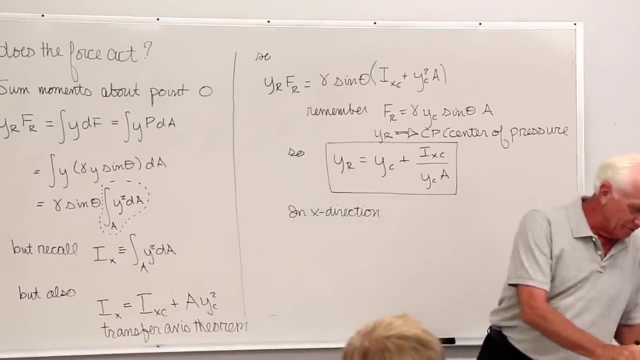 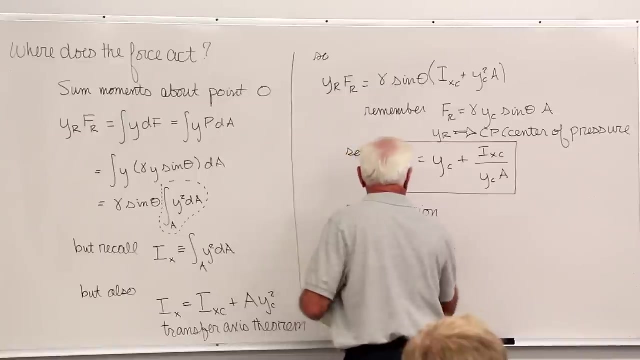 How far left or right is that? Okay, we're not going to go through it. You go through it very similarly and the results give you this: X resultant Equal X sub C plus I sub XY, product of inertia about the centroid divided by Y sub C times A. 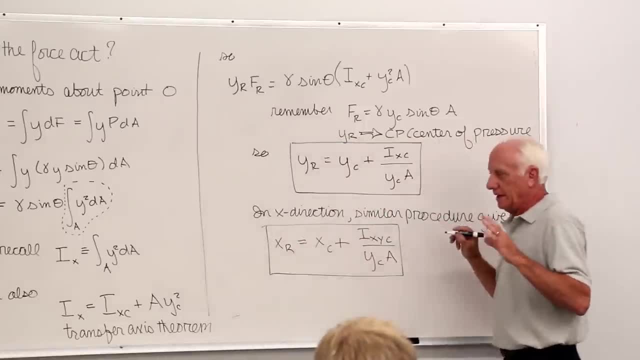 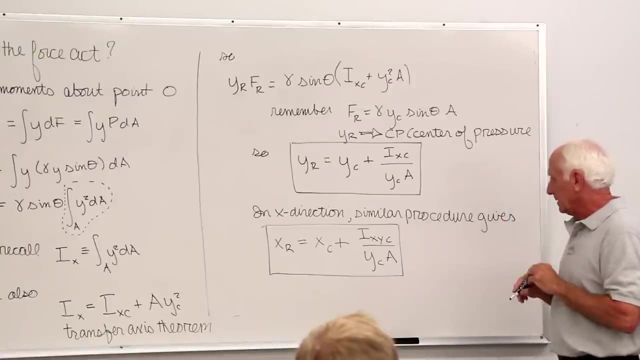 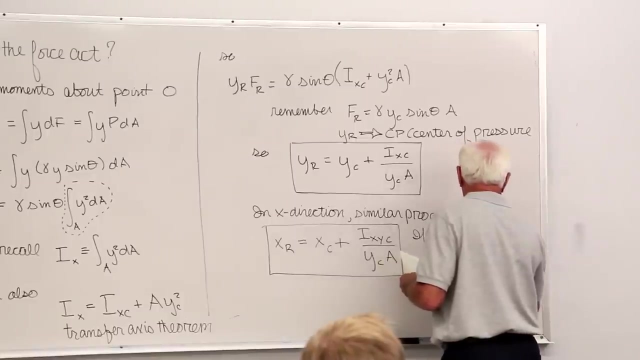 So that tells me, in the X and Y plane of that surface where the resultant force acts, I sub X by product of inertia. If either of these centroidal axes are an axis of symmetry, I sub X, Y, C equal to zero. 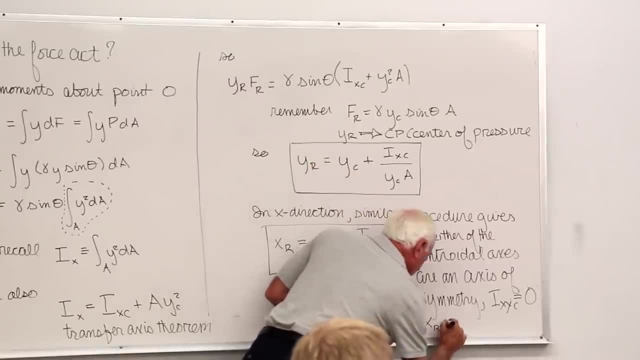 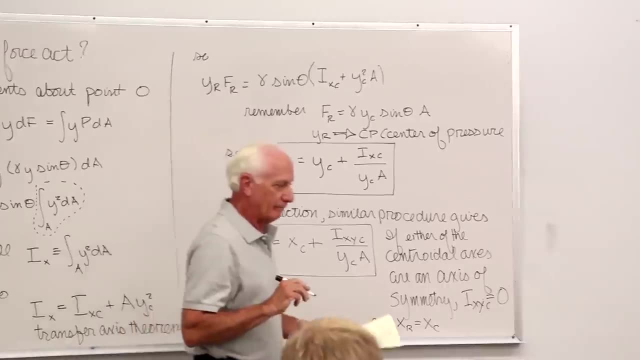 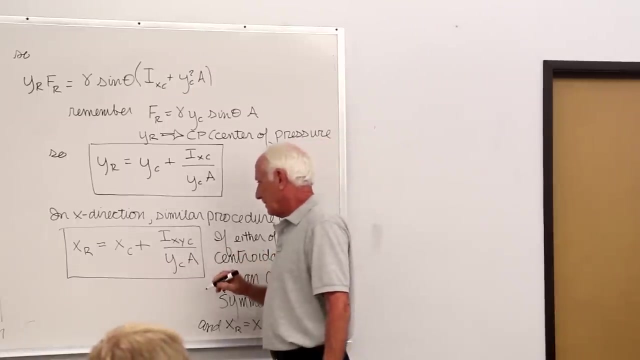 And X R equal X C. Is the last variable of I X Y. X R equal X C over Y C A. Is that dependent on the depth? why it's still Y. Why it's still Y. 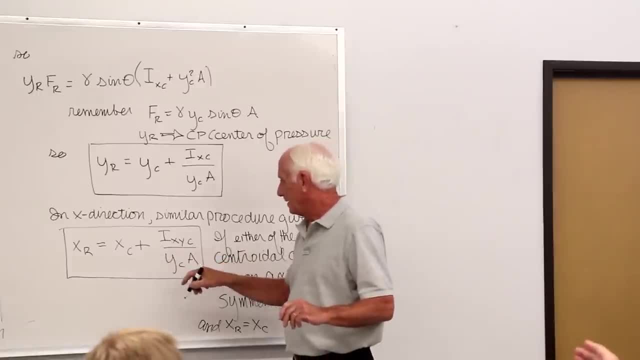 Well, I was curious, because X R equals X C, I was wondering why it wasn't X. Oh, oh, oh, yeah, yeah, These guys are both Ys. That guy's an X, He's a Y. 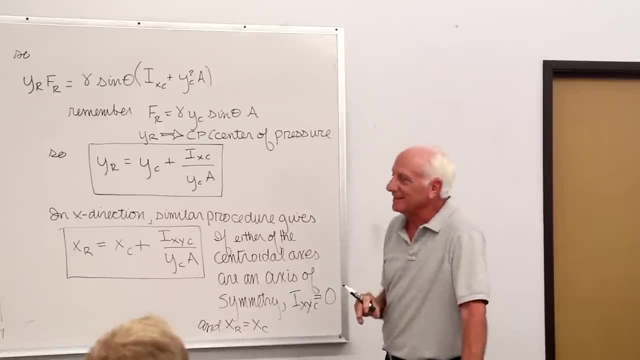 And that's because it's dependent on the depth. Yeah, it's the depth, Right, exactly, It came in that force. you know the force equation, Yeah, which is a function of depth, Mike, just to note down here. 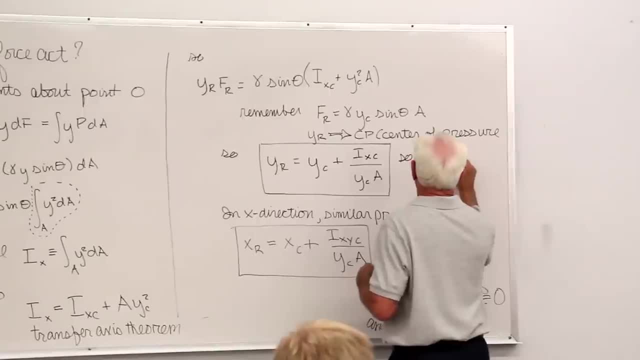 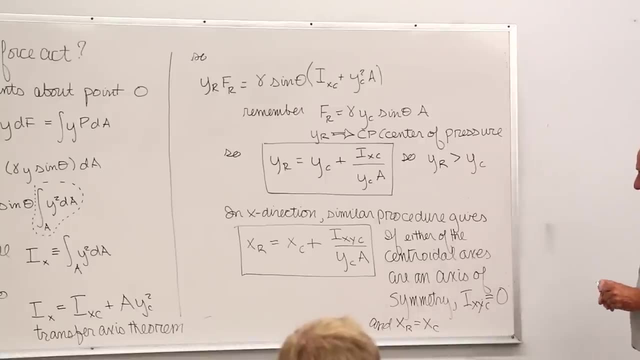 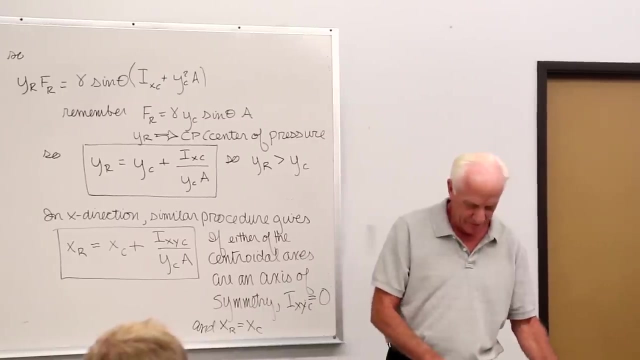 So the conclusion? The conclusion is Y sub R is always going to be greater than Y sub C. It will always be further down into the fluid water. for instance, And in the textbook, chapter 2, figure 218, I'm going to give you all the I. 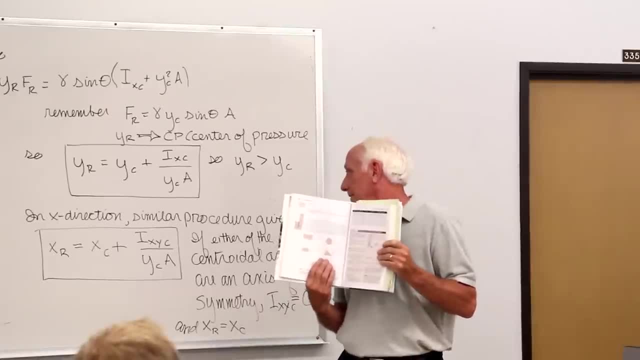 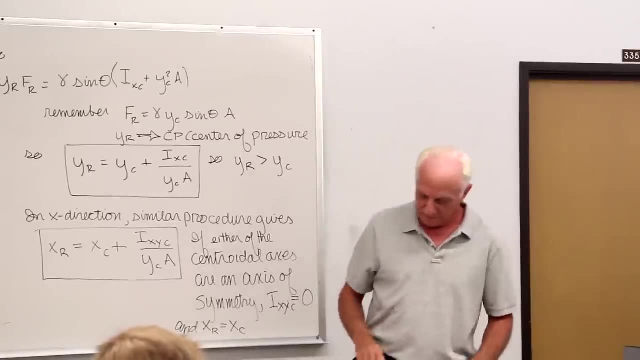 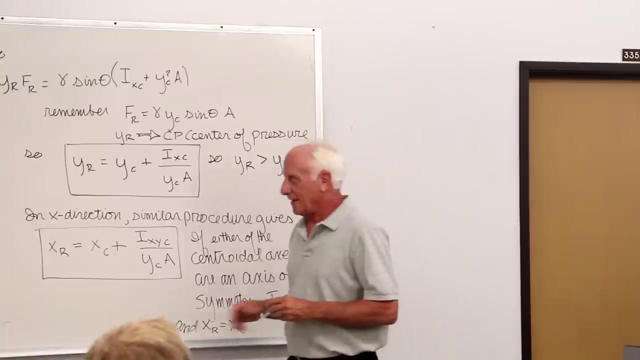 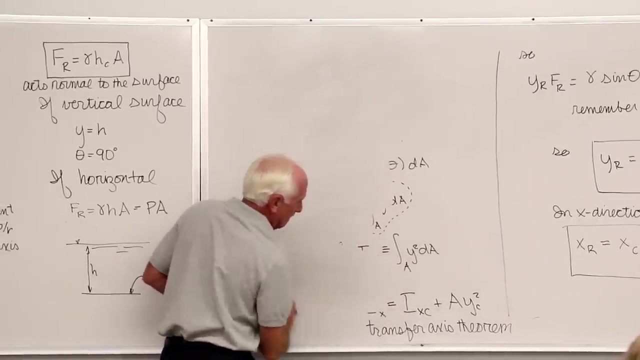 Sub X Cs. they give you all the I sub X, Y Cs. Here they are for all kinds of shapes. Okay, Just so you I'll just I'll point a couple things out from that table there, All right. 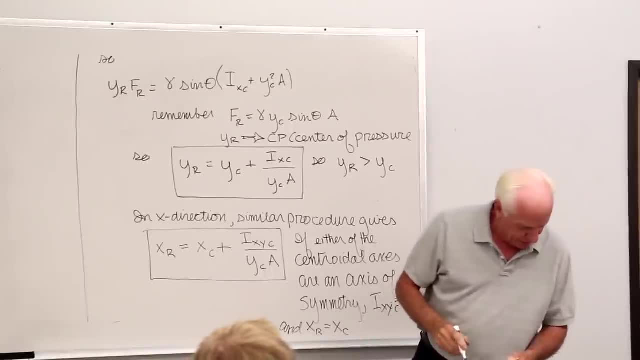 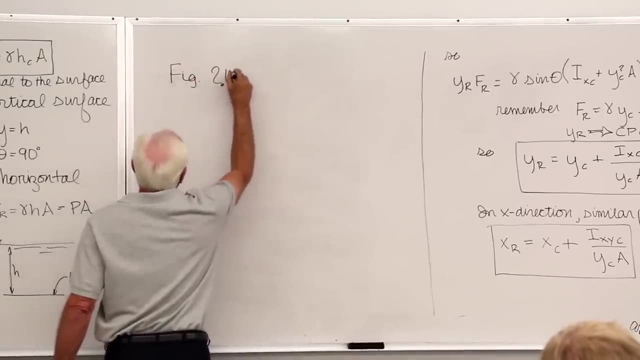 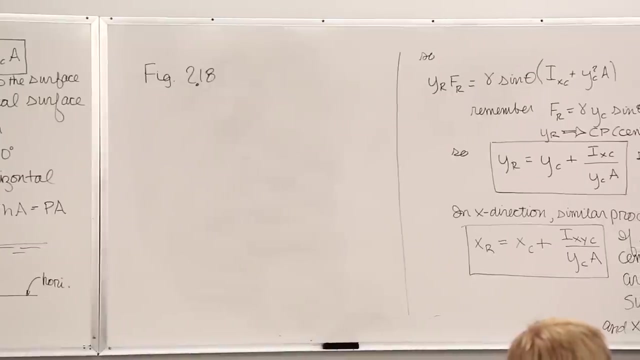 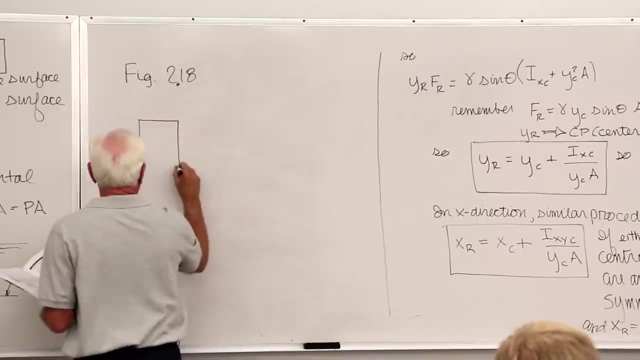 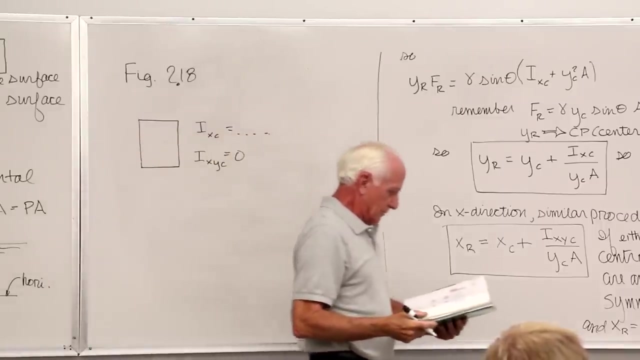 Here's figure 218, geometric properties, figure 218.. Okay, I'll just put a couple up here. Rectangular: Okay, He gives you: I sub X C, I sub X Y C, I sub X C, 1, 12, V, H, Q, 3, 0.. 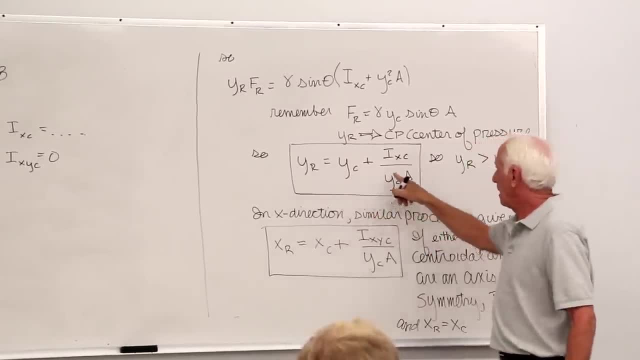 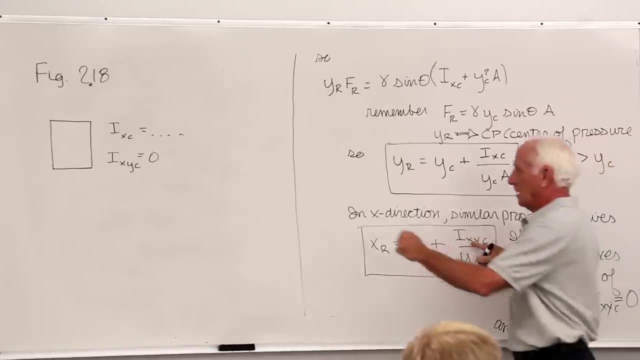 So if you want to find Y sub R, that's what goes in there. You want to find Y sub R, that's what goes in there. You want to find X sub R, that's what goes in there. a 0, a 0.. 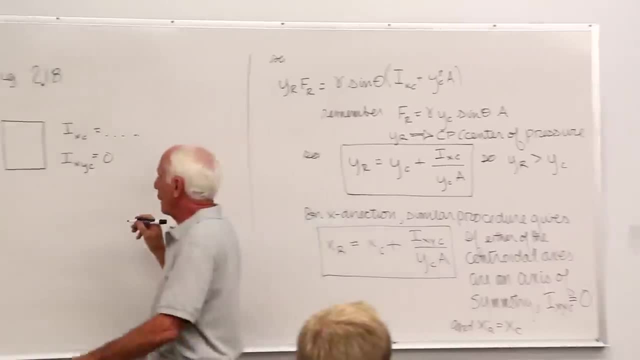 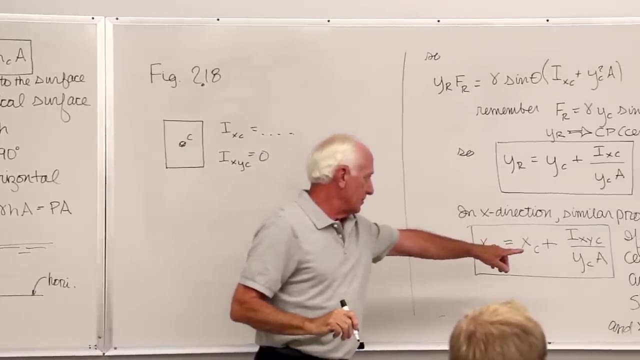 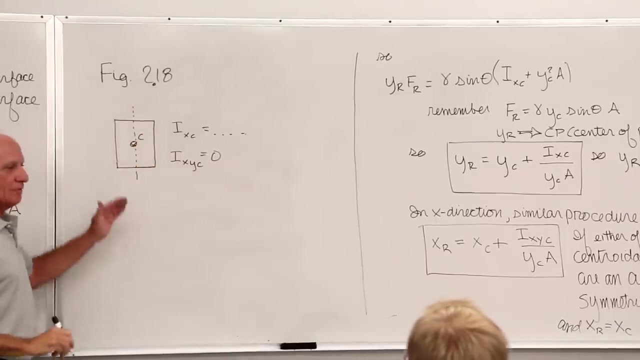 Y. where's the centroid there? If either of the centroidal axes are axis of symmetry, take the vertical one. is that vertical line an axis of symmetry? Of course it is. Fold it over, perfect fit. Is that axis? 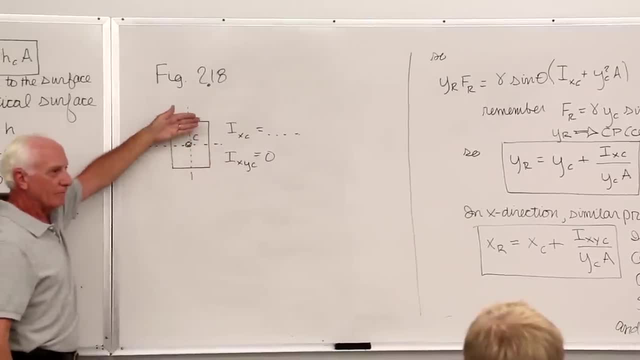 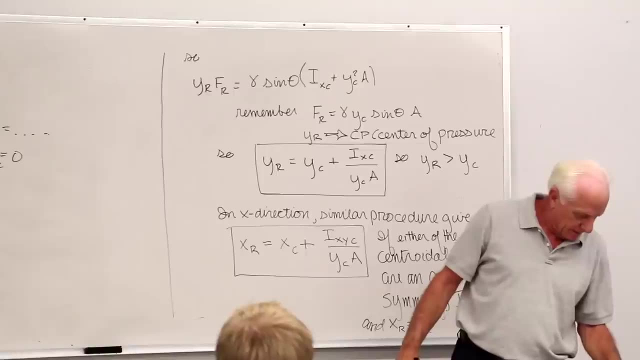 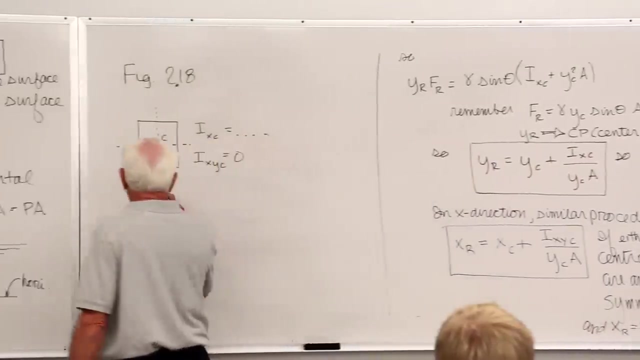 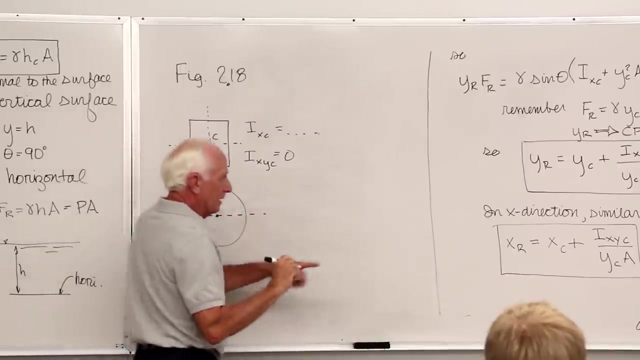 An axis of symmetry. Of course it is. Fold it over, perfect fit. Okay, That's what it means by this comment. Take another one: Circle Centroid. Centroidal axes means an axis that goes through its centroid In the X direction. 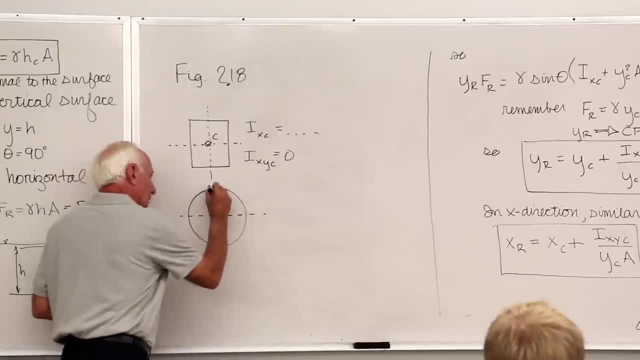 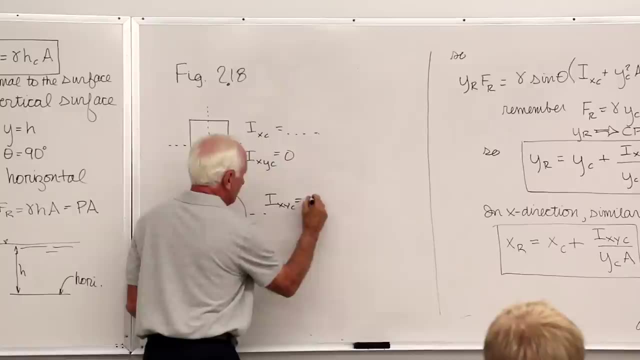 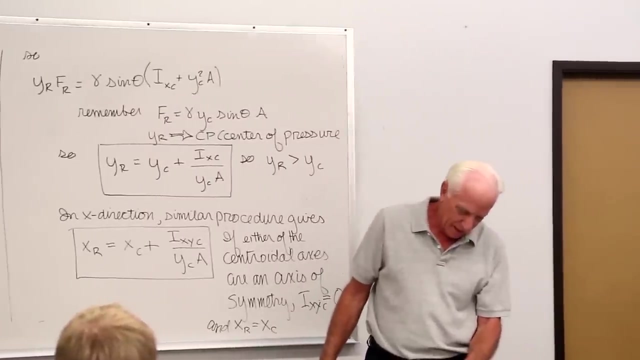 Yeah, Axis of symmetry In the Y direction. Yeah, Axis of symmetry. I sub X, Y, C equals 0. I sub X is not 0. Give it right there. I sub X Pi R to the 4th divided by 4.. 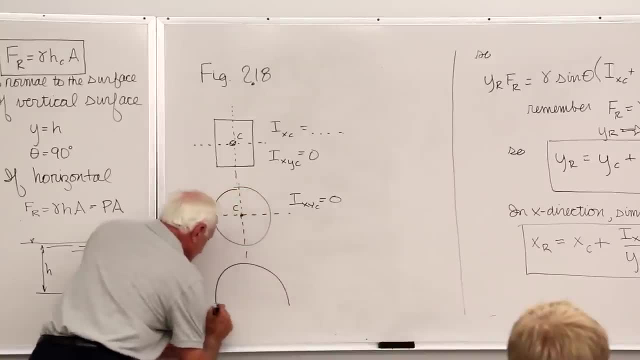 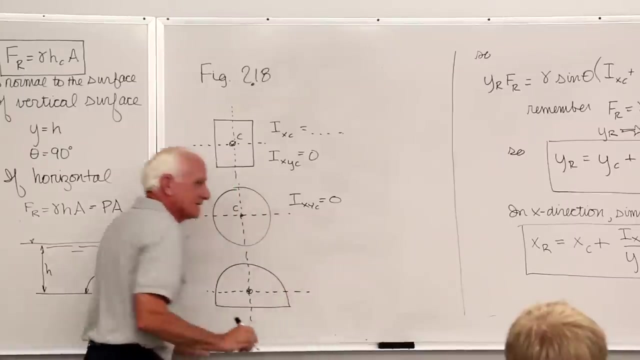 Take this one Semicircular area: Centroid Y axis, Yep Y axis of symmetry. Uh oh, Here it comes, X axis. No, it's not an axis of symmetry. I sub X, Y, C is not 0.. 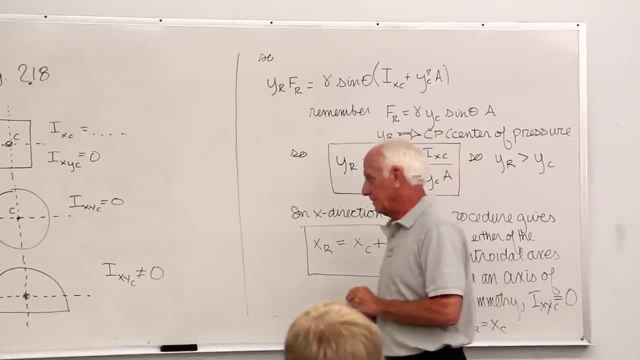 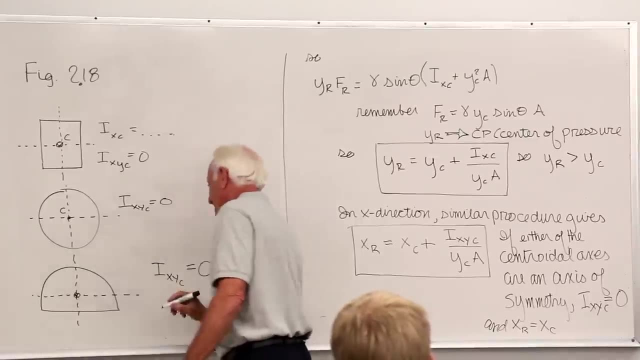 It's got a value here. Okay, I sub. X is not 0.. It's got a value here? Oh, I'm sorry, Is zero, I'll get one. that's not either one or the other, but that's okay. 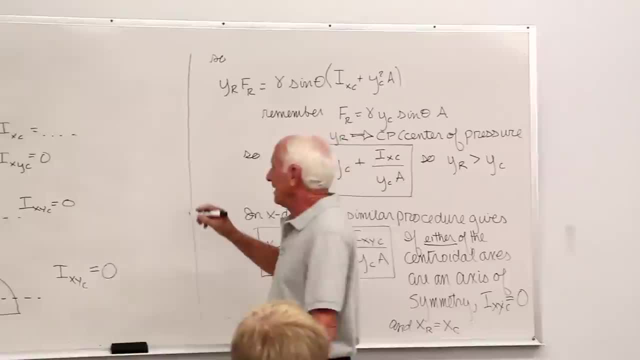 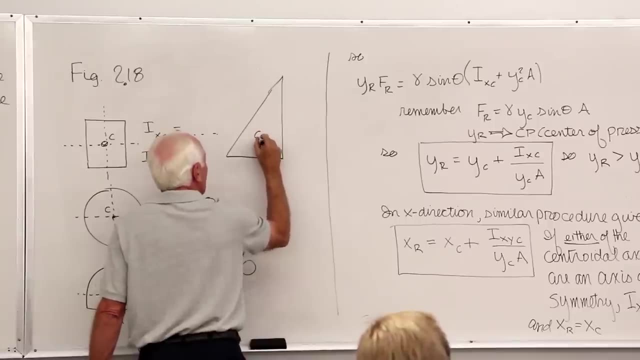 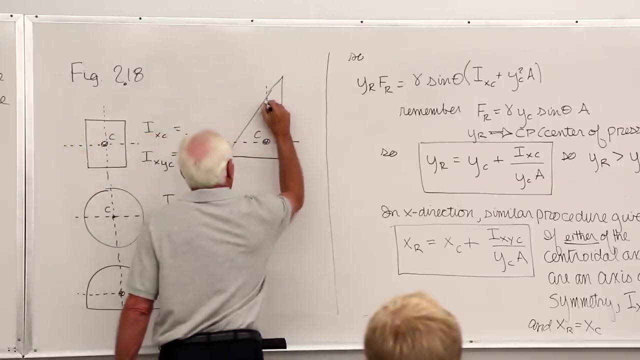 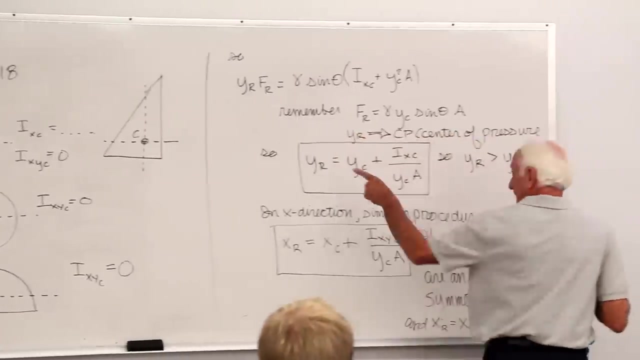 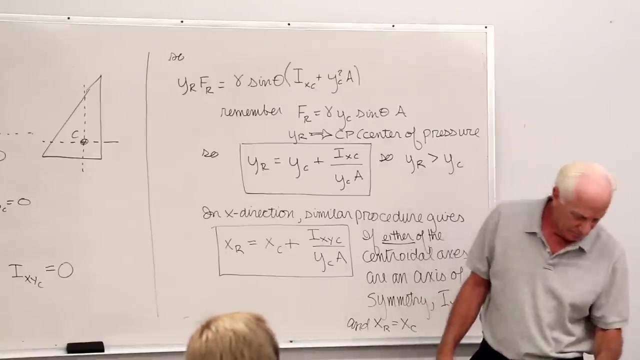 See the word either. Okay, now let's take this one Jump ahead of myself. Centroid Axis of symmetry- No. Centroid Axis of symmetry- No. Now, neither are axis of symmetry. It's not zero, It's given right there the love. 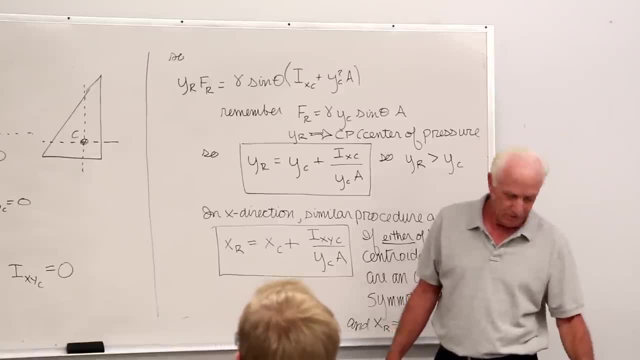 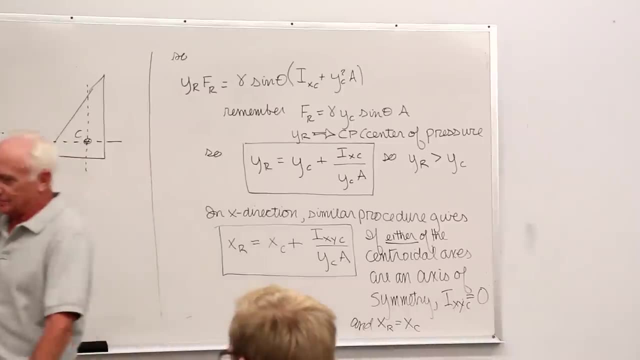 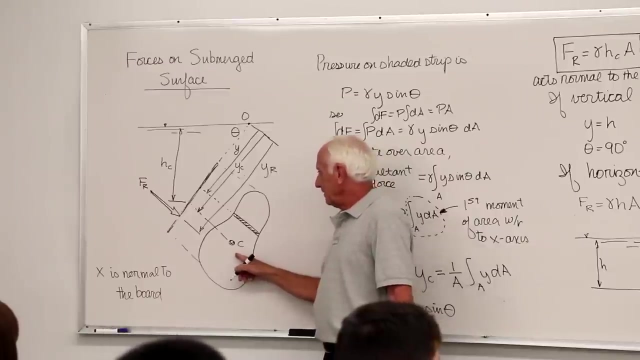 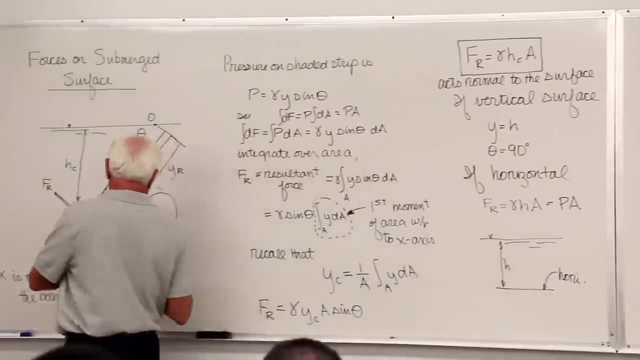 expression, but it's in table, our figure 218.. Okay, so that's what it means Over here. the answer is no. no, The axis of symmetry, No Y axis, No X axis, you know for that one right there, there would be a shift from the centroid to. 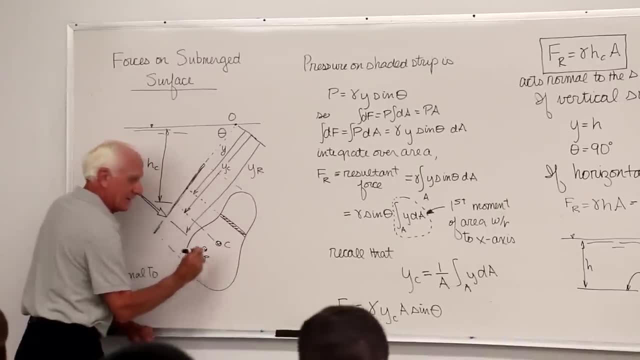 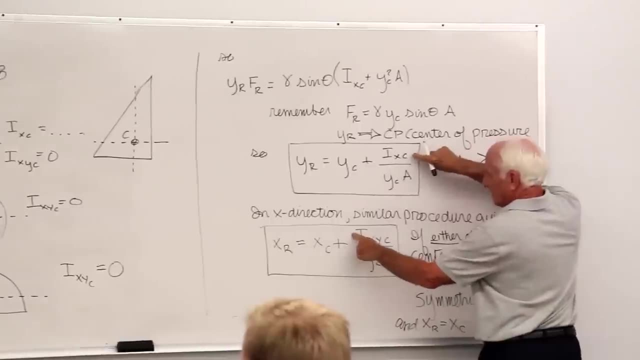 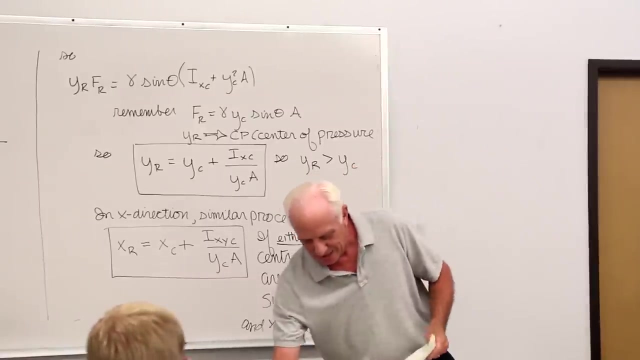 center of pressure might be over here somewhere. It's an X shift and a Y shift, because these two modes of inertia are not zero. in that case, Okay, big long story, but just so you know how to read that and do that, Okay. 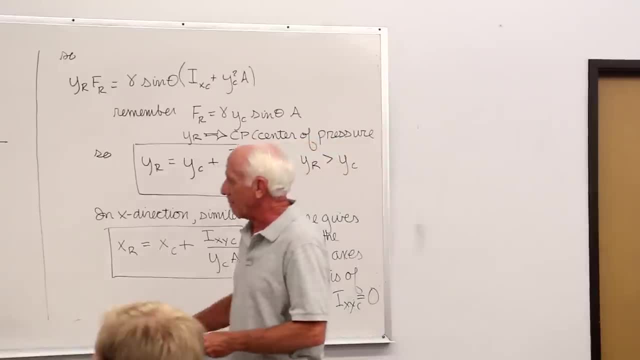 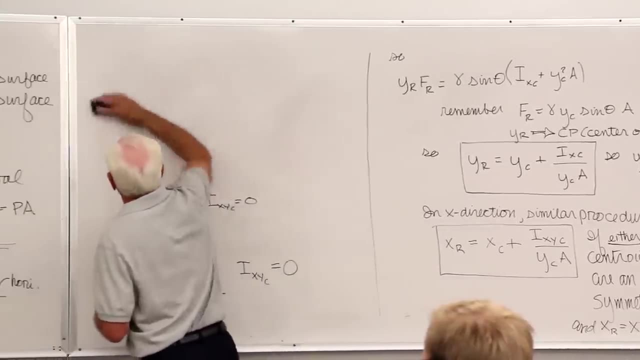 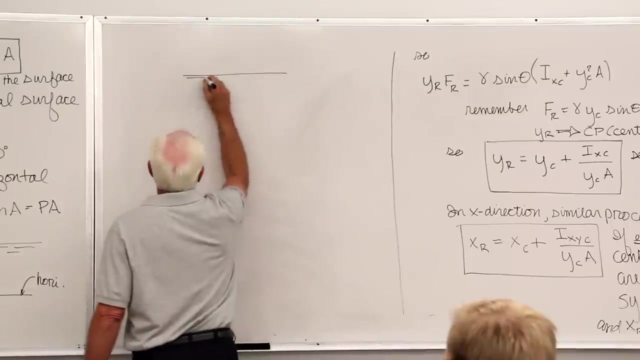 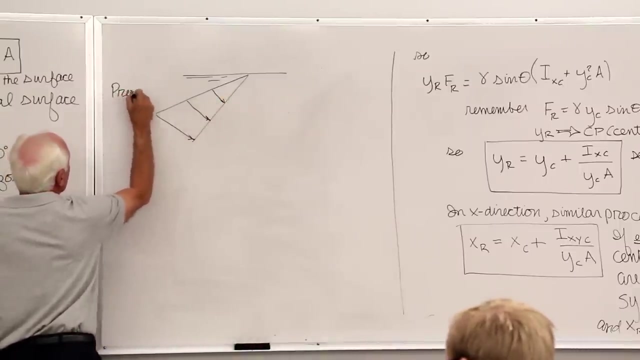 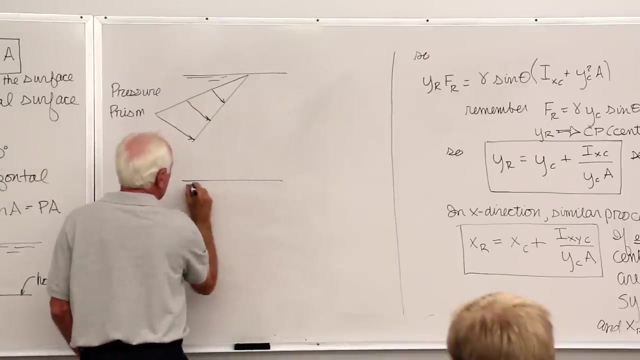 Let's see, I raised a figure I wanted to show you real quick. Let's just so you know nomenclature. This guy here is the pressure distribution. This guy is called pressure prism, Or this one is called the pressure prism. 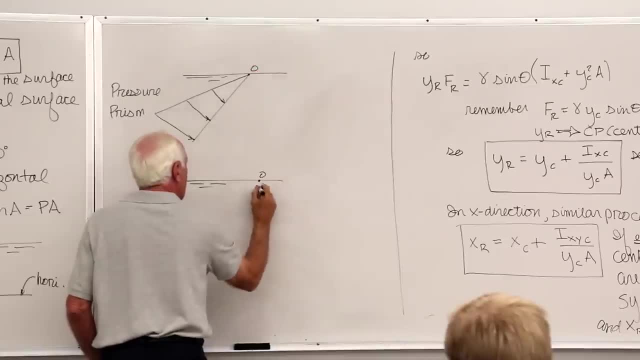 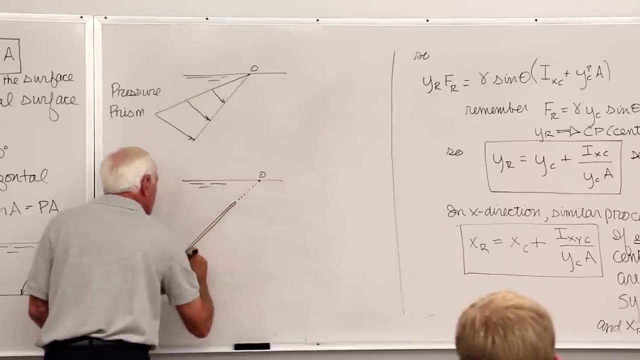 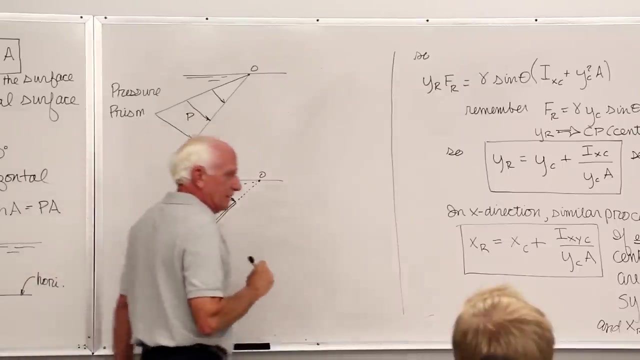 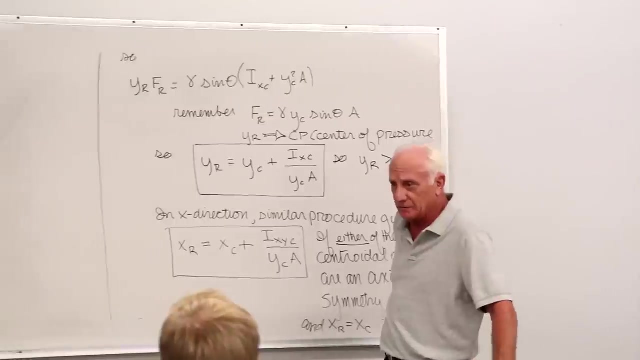 This is a prism here, Okay, The shape of it. So in case you see the word in the textbook, pressure prism, you can solve some of these problems by using the pressure prism, sometimes relatively easily, especially for rectangular plates, but for other shapes not so easily. So 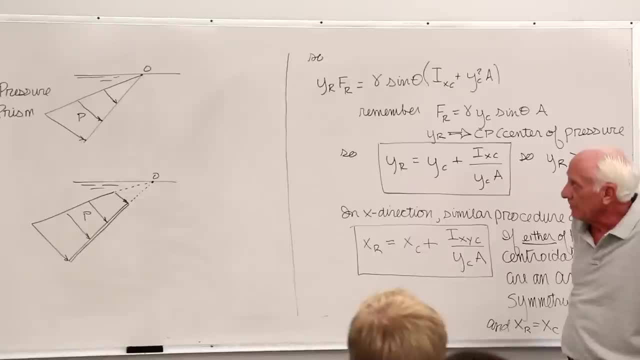 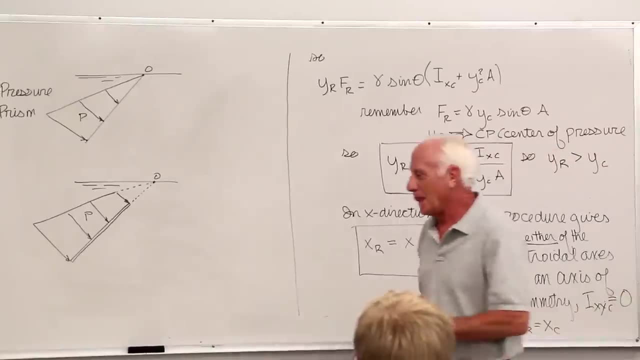 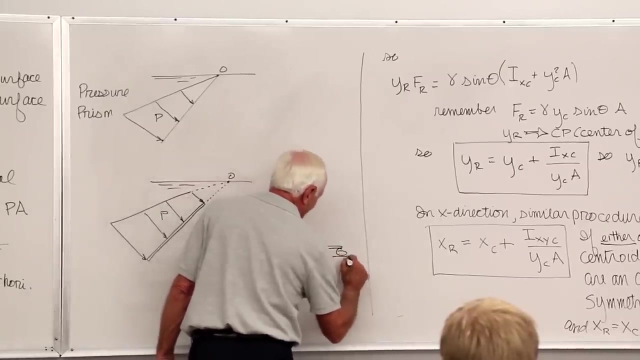 it's another alternative to solve for the resulting force. It of course it's. If you have statics, you know, you know I'm not going to go through it because you know what you've done before in statics, I'm sure. 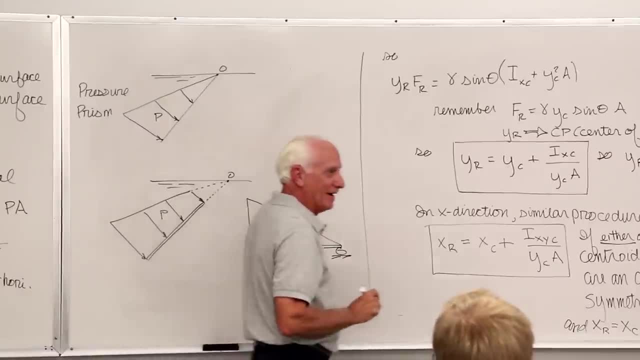 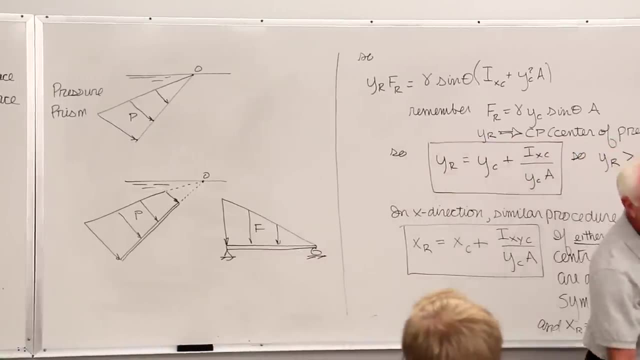 Go ahead, Find the resulting force on that load and then find the reaction under point A and B. You've probably done it many times in statics. Does it look like the fluid problem? Oh, of course it does. Just turn it 90 degrees. 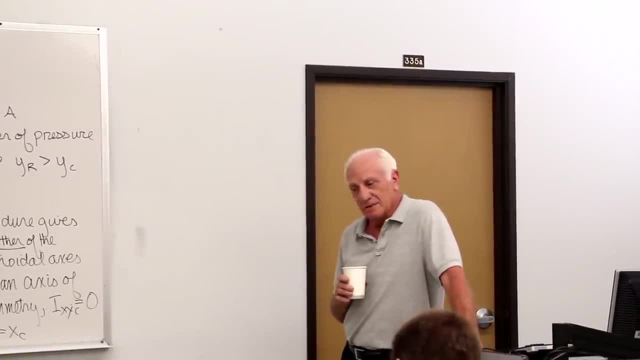 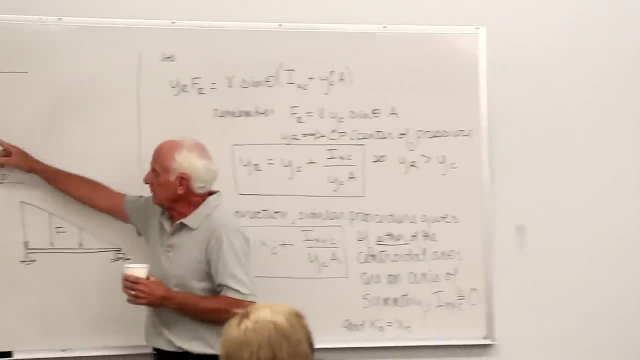 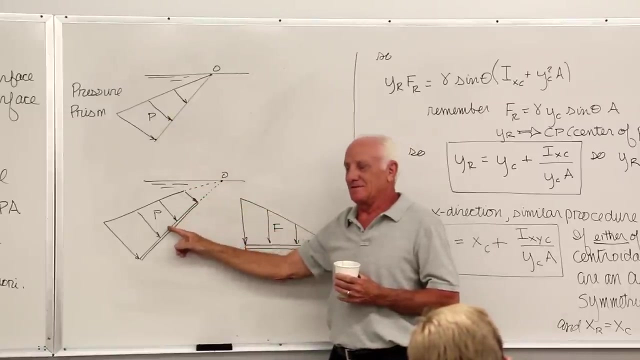 Do you solve it the same way? Pretty much so. Yeah, Uh-huh. Where does the resulting force act Through the centered of that triangle right here? Where does the resulting force act- It's a tough guy- Through the centered. 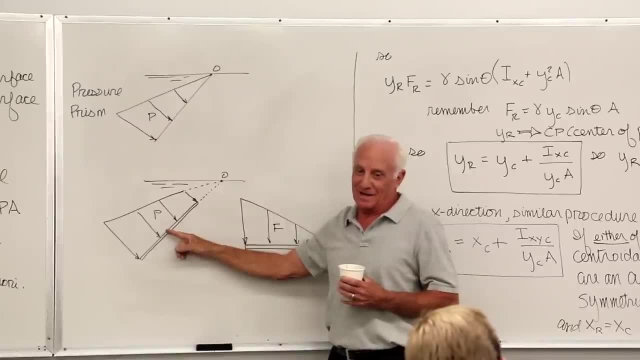 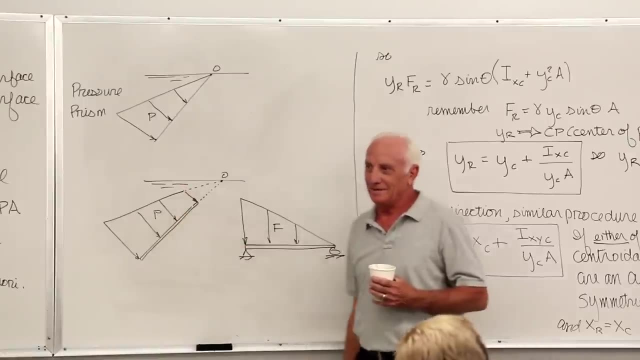 of the pressure prism. where is it at? I don't know, but I can find it. There's a rectangle here And there's a rectangle here- pardon me- and a triangle here. I'll do it piecemeal. You've probably done that in statics. 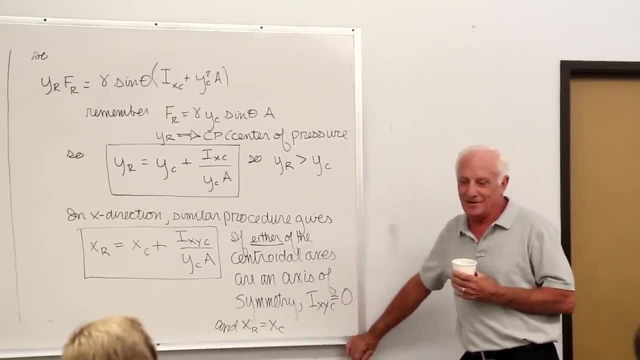 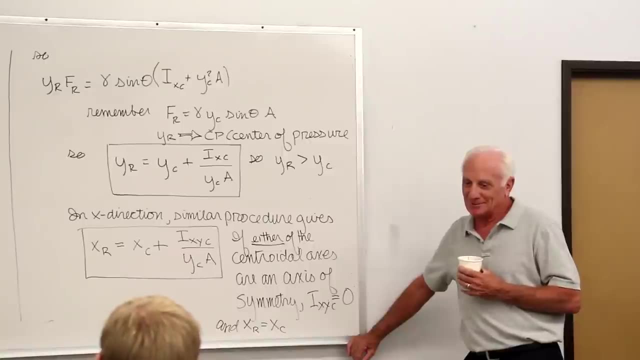 So that method works really nice if it's a rectangular area, but all things in the real world aren't rectangles- for gates and underwater windows and things like that. So you can use it if you want, but the sure way of doing it. 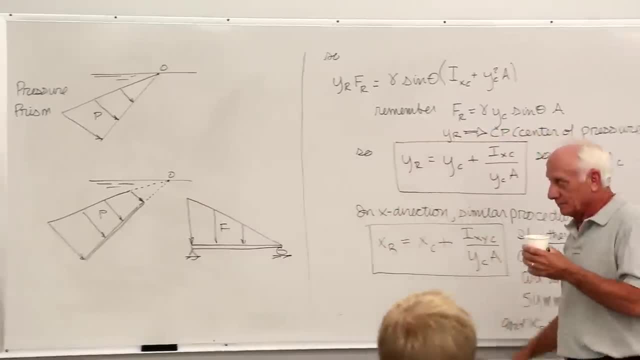 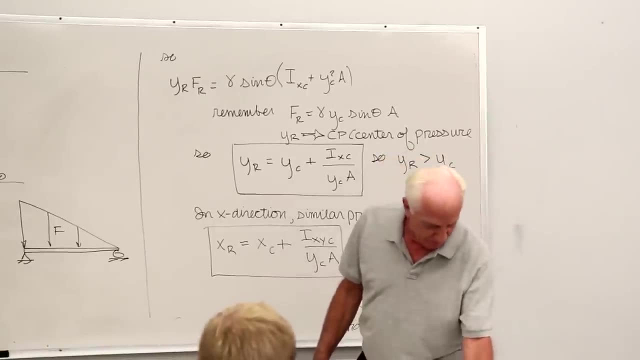 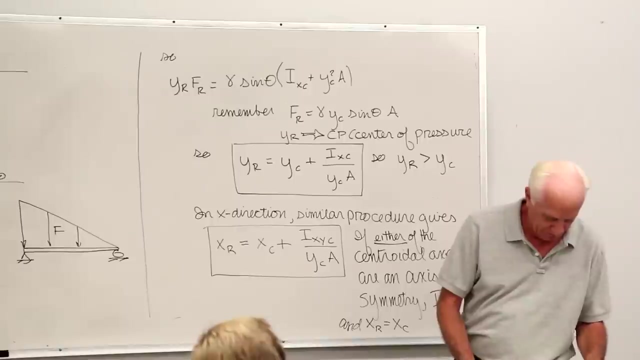 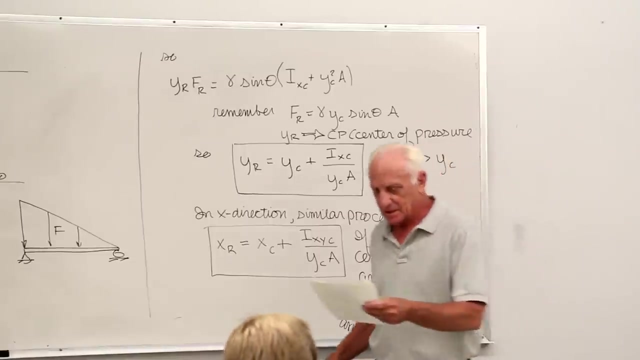 is the method I put over there and over here. But just so you know what the word means: pressure prison. Okay, now we're gonna take a couple of examples. The first one is gonna be a submerged circular area, So I'll start over here, I think. 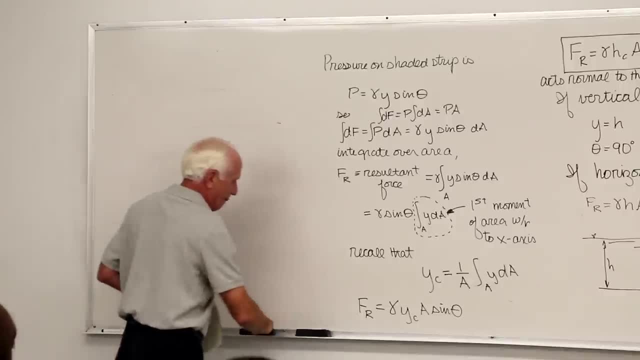 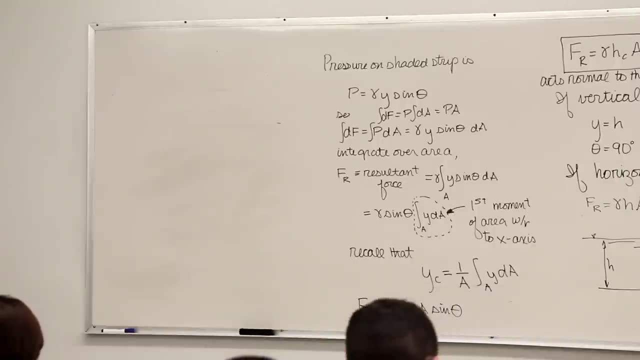 So I'm gonna take a lot of the apartment's直, so I'm gonna keep it here, I'm gonna put this one next to my有 And I'm gonna make sure that all of these are in this one. Now, this part's gonna be in the very middle over here. 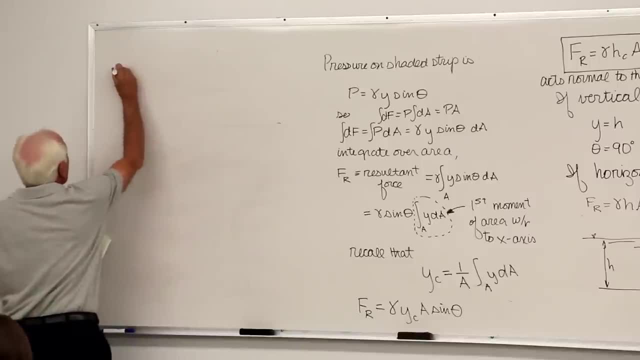 so I'll pull this out of the right part and it's gonna overlap right over here. So now I have my two attached. Now I've got the other one as well, So this part is gonna be on the left. 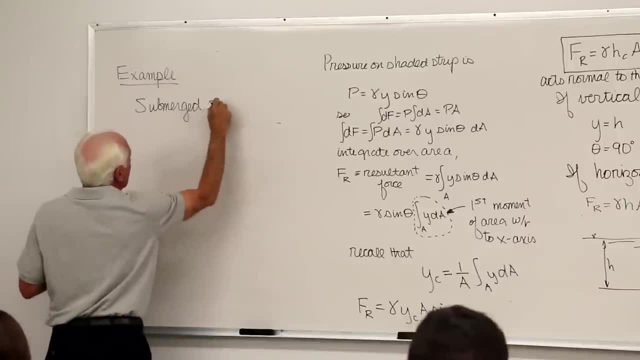 and this is gonna be on the right side. So I'm gonna cut a lot of this in the middle. right here, I'm gonna go over to the right side. Finally, I'm gonna go over that right there. There's a lot more to do. 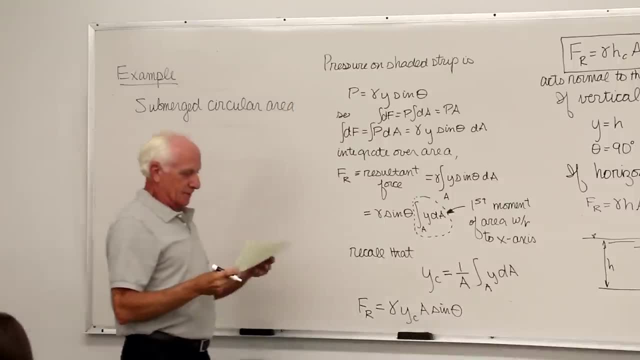 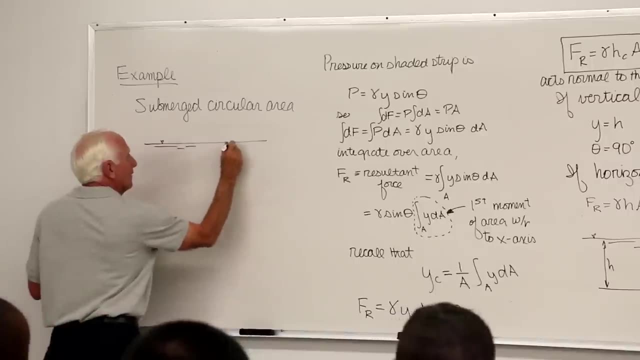 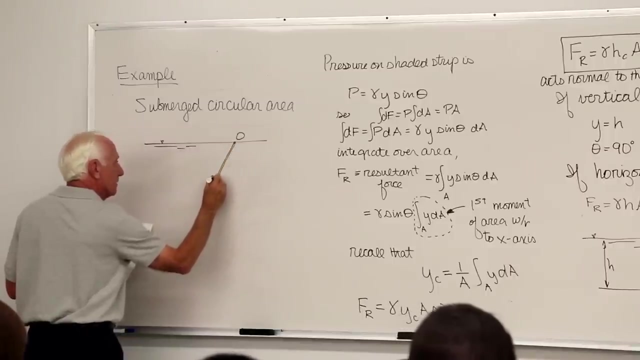 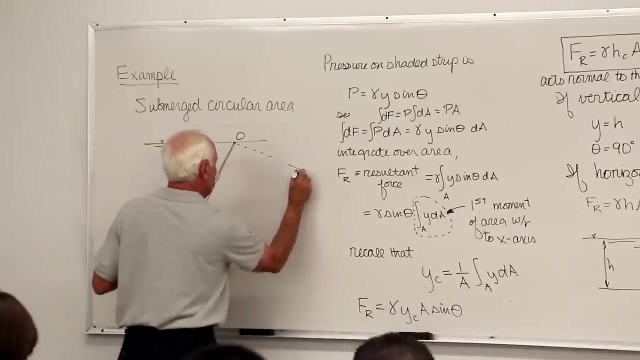 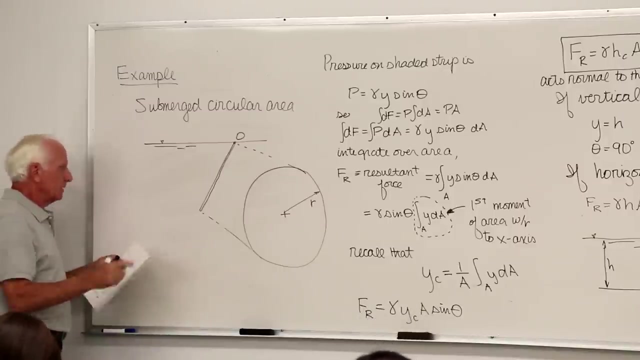 See what I mean. And let's see where I put that: Right on the free surface. So here's the free surface And here is the submerged circular area. So if I look down on that area it looks like this: The radius is r. 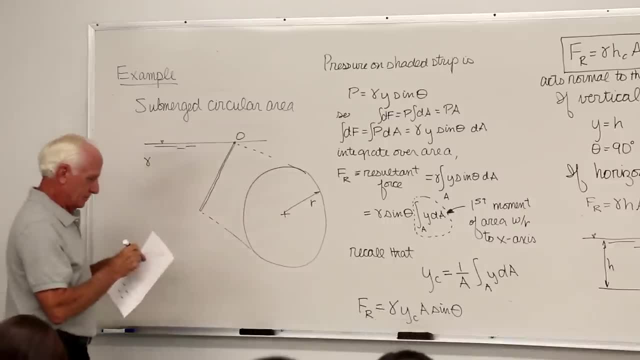 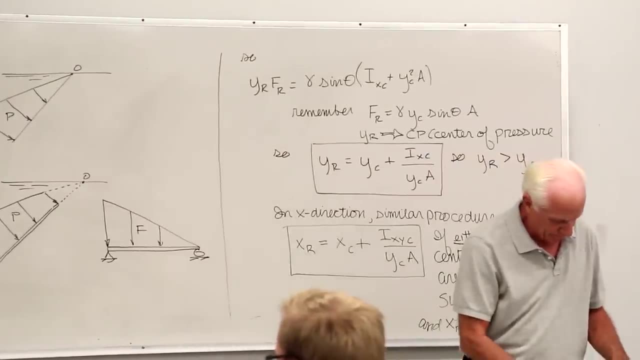 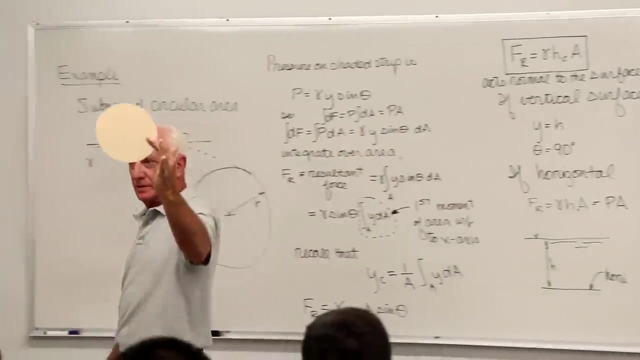 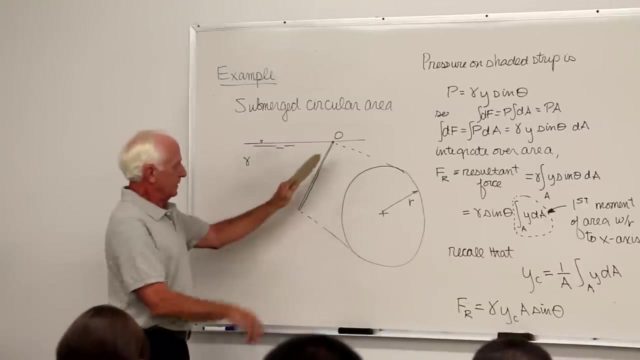 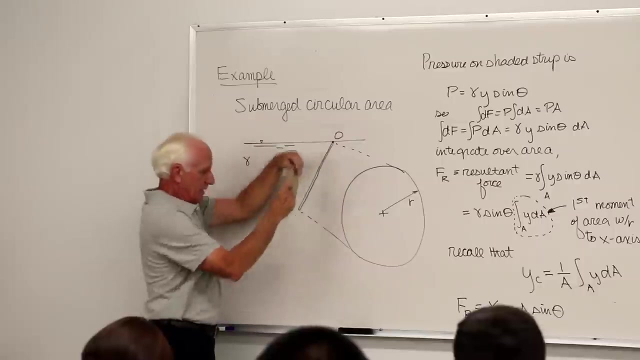 Fluid has a specific weight. again, There it is. It could be a windmill, It could be a window, Some submerged vessel. Okay, There it is like that It's touching the top Caught water, Touching the top of the water like that. 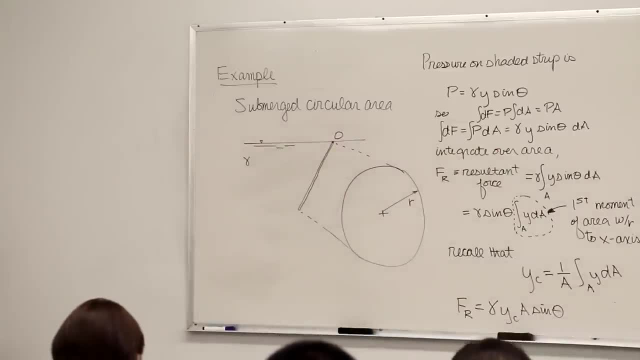 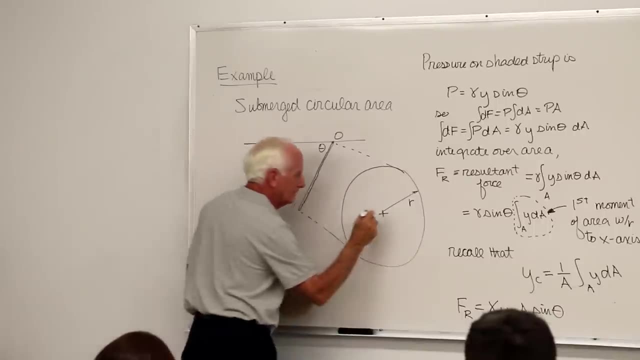 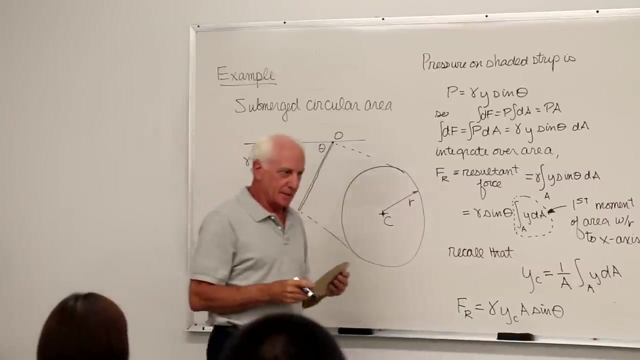 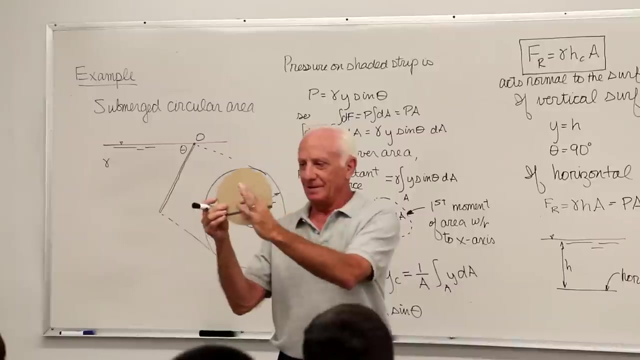 Inclined at an angle. theta, That's theta. there We know where the centroid is. Okay, I want to find the resultant force And then I want to find where it acts on the surface. By the way, if you want to play the same game before, you would draw a big, heavy dark line. 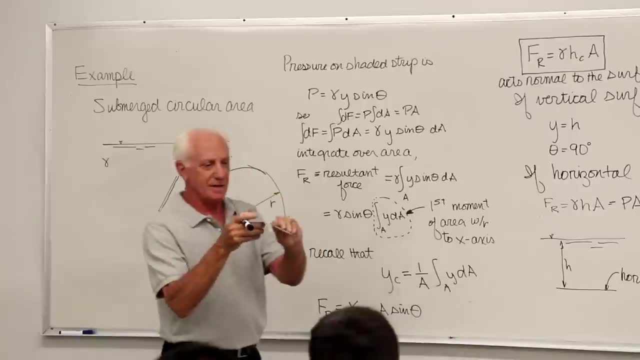 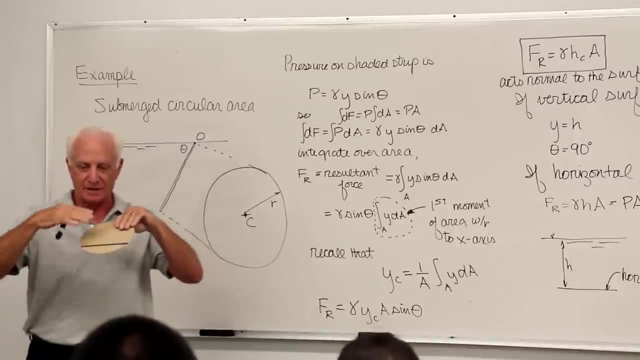 That would be a little differential area da. That's differential area da. And if I incline it like this, then the pressure on that line would be the same from left to right. Here's the top surface of the water. That pressure is constant. 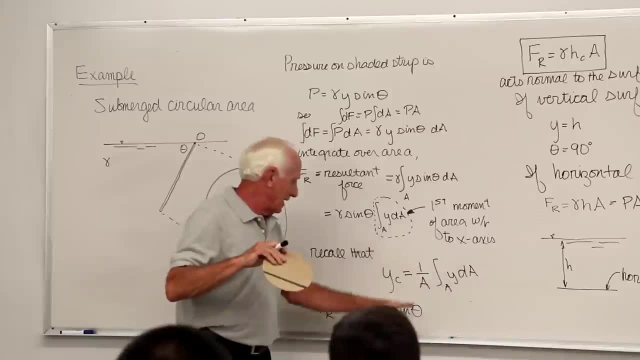 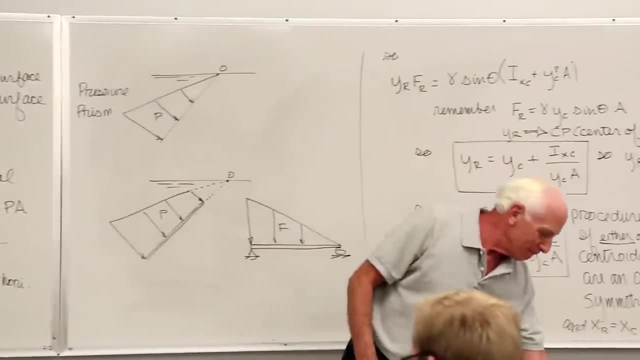 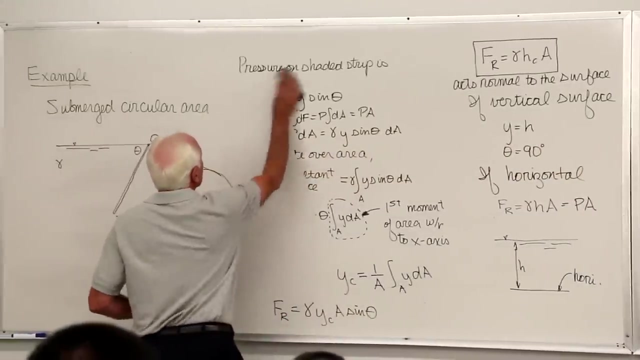 I go through the exact same thing here And end up with this guy right down here. Okay, So there is our F sub R. Let's erase this and put this up here. I'm not going to put numbers here, It's going to be in symbolic terms. 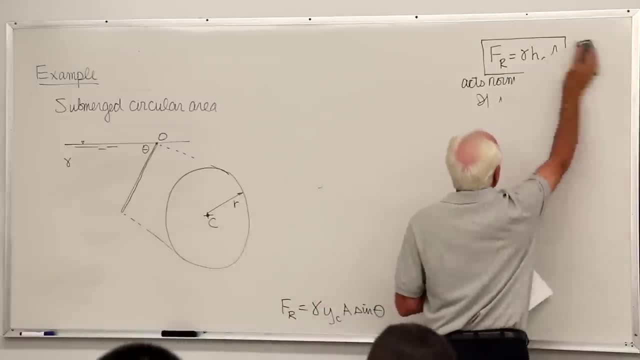 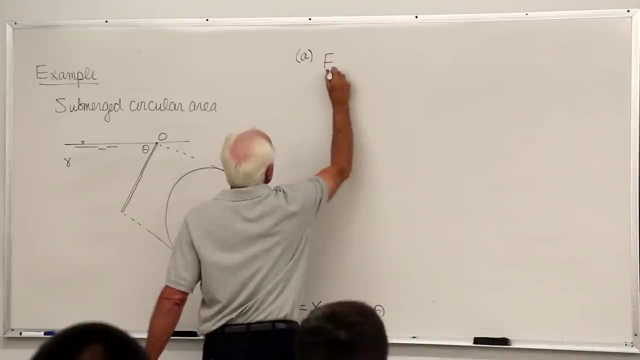 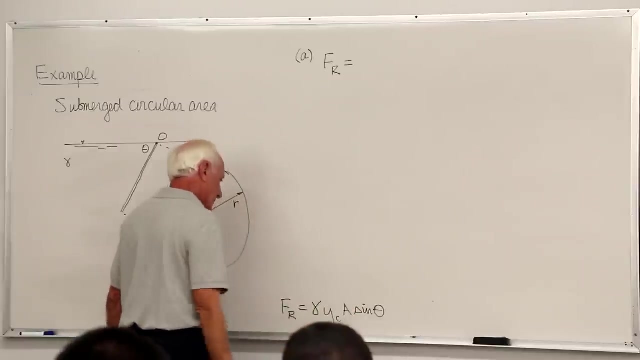 It's not horizontal, It's not vertical. Okay, So Here's our. A Resultant force is equal to like down here, This: Y sub C times sine of, let's just yeah, Y sub C times sine of theta. 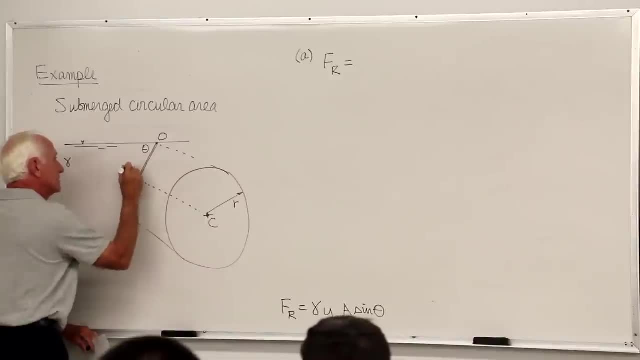 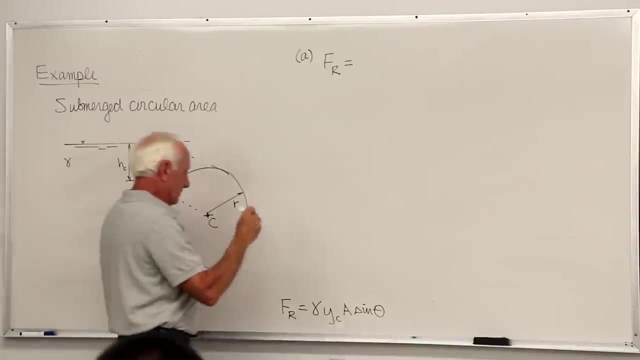 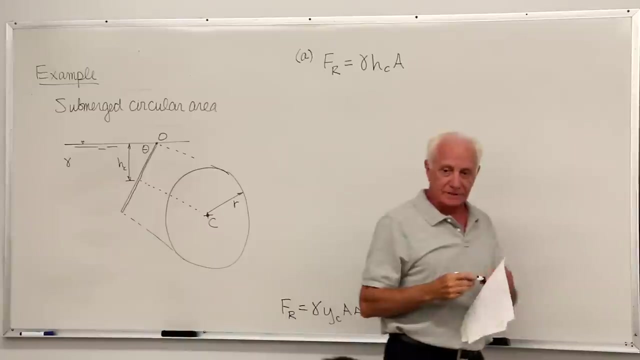 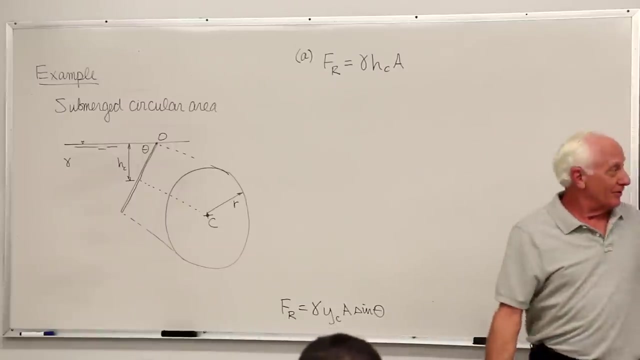 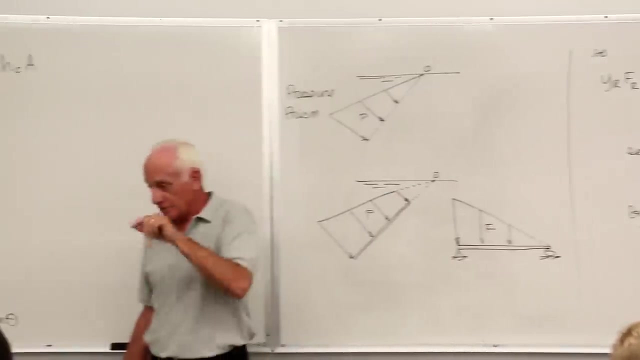 Here's the centroid. Here's the distance down centroid H sub C. Okay, So gamma H sub CA. See how far below the free surface the centroid is. That's called H sub C. Now I know I told you that where X is going to be below the centroid, further down into the water, 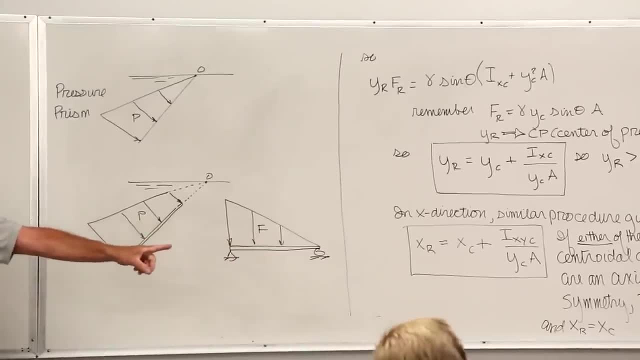 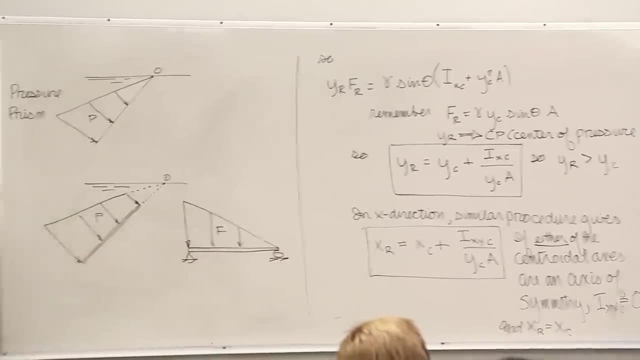 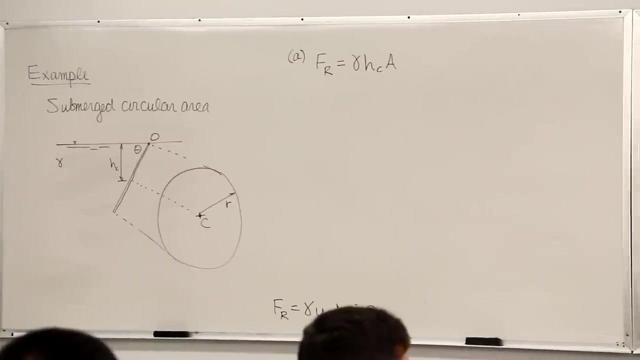 Either. in this case, both centroidal axes are axes of symmetry. Both are axes of symmetry. Therefore I sub. XC is zero, So it doesn't shift left or right. The resultant force doesn't act left or right. of that The resultant force is going to. here's the centroid. 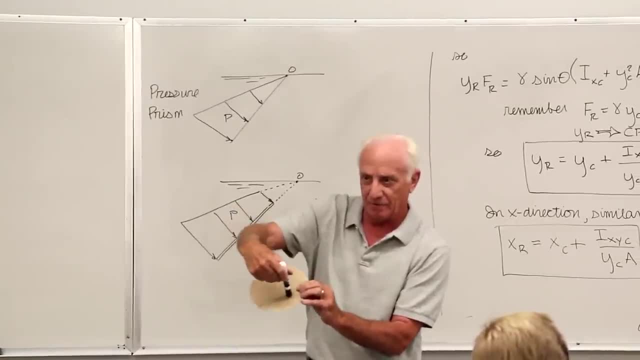 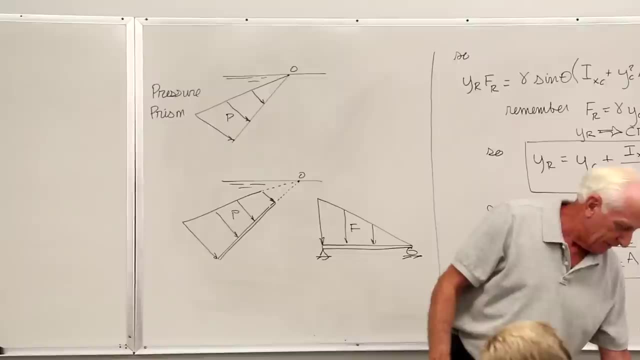 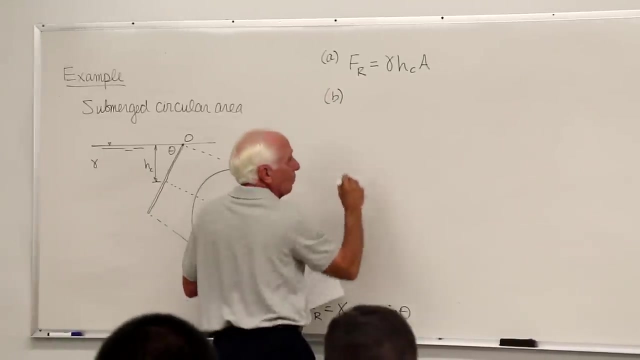 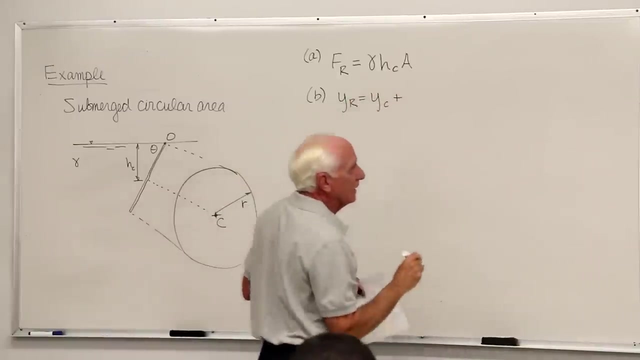 It's going to act down in the Y direction, but not left or right Doesn't make any sense, It's symmetrical. But it's going to act below the centroid, Below the centroid. Okay, Here's the equation: Y sub R, equal Y sub C, plus I sub XC, divided by Y sub CA. 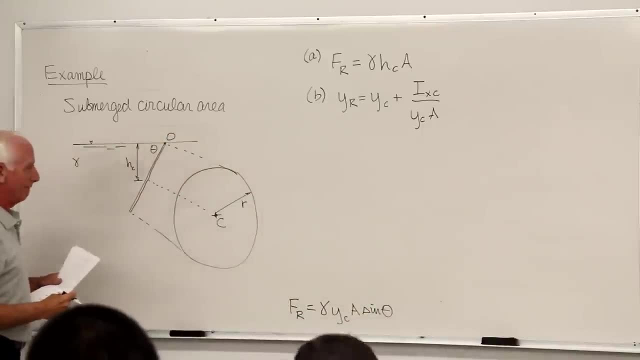 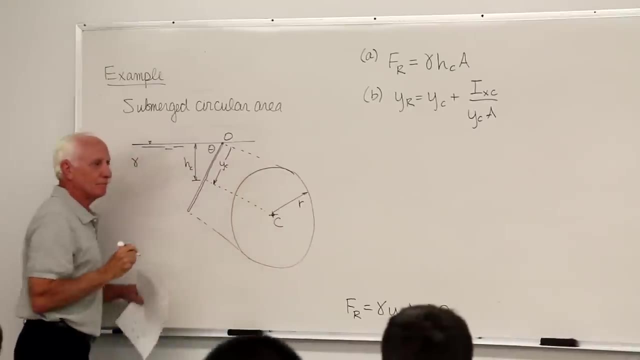 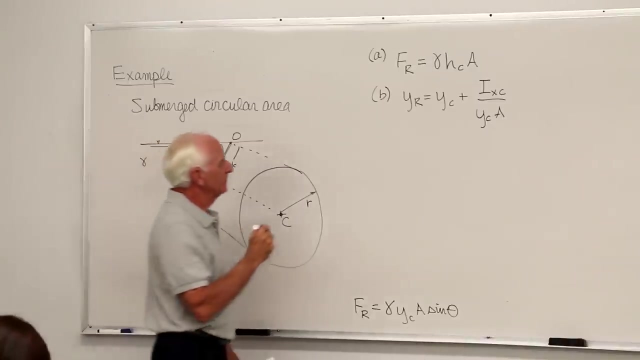 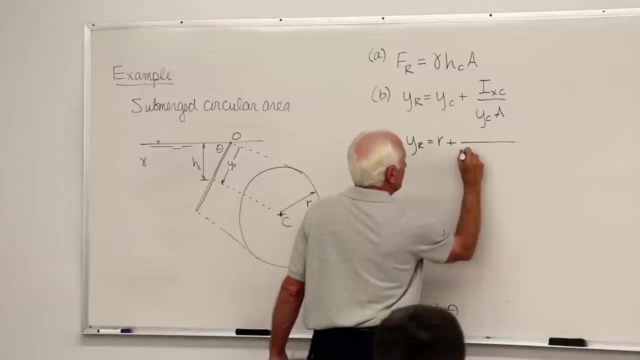 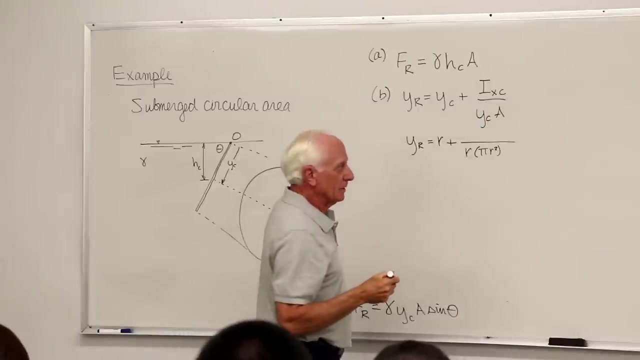 Okay, Y sub C There. Hmm, interesting Y sub C looks like it's just the radius. Yeah, it is Y sub R, equal the radius plus the radius area pi R squared. Now I sub XC, Go to table or figure 218.. 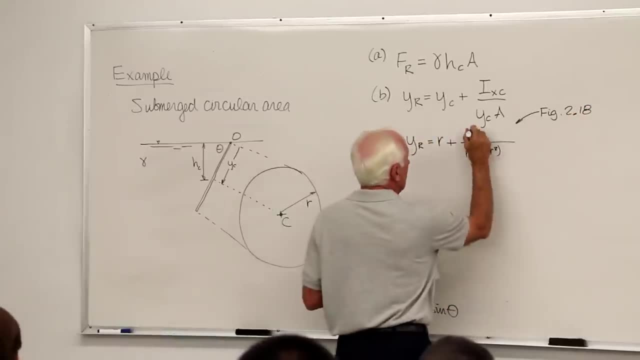 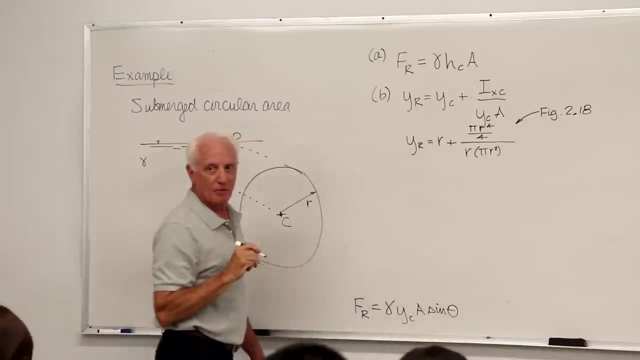 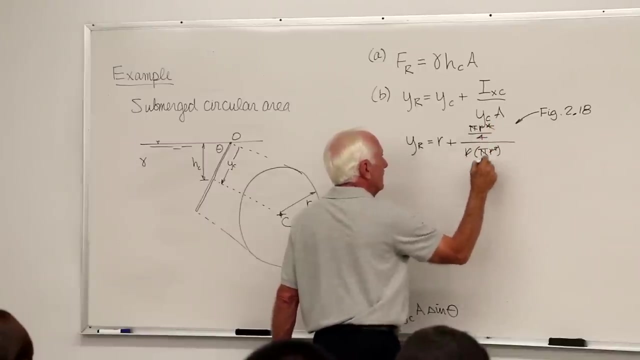 Pi R to the fourth over four, Pi R to the fourth over four. Pi count to a pi R, cubed R to the fourth. There R plus R over four. Yeah, So how much further down from the centroid is it? 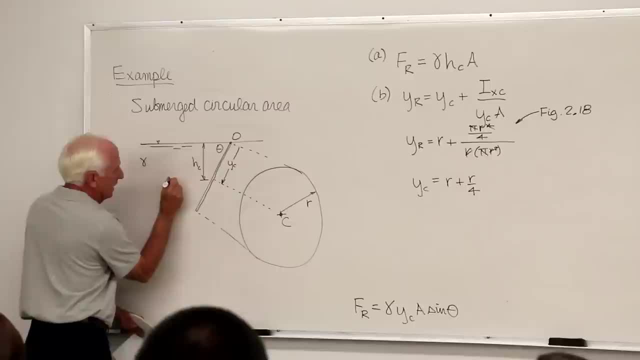 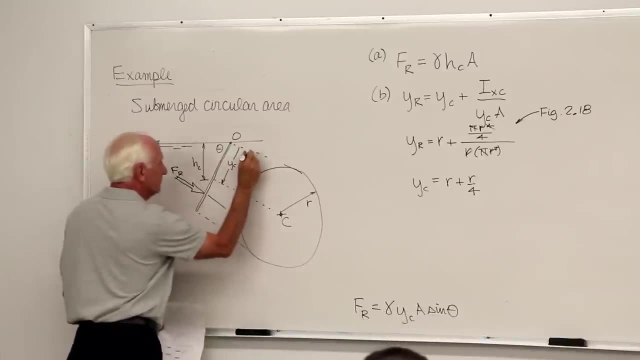 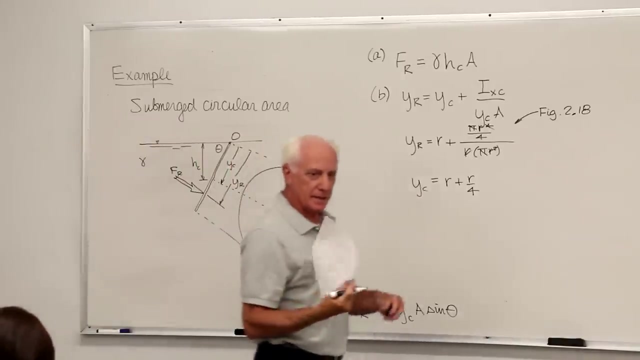 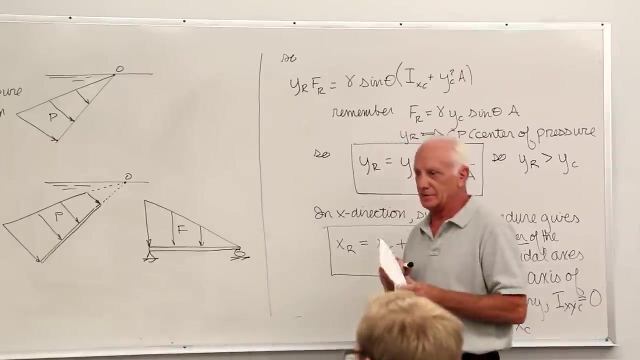 R over four. So the resultant force acts right here: F sub R, Y sub R. So that's what somebody could ask you. Number one: what is the force on the surface? Number two: where does this force act on the surface? 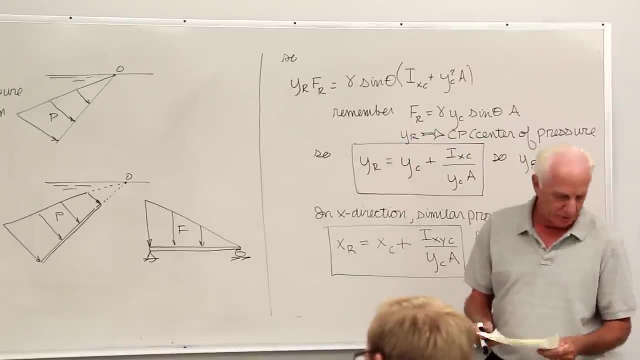 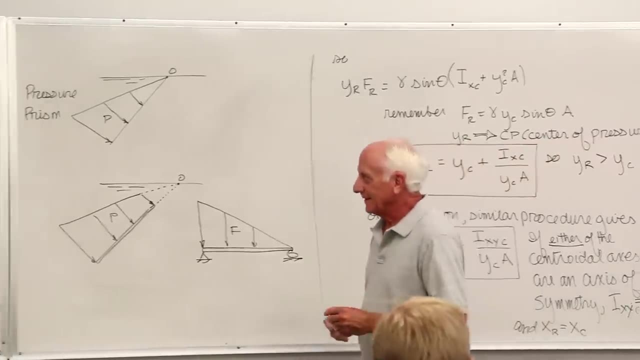 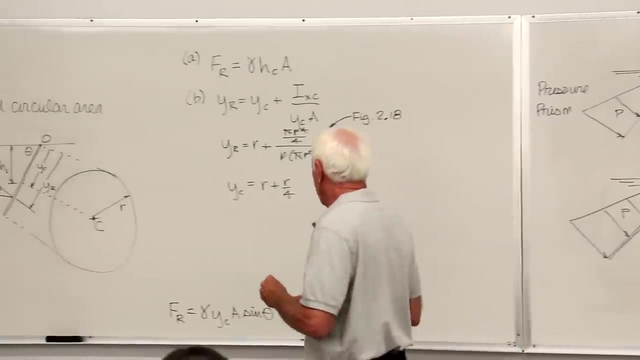 And of course you know that it's perpendicular or normal to the surface. Okay, It could be triangle. Yes, sir, Yeah, Did you write Y sub R? Where is it again? I'm sorry You lost my question, This one. 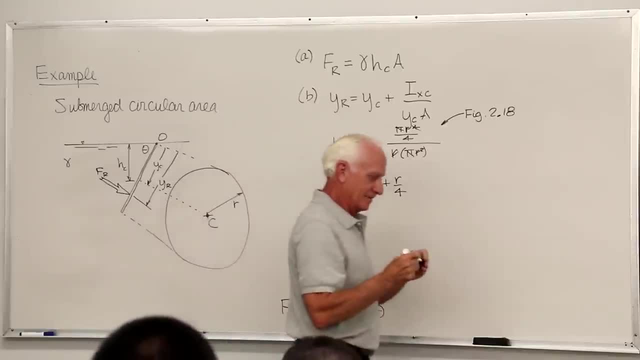 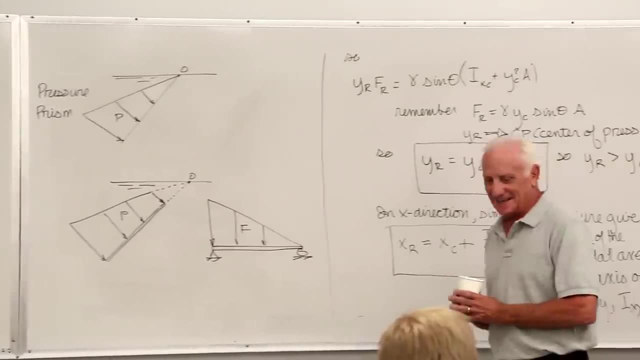 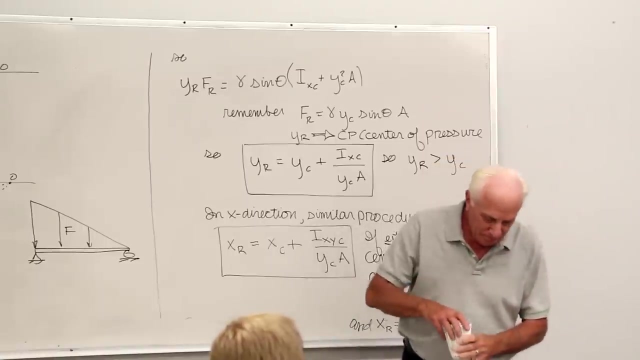 Yeah, Oh, thanks, Sure, Thanks so much. Good, Okay Now. Now that is a circular area. Okay, Now we're going to take a rectangular area, So let's look at that. I think I'll start that over here. 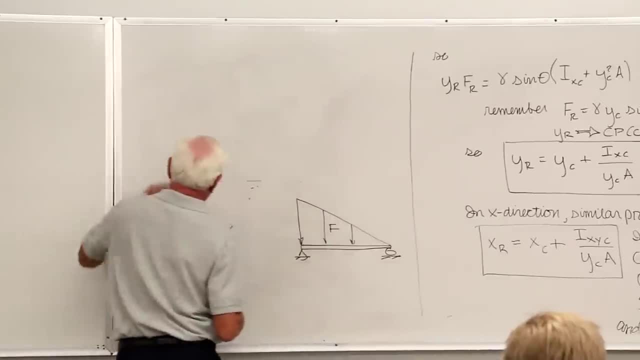 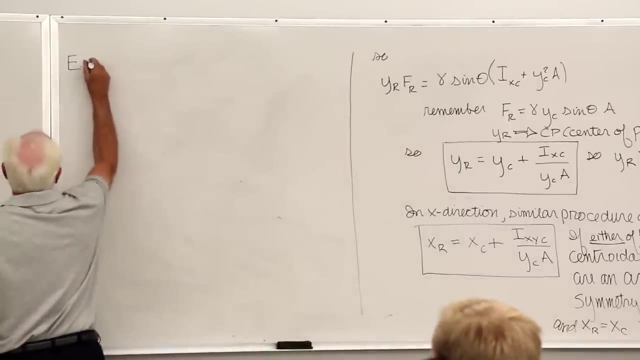 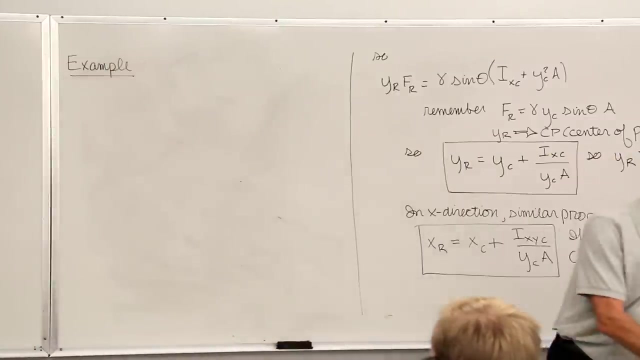 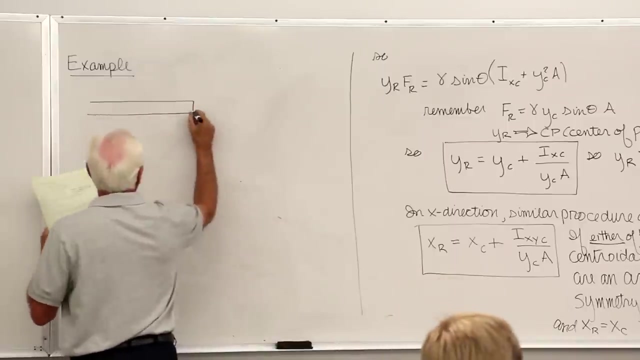 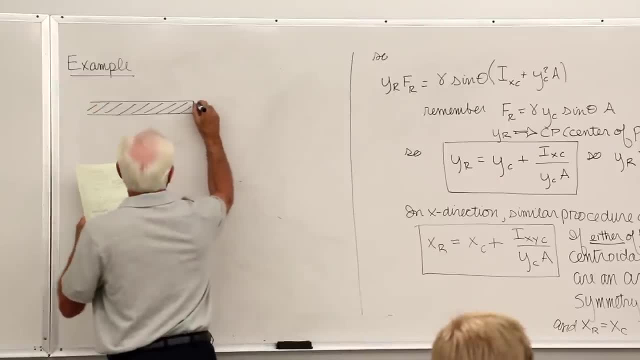 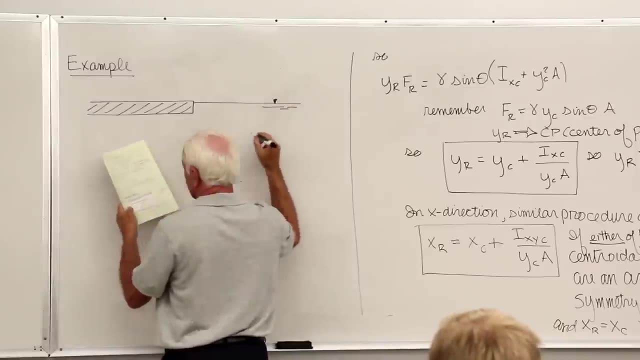 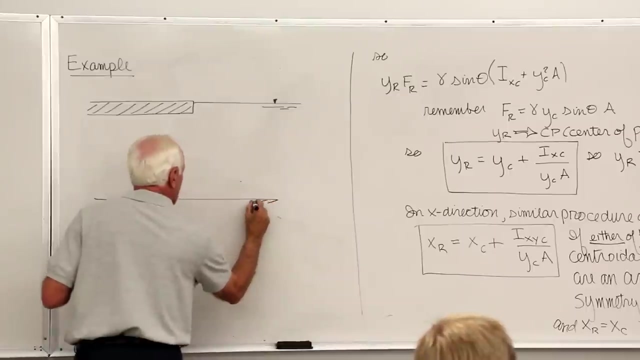 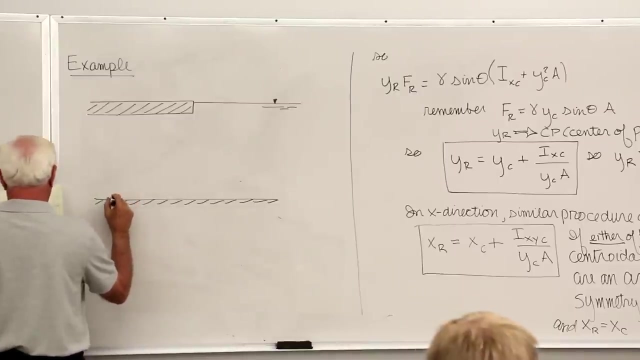 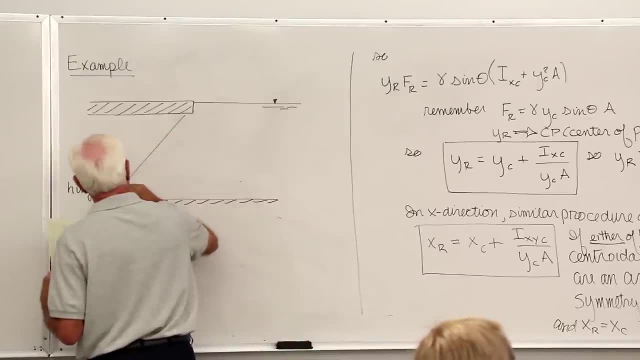 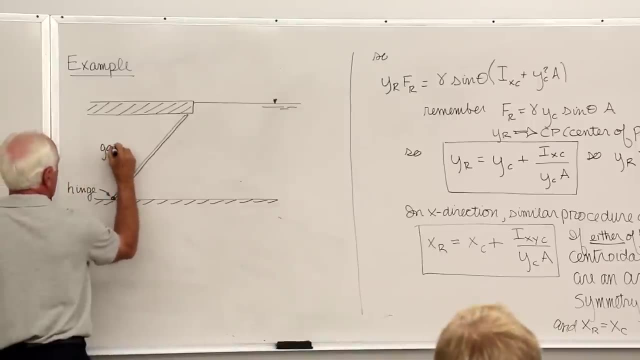 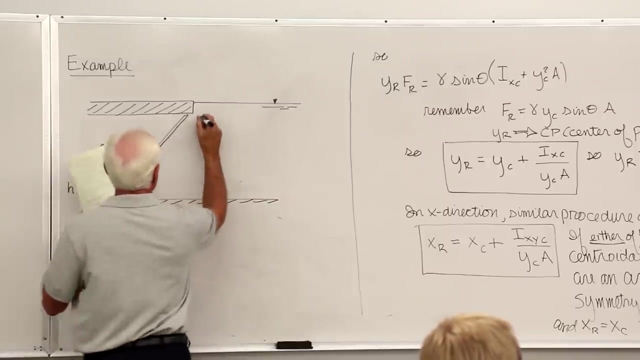 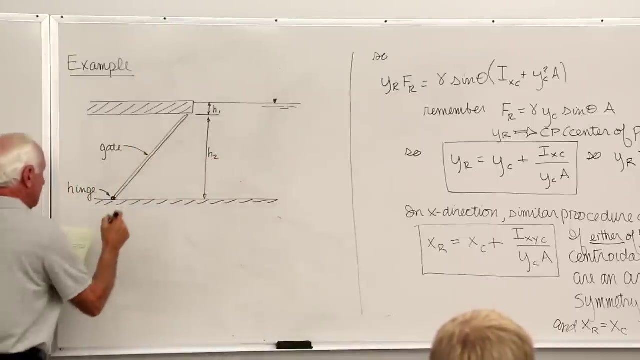 There's a gate right here And we're given the following: distance from here to here is called H1, and the distance from here to the bottom is called H2.. Okay, This is the angle theta. So for this problem, theta is 45 degrees. 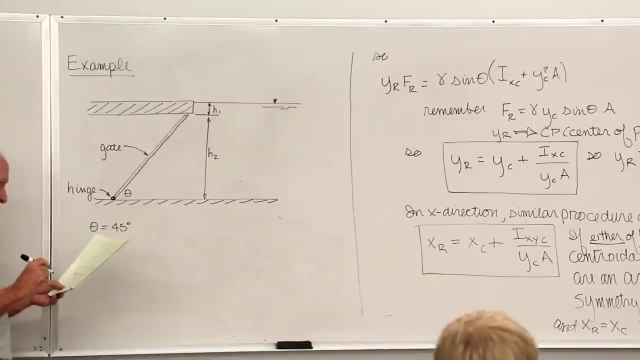 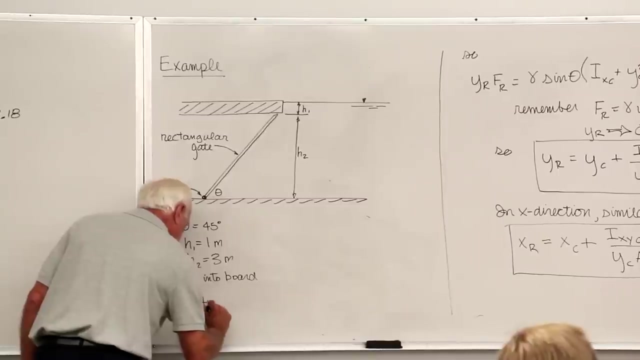 H1 is one meter, H2 is three meters Is one meter, One meter into the board. So we'll put it down rectangular Gabe, just so we know it's rectangular shape. One meter into the board. Gate weighs 90,- yeah, kilograms. weight of the gate. 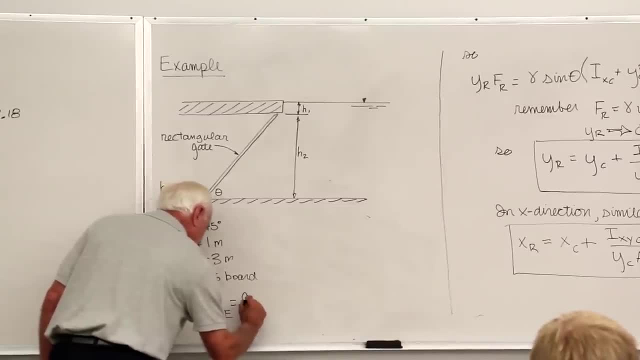 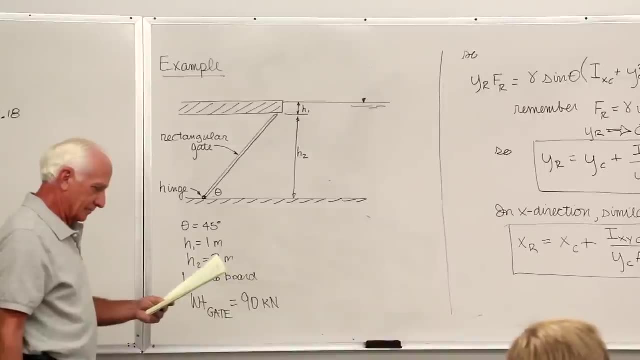 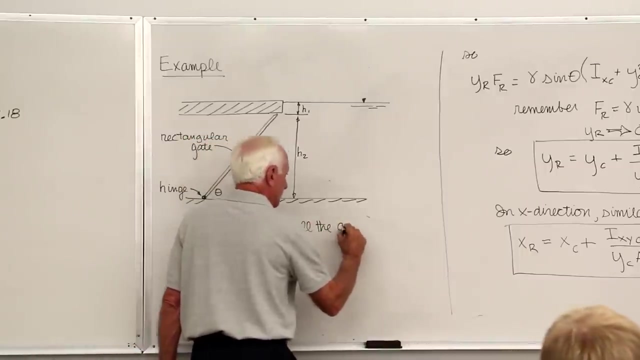 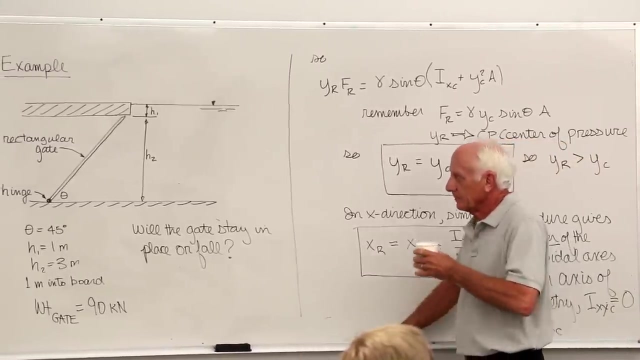 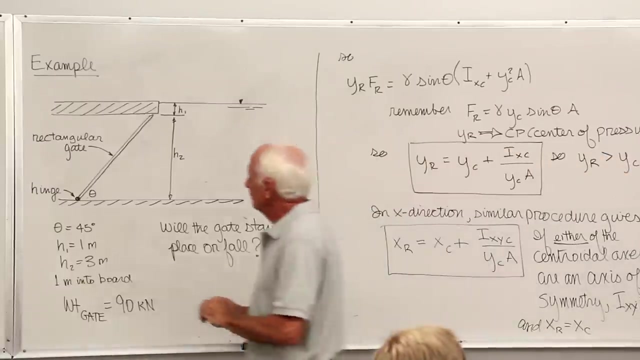 Okay, Okay, Okay, Okay, Okay powerful. Will the gate stay in place Or fall? Okay, we're gonna sign the door on the table. Okay, Okay, Okay, Okay, Okay, Okay. On the other side of the gate is the atmosphere here. 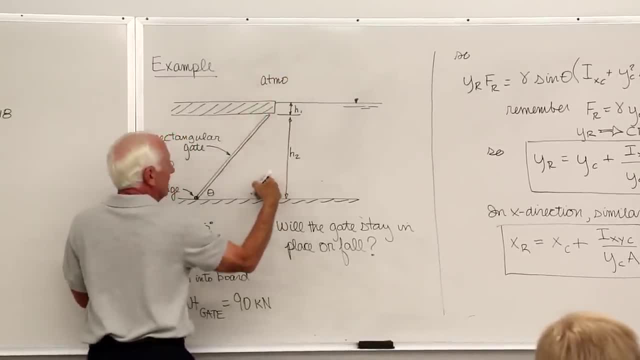 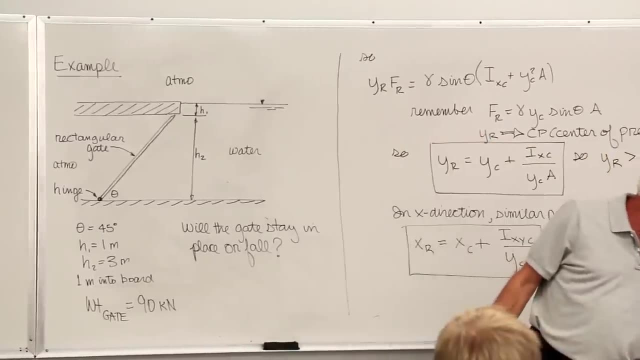 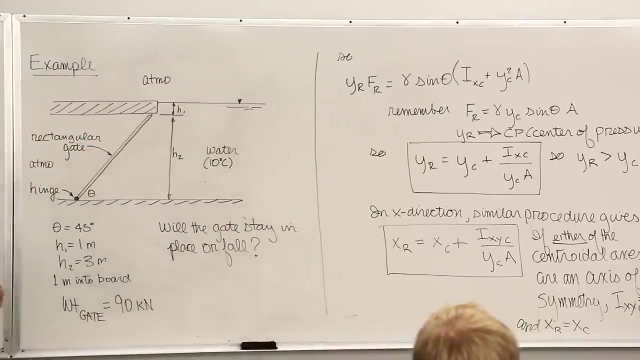 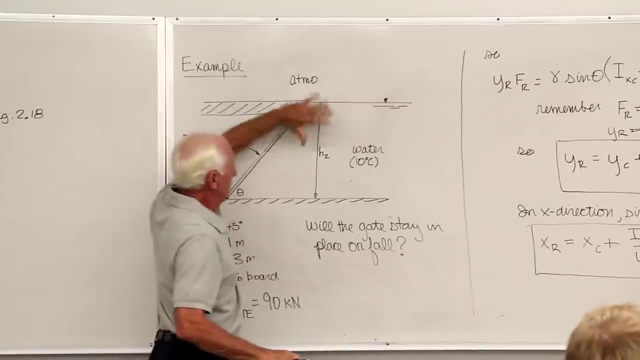 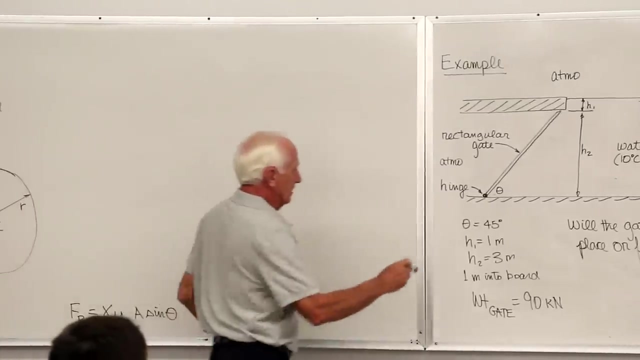 Up here, atmosphere, Right here, water Here, 10 degrees C. Okay, so air on this side, air up here, water there. The weight of the gate itself about the hinge point. here's the hinge point, the way the. 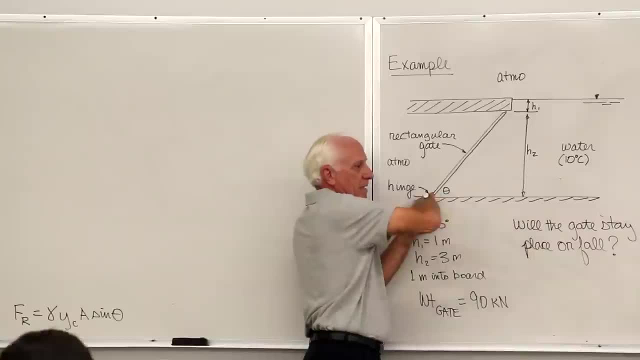 gate's acting this way, the moment's going to be clockwise, clockwise, clockwise, clockwise, clockwise. the pressure of the water is the pen. It creates a force. That force tends to cause a moment which is counterclockwise. The question is which one wins, clockwise or counterclockwise. 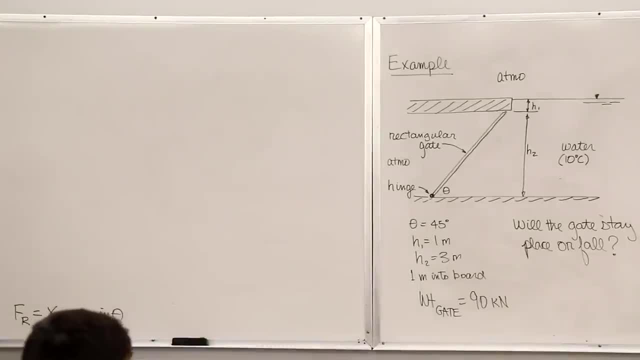 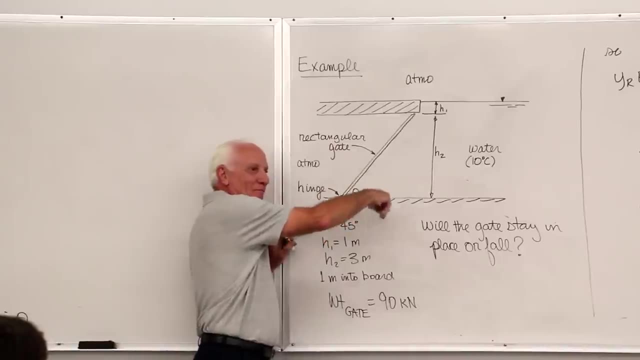 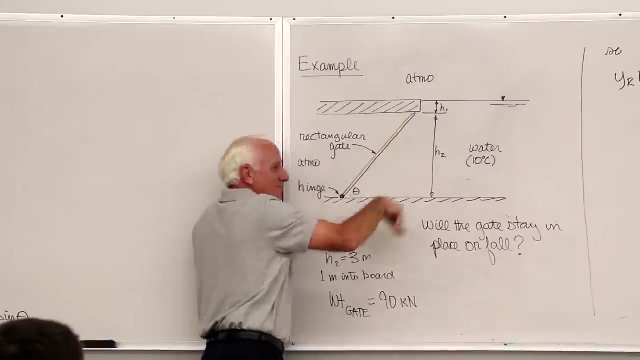 Okay, take a short 15-second break while Matt is talking. Okay, If the counterclockwise moment's bigger, counterclockwise, If the gate's jammed up on the stop, what's happening? If the clockwise moment's greater, the gate falls down. the water comes rushing through. 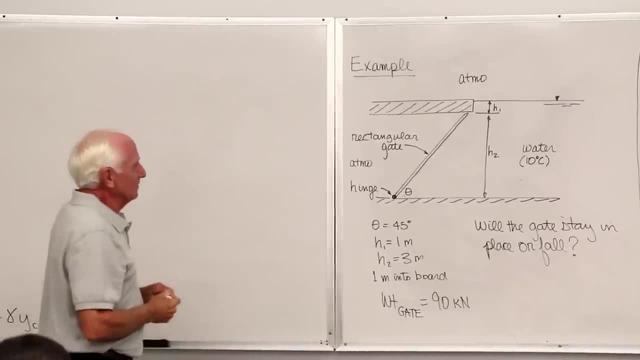 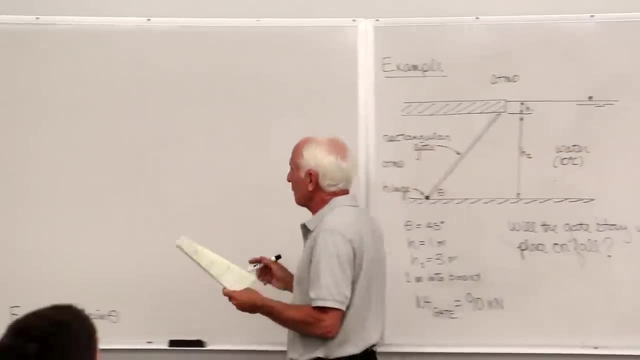 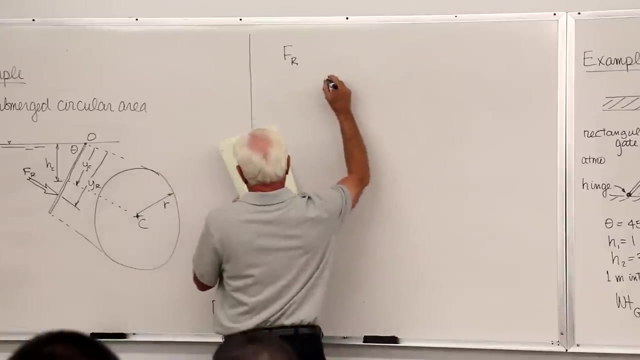 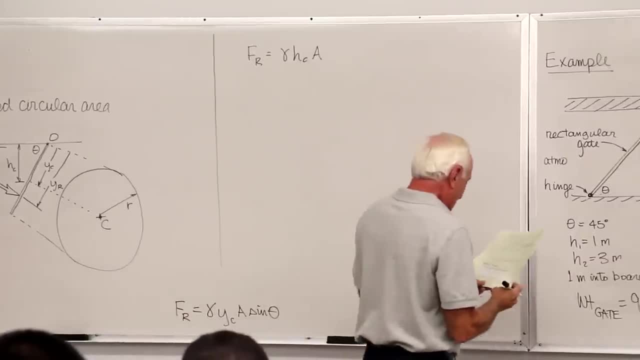 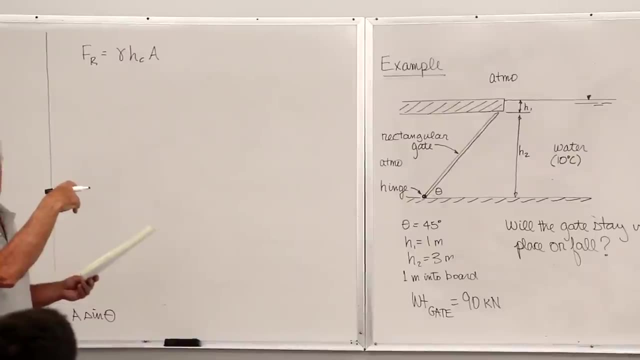 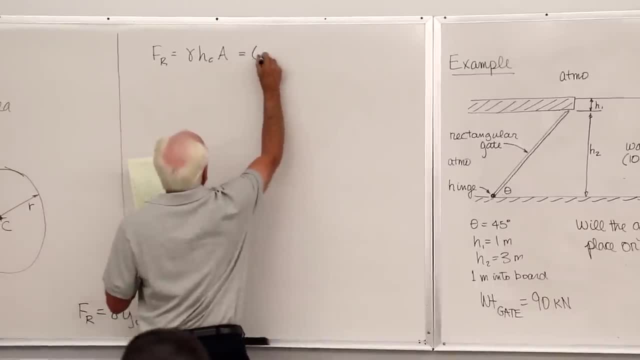 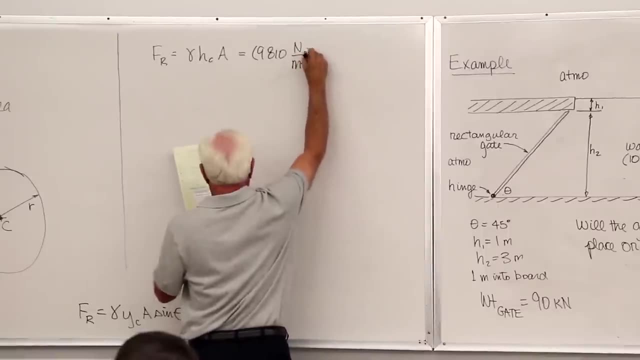 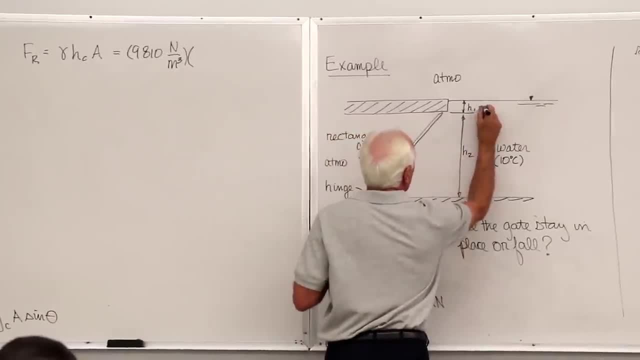 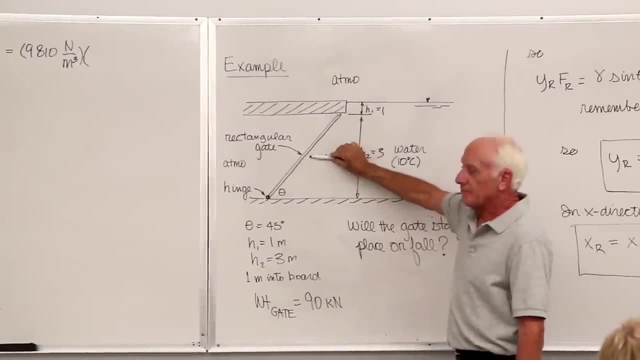 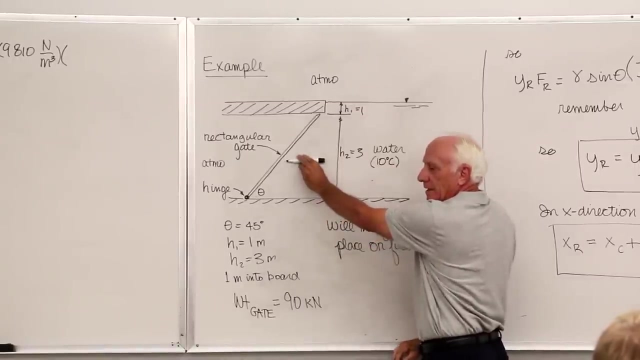 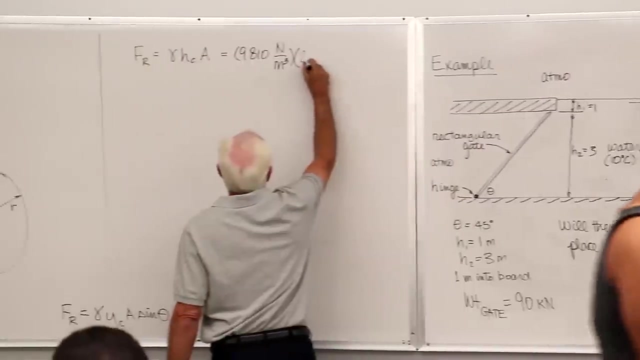 The distance down to the centroid, H1 is 1,, H2 is 3.. Where's the centroid Right, in the exact center? 1 plus half of 3.. H sub C: 1 plus one and a half. two and a half. 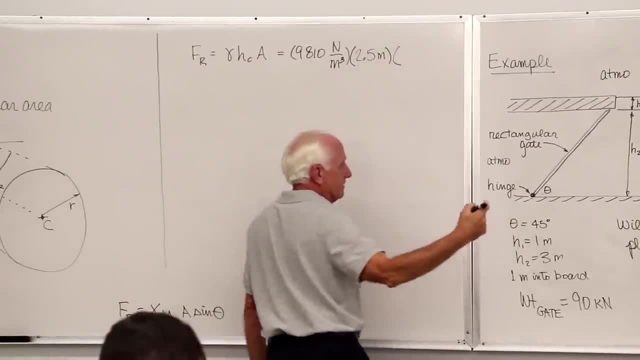 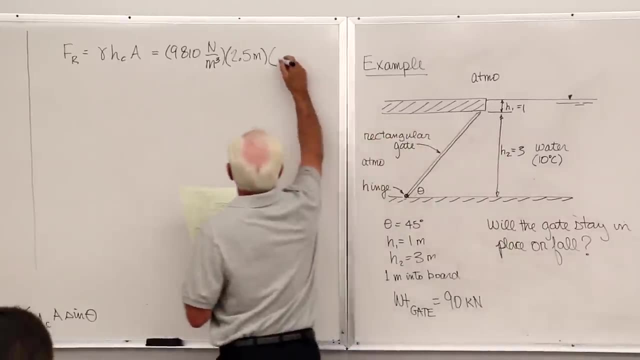 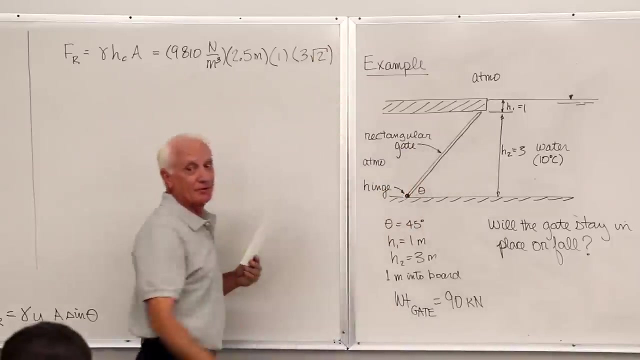 Area of the gate 1 into the paper, Hypotenuse 3 times square root 2. It's 45 degree, luckily, so that's fine, Okay. the resultant force due to the water: 104,051 newtons. 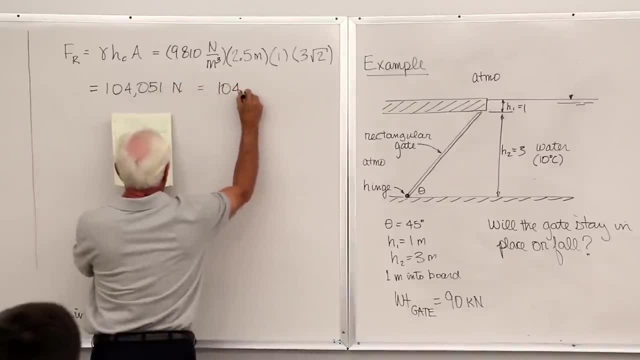 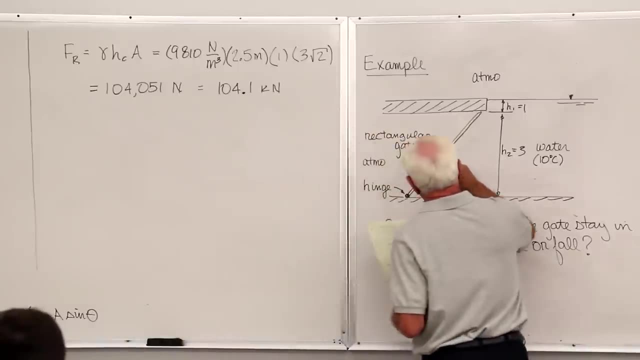 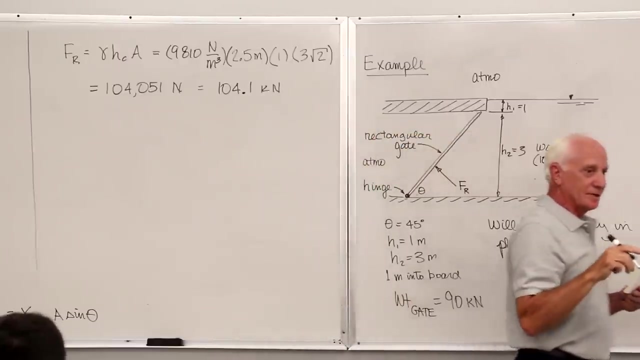 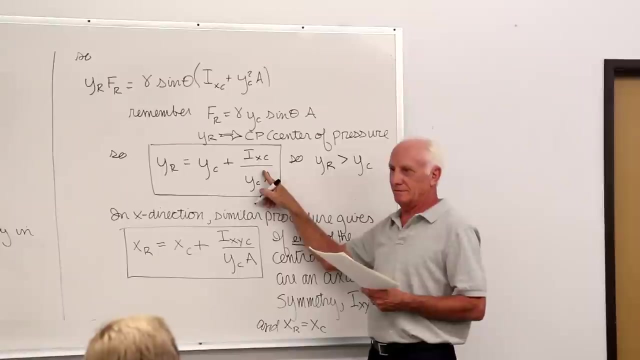 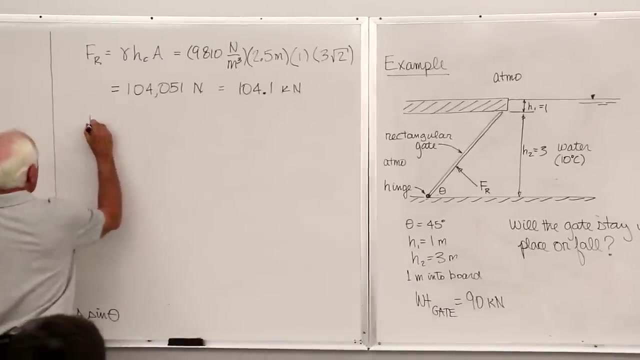 104.1 kilonewtons. Okay, and of course that force is acting up here, Not through the centroid. Through the centroid plus a little bit. How much little bit? My computer tip is Okay, so let's have a look here. Okay, so you start on a small formula here: Y sub R Y. 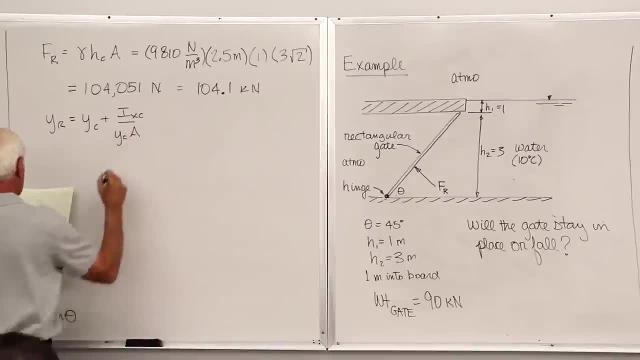 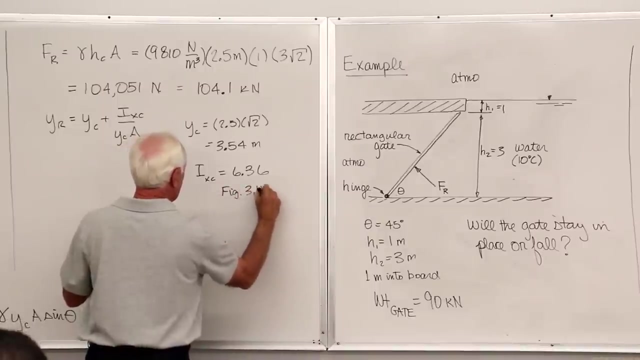 sub C. I sub X C, Y sub C A. Okay, Let's get down the Y sub C, Okay, Okay, Okay, Okay, Okay, Okay, It's a 45 degree triangle. square root of 2, hypotenuse i sub xc equals 6.36, figure 318, figure yes, 218.. 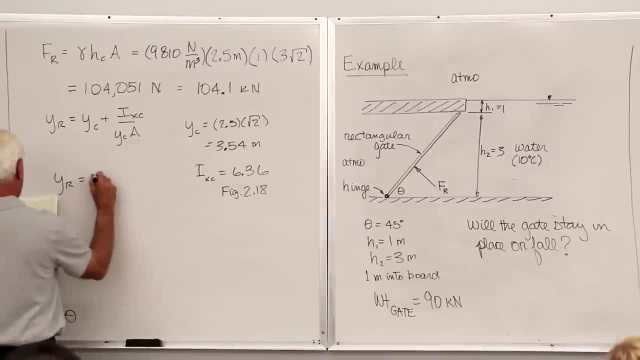 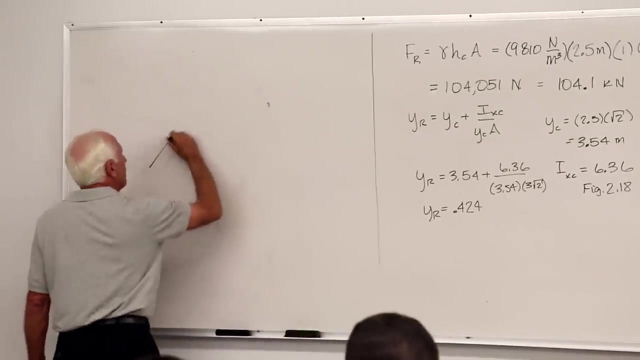 So y sub r, 0.424.. 0.424.. Okay, Okay, Okay, Let's make a diagram of this thing now, with the forces on it, The weight acts vertically down. So here's the gate. The weight acts vertically down through the centroid. 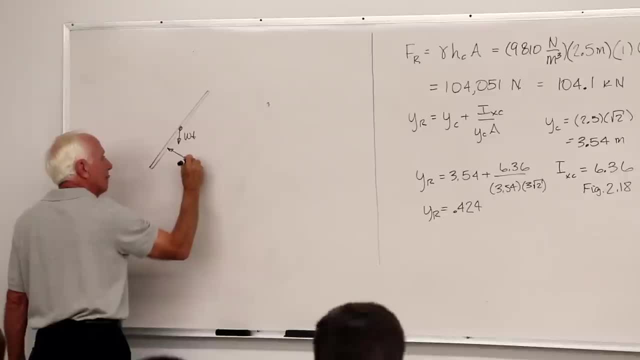 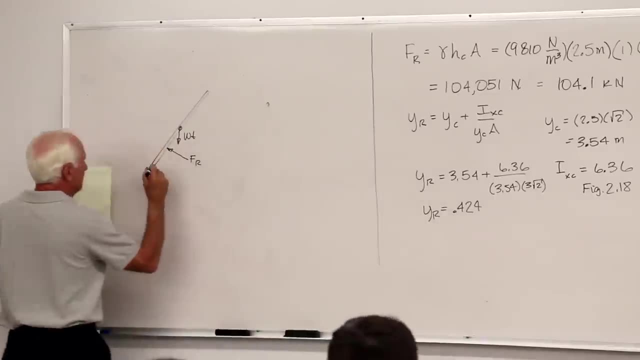 The resultant force acts this way. Okay, So this distance, here's the hinge point. So the distance the weight acts over here, 1.5 meters, And then our f? sub r- you can hear it in here. you have to subtract. 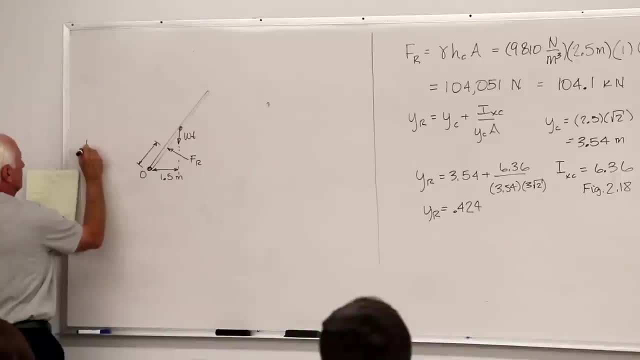 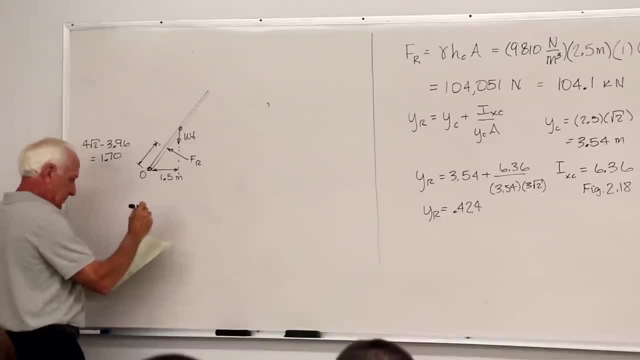 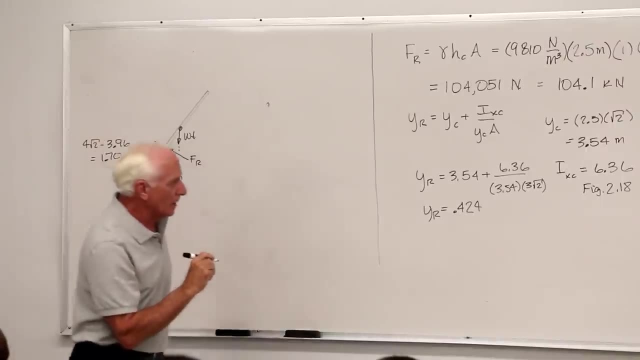 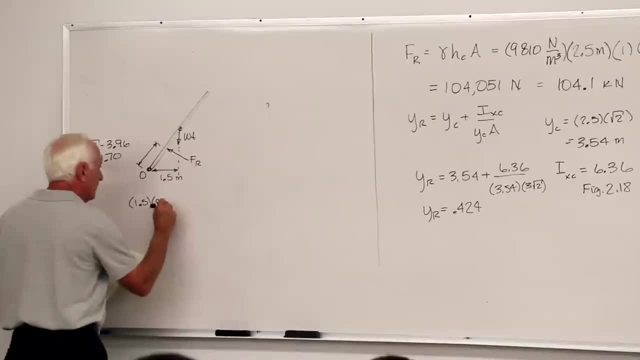 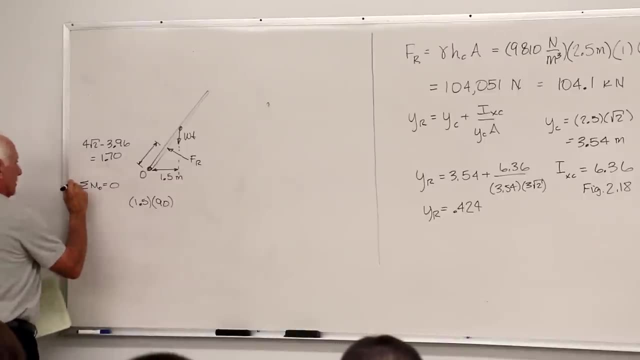 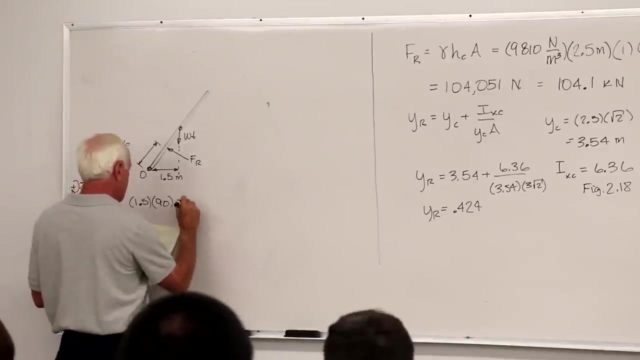 Ninety kiloliters, Some moments about. .0 equals 0.. Let's call it clockwise positive, Okay, Minus f sub r times that distance 1.10.. Minus f sub r times that distance 1.99.. 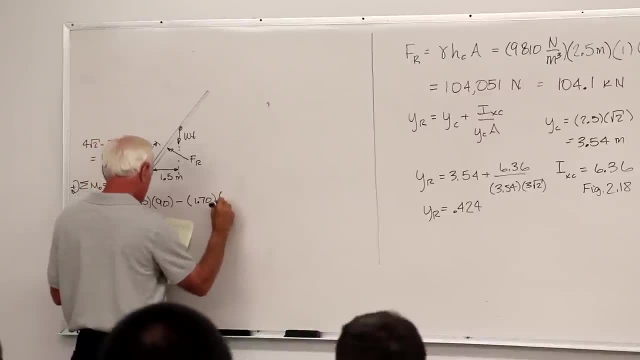 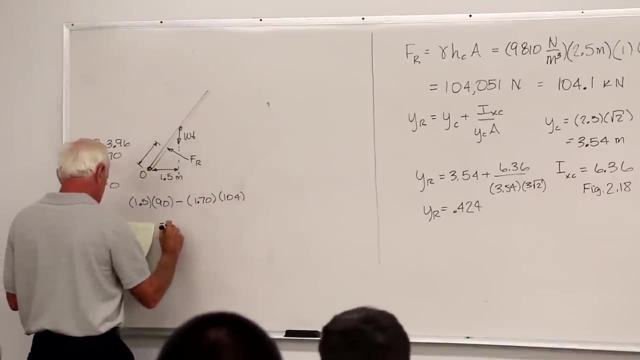 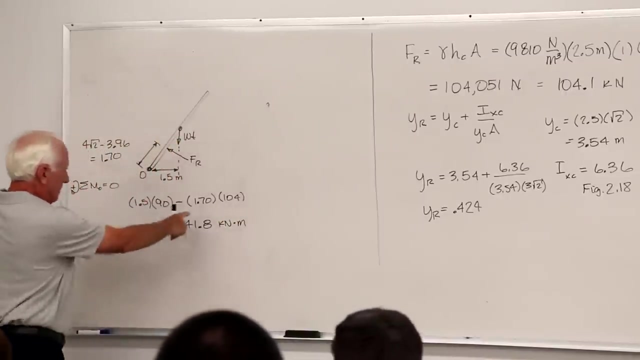 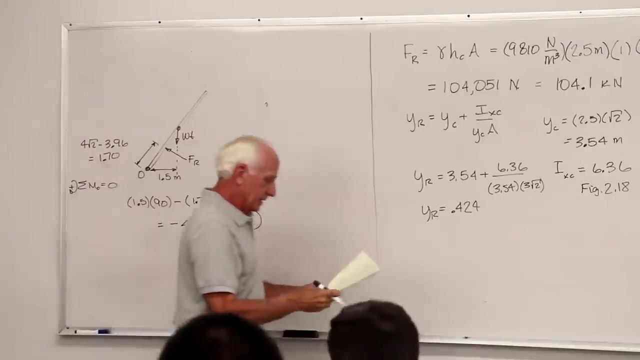 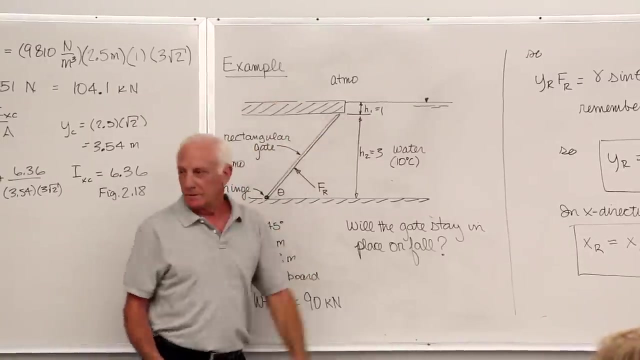 point seven and I get minus forty one point eight and that's kilonewton meters. minus means counterclockwise, so it's going to go this way. I don't want to push the gates up, jamming against that. top horizontal surface stays in place. 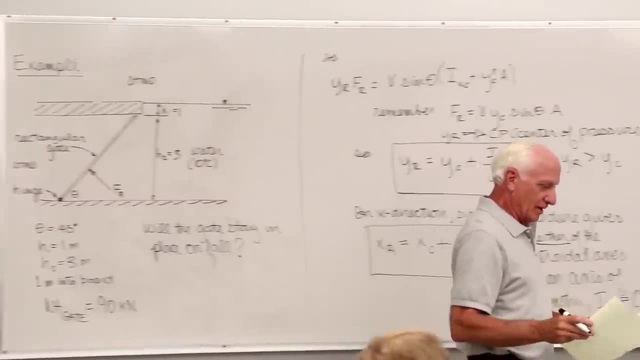 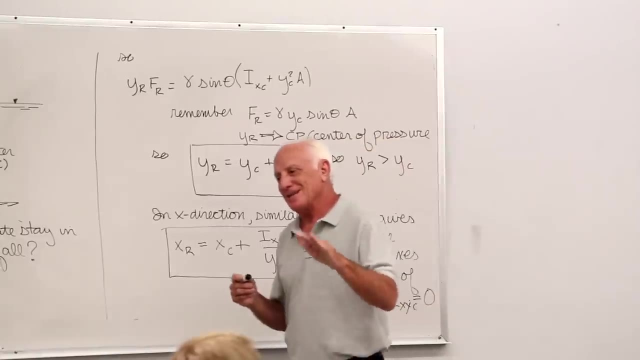 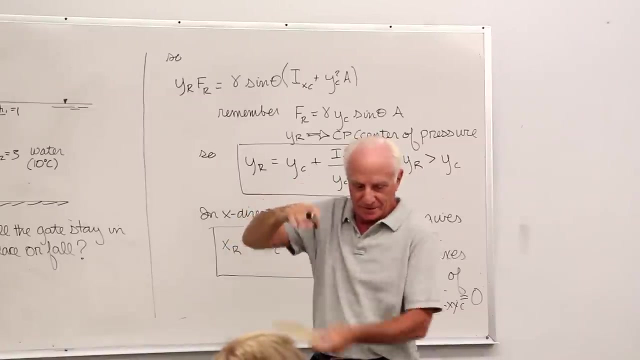 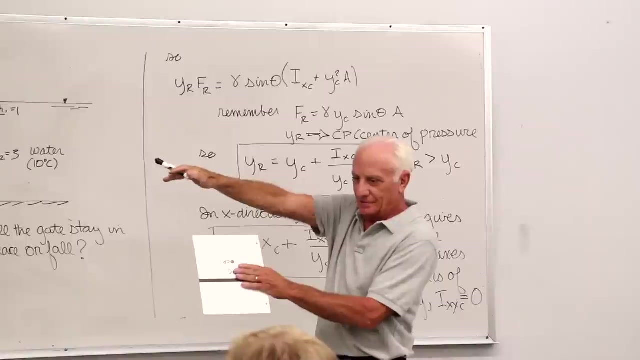 okay, so that now we've worked one which was a circular area. we worked on the circular area. the top of the circle touched the top of the water free surface, the rectangular one. the rectangular surface was below the top of the water. so I'm trying to show you what we do in different cases like that. okay, 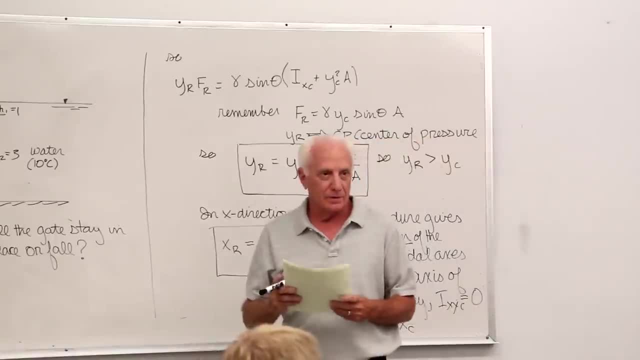 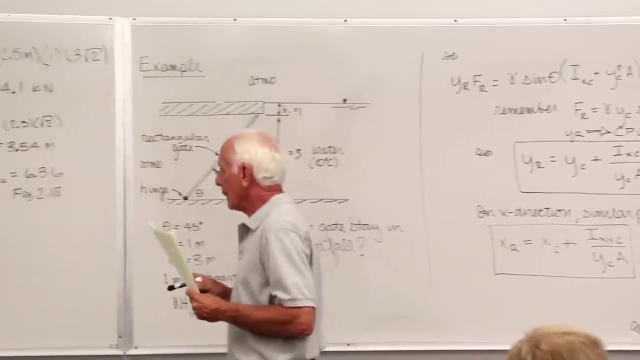 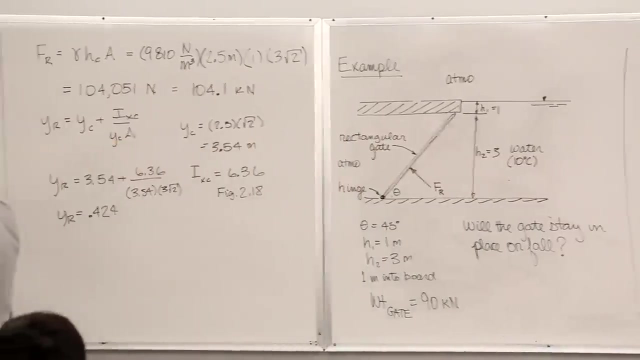 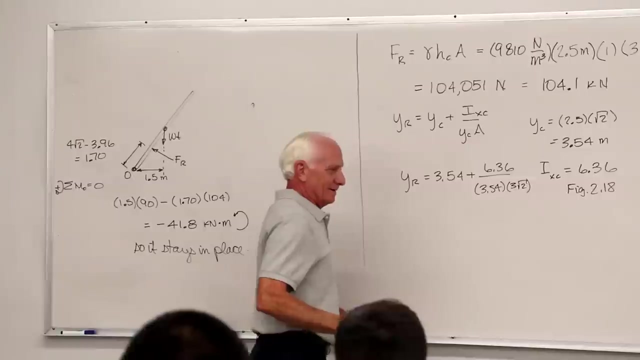 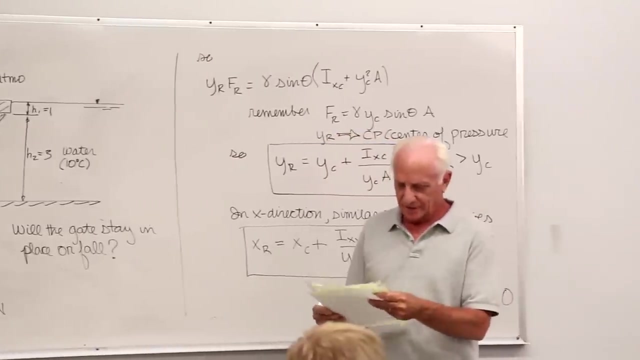 now we have all right. oh, yeah, should be. and why is that? yeah, it is, it is that's just a value. yeah, it's over here. yeah, right here. yeah, yeah, it's this, here's why Samara up here. okay, yeah, thanks you. that was just a value of the 6.36 over three points. 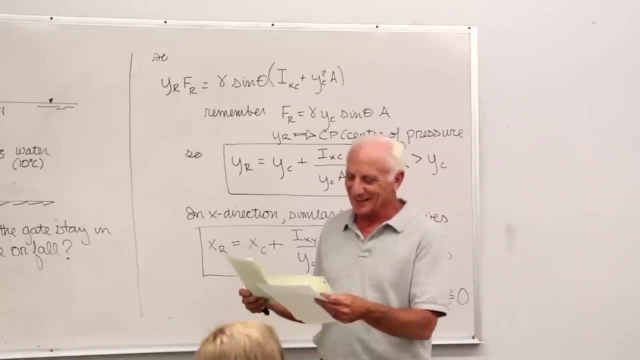 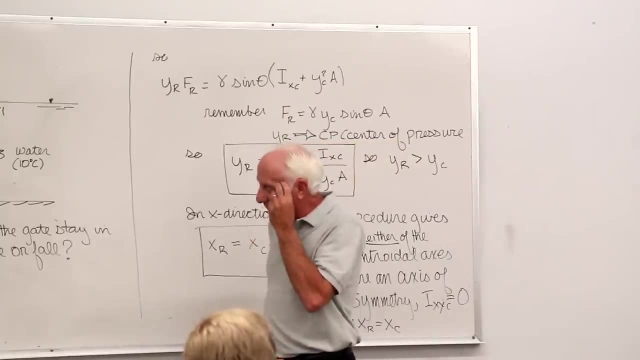 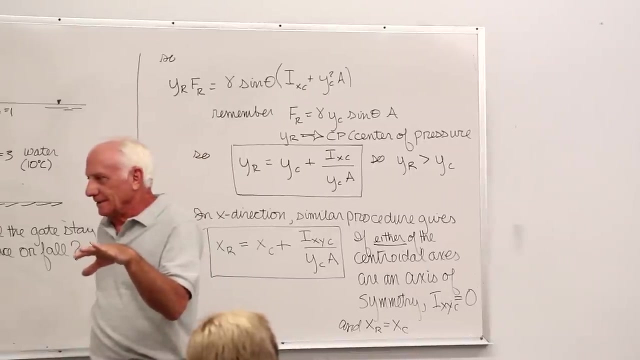 that's what it was. yeah, it was, it was. yeah, it was okay. now I've got one more to work, but I'm gonna wait and work down next time, so I want to go over a homework right now. pass court back. did it get over there to you guys over there? okay, if anybody? 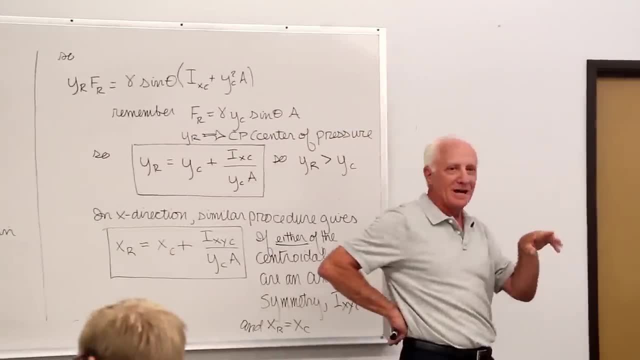 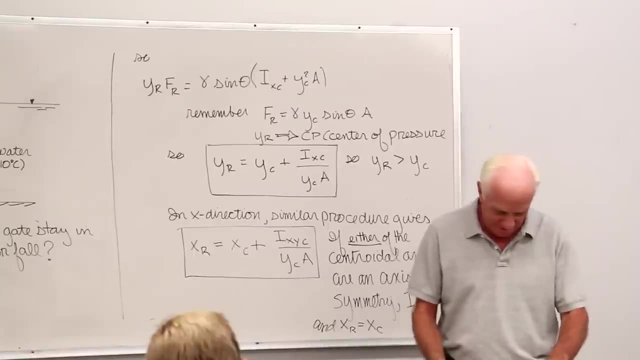 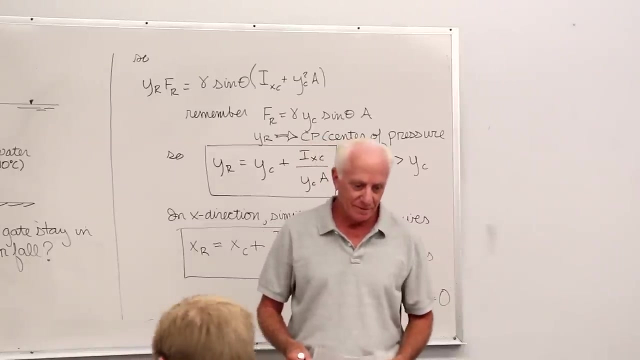 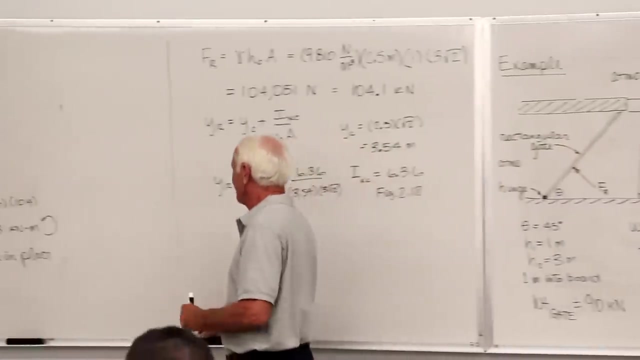 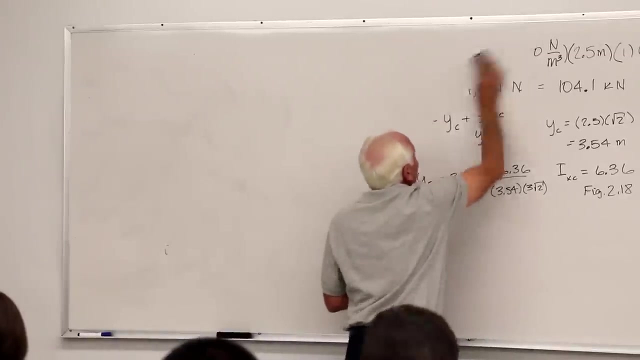 missed it? there's anything left over there? no, okay, everybody gets their homework. okay, so let's talk briefly about home. oh yeah, that's fine. no, I'm sorry, you won't need to, I'm gonna. I'm gonna mention things that are not problems. okay, these? 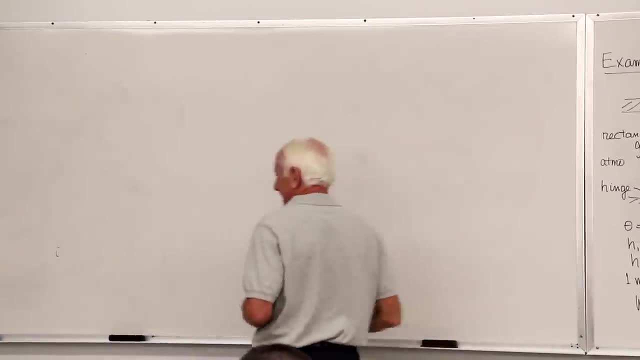 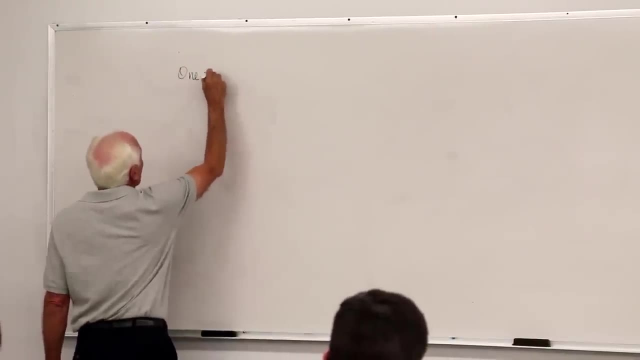 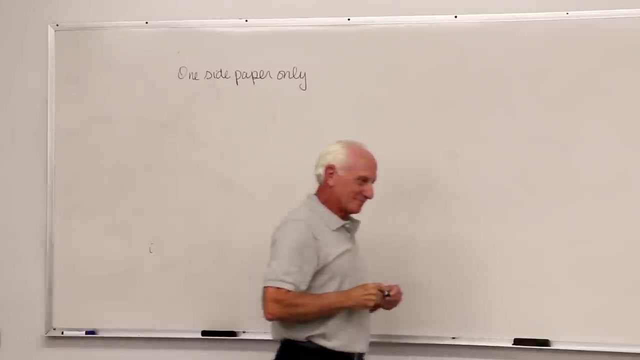 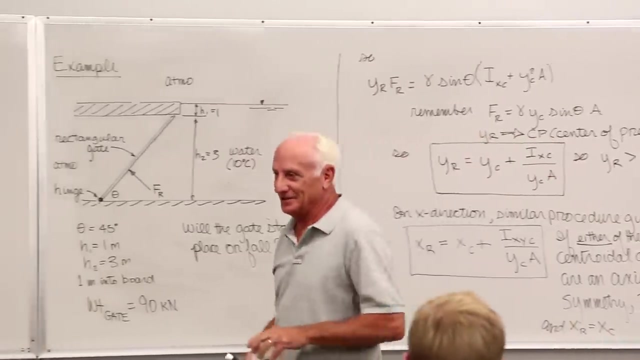 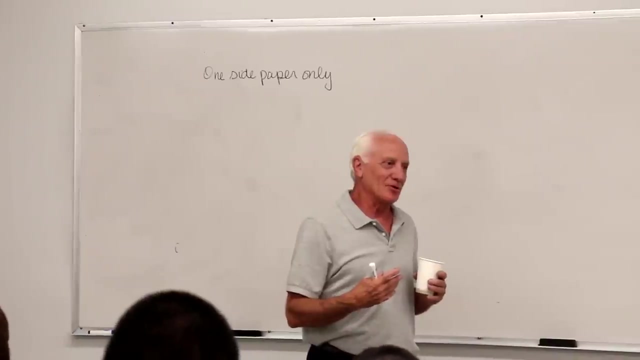 are things that helped me when I'm rating your homework. number one: use one side. 65 people times like five pages. you know 300 pages I'm going through. sometimes, if I'm going through a fast, I won't look at the back side because I'm just flipping pages and I 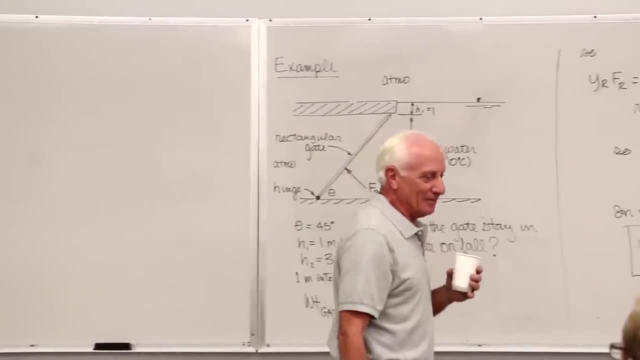 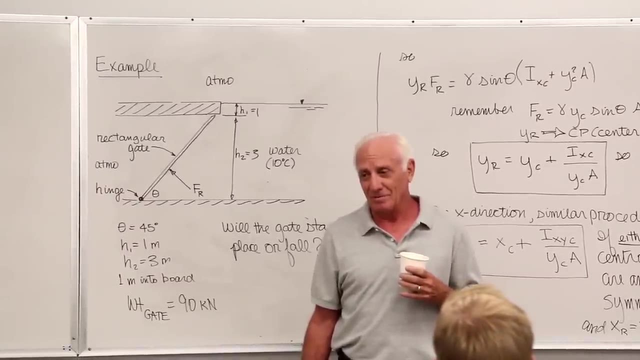 end up missing what's on the back side. so it really helps me if you put all the problems on one side on exam. it's absolutely critical if you use your own paper never on exam, push up on the back side because it's too late if you come. 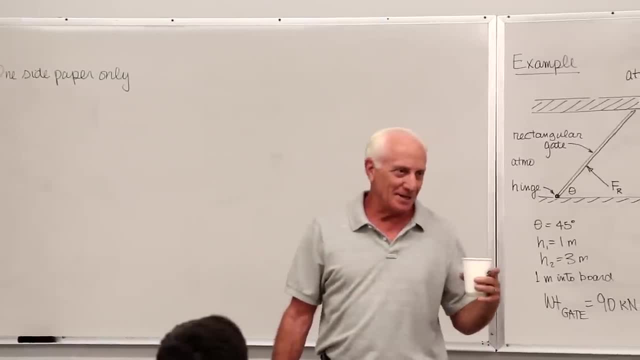 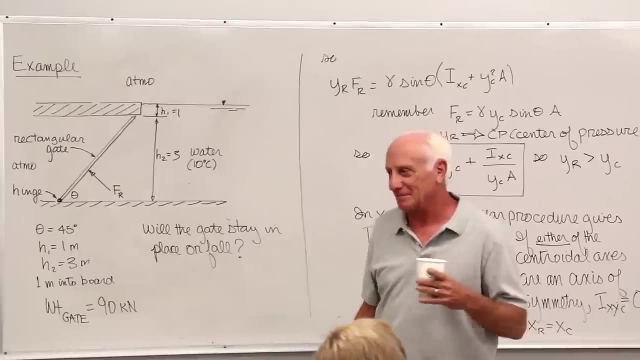 back. the instructor said: well, Professor Biddle, you missed the back of my page. I did that problem, the back side of the page. I'll say, are you sure? so never use the back side of the page, especially on exam. it's really can get you in deep trouble, obviously everybody. 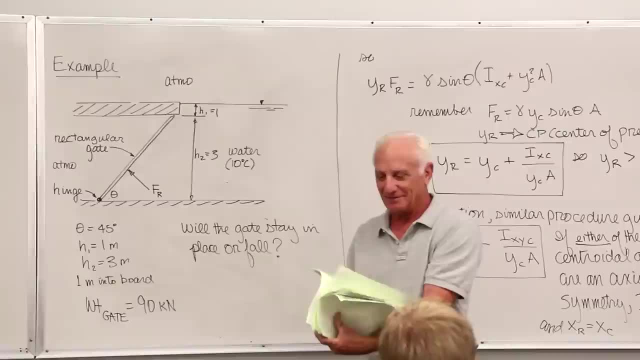 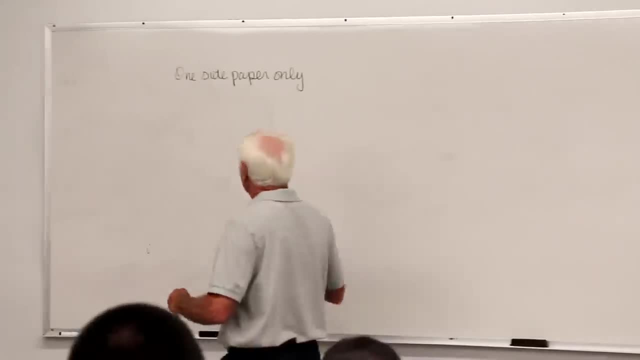 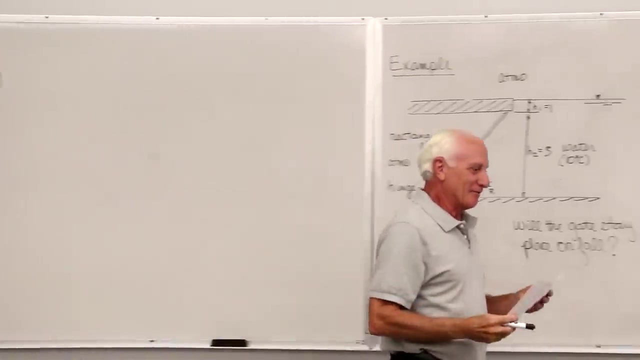 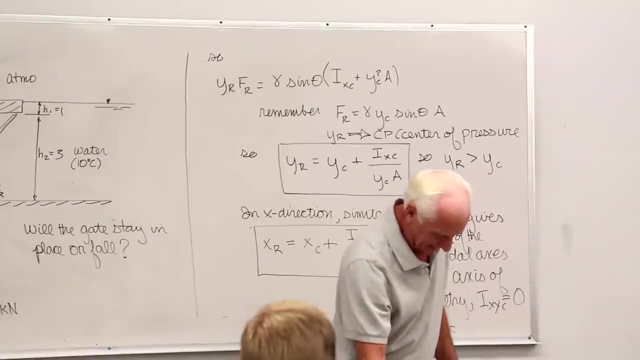 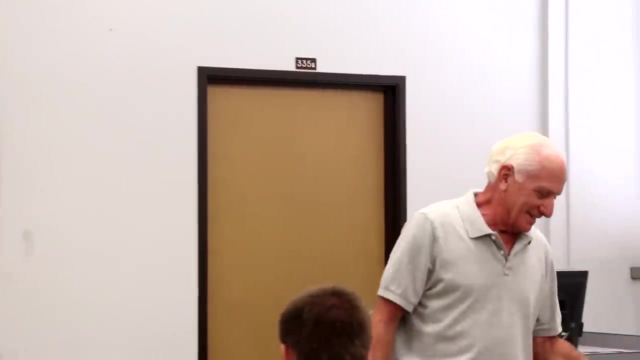 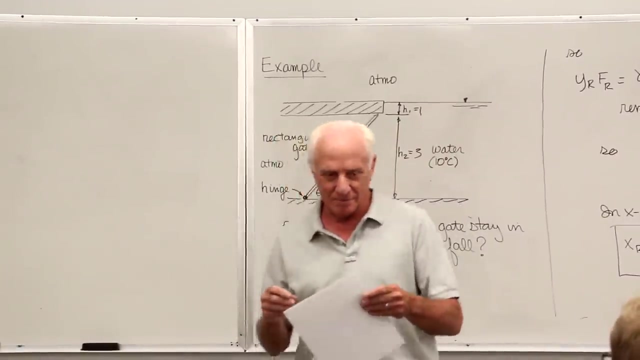 pretty much usually using engineering, green and white line. fantastic, okay, everybody almost stapled it together. we tell our freshmen in the freshman class if you've got some paper, she's just two sheets. what you don't want to do, let's just say: you know, I can't afford that three dollar cup stapler. so what I do is: I've learned. 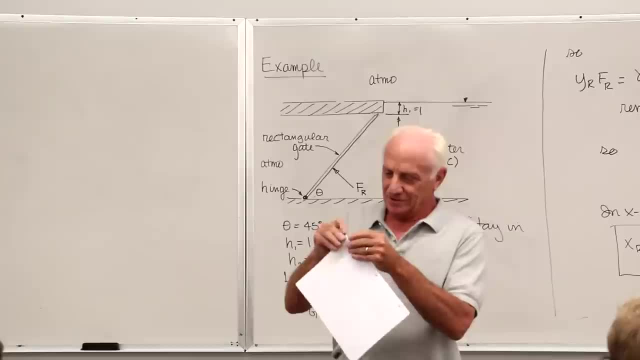 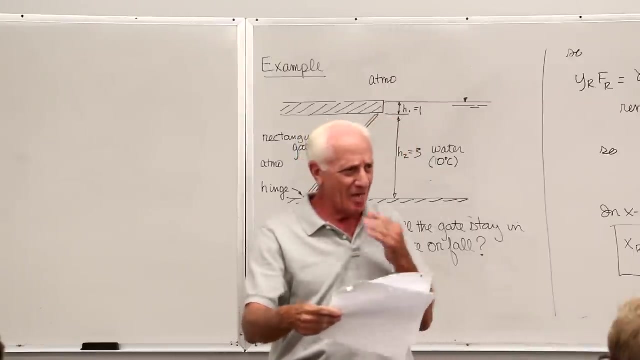 this with my years in junior high did you take this and you fold this three times and then you cut up, like with your fingers- you need scissors please- and you Fold it back like that. Here, Professor Bill, here's my homework. Are you kidding me? 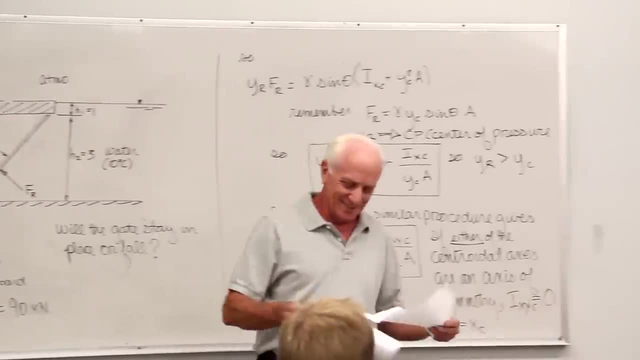 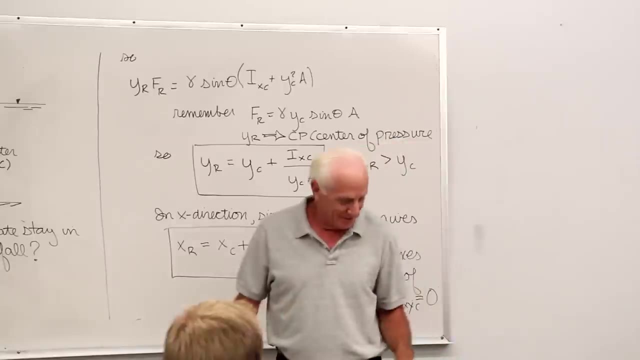 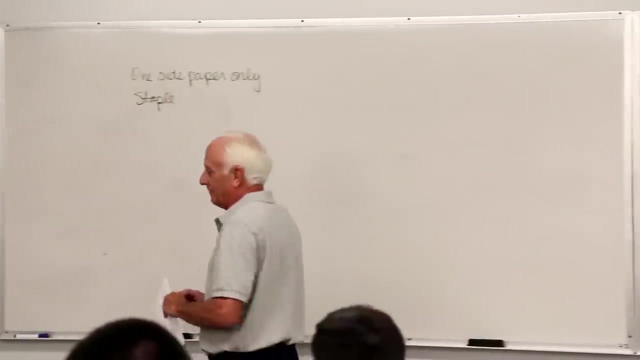 This is engineering. you know This isn't. you know junior high, So don't do stuff like that. Go out and buy a $3 cup stapler for your homework, Okay. you'll notice something that says problem or divider lines. problem, divider lines. 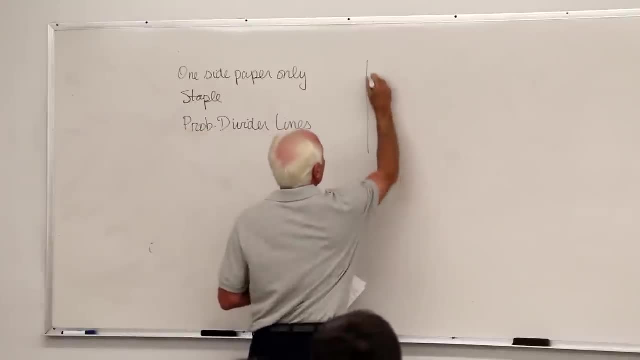 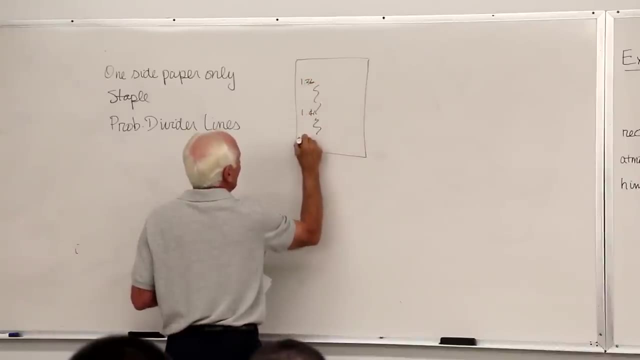 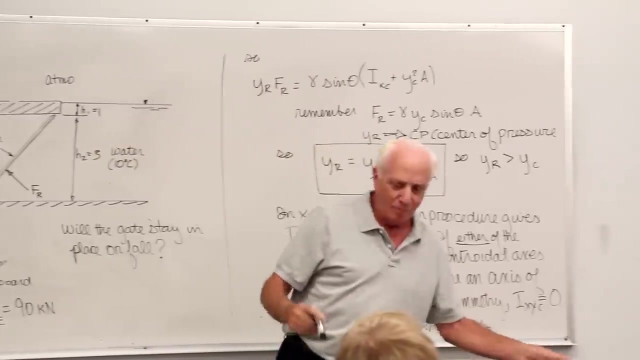 So if I see a homework page that's got from 136 and 141 and all kinds of stuff and 172, sometimes I don't pick up those problem numbers because the whole page is full of calculations with numbers. So in order to make my life, it really helps me. 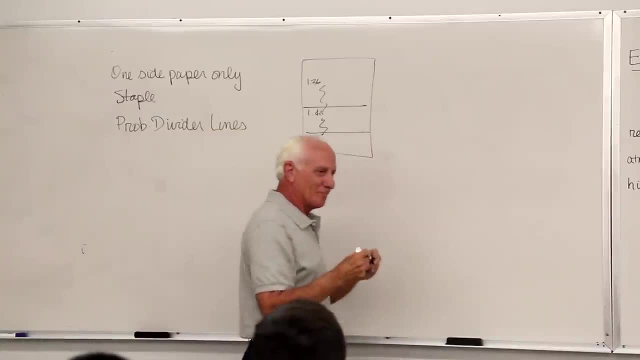 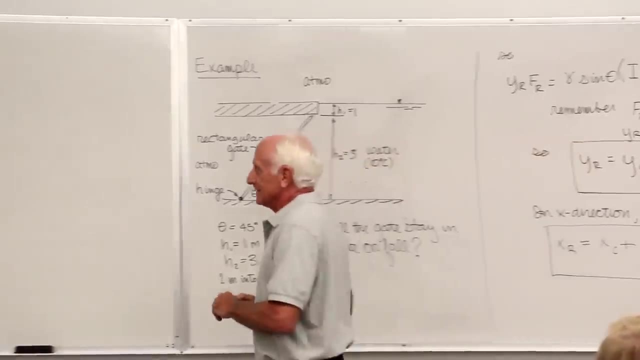 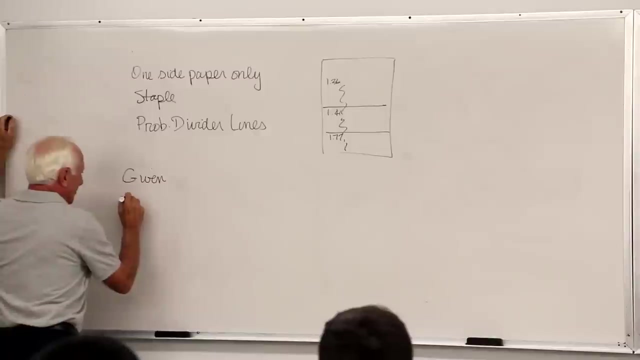 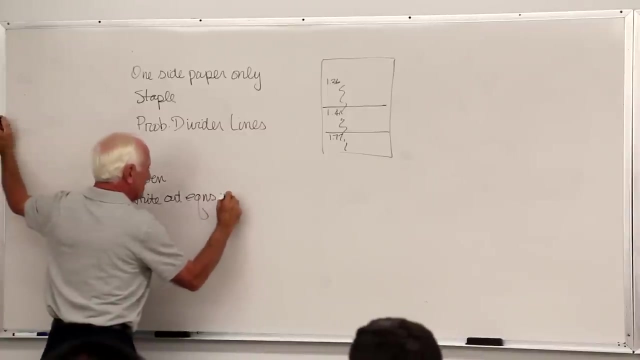 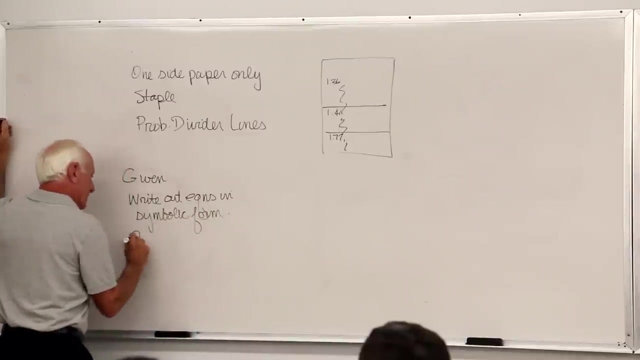 if you just do this, so I know one problem stops and one problem starts. That really helps. So let's call problem divider lines. Okay, most people do this. First of all they put down what's given, then they write out the equations in symbolic form, then put in numbers. 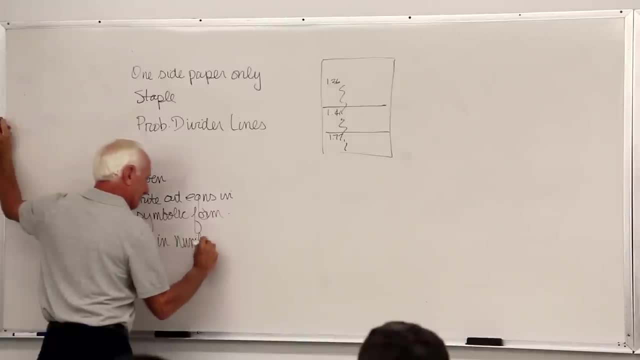 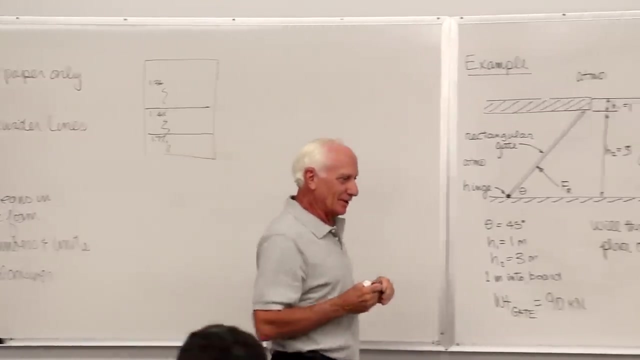 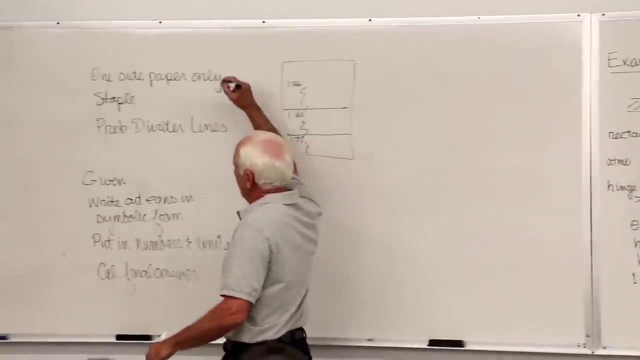 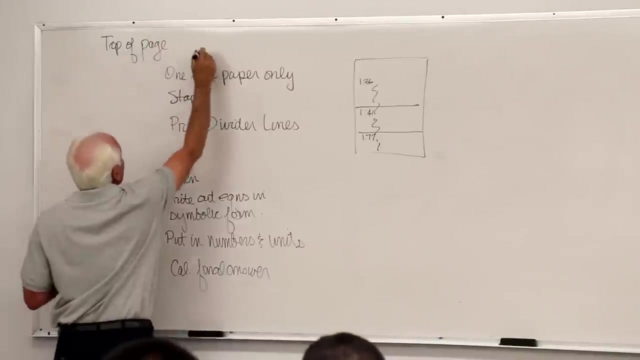 and units And finally calculate the final answer. That really helps me and that helps you On the top of the page. here's the top of the page. It's the top of the page, So I don't care where they are. 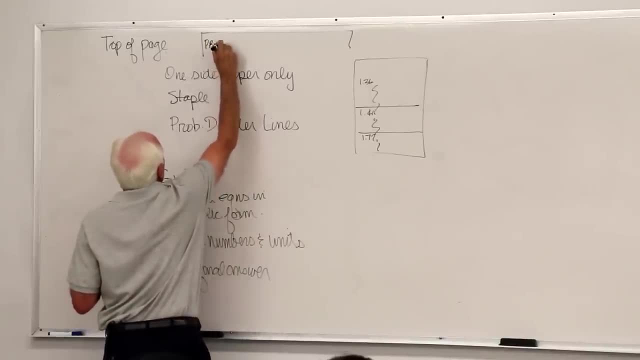 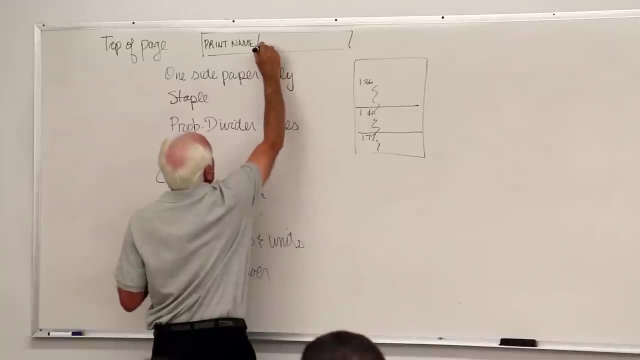 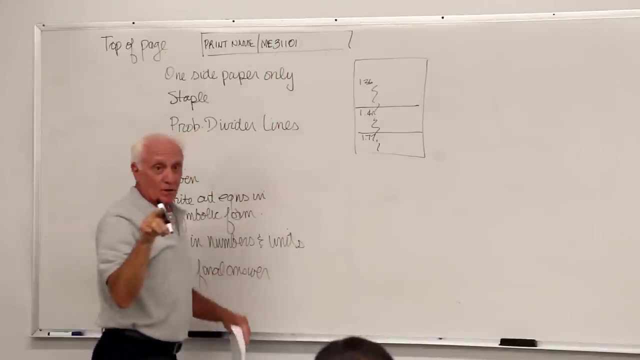 Top of the page is fine. Print your name And then you have ME 100, I mean ME 3,, 11.. Here's section one. Here's section one. okay, So every time, because I've got two sections. 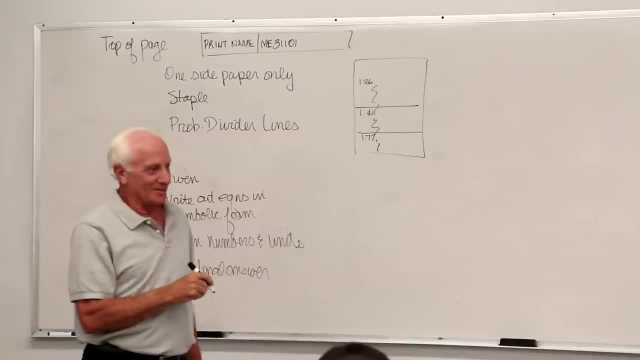 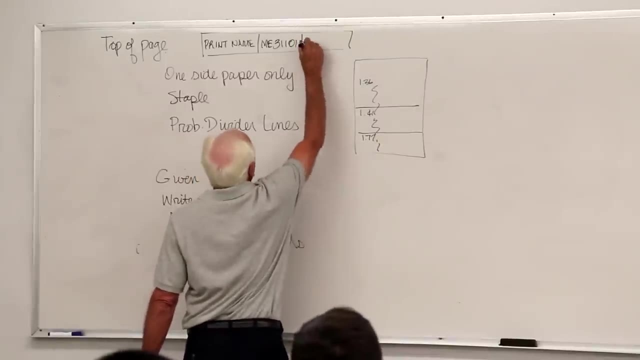 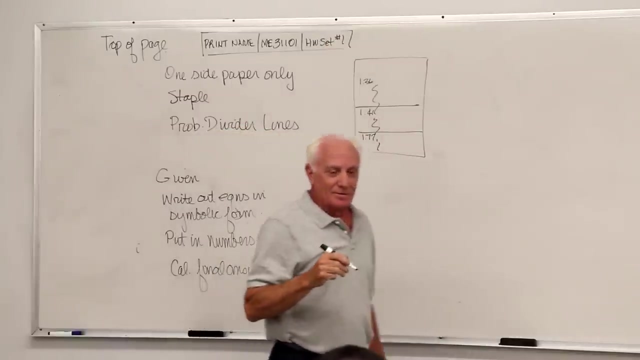 If I drop all the homework I've got to reconstruct. you know It helps me if I have a section number on there, So section 01.. And then homework set number one. It's okay if you want to do homework, set number one. 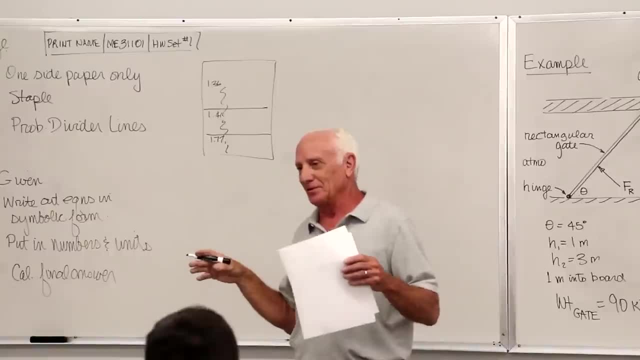 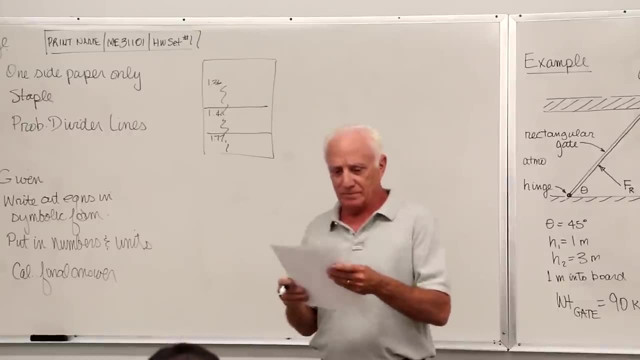 chapter one. fine, Don't just say chapter one, because there's going to be multiple homework sets on some chapters. Chapter five has like three homework sets on it. So if you come to me at the end of the quarter and say, Professor Biddle, are my homework grades right? 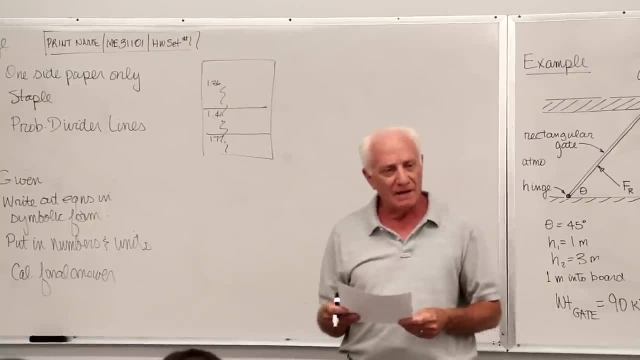 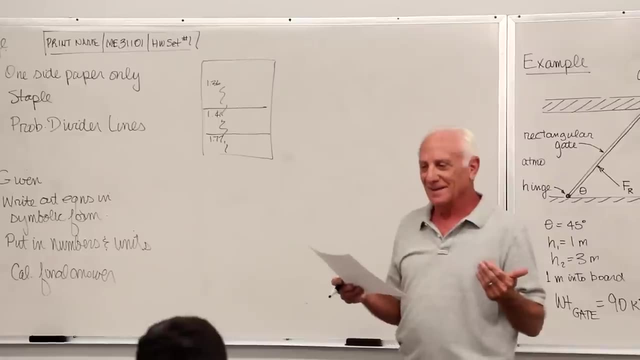 in your grade book And I'll say: well, you're missing set number five. Do you have homework? Do you have it with you? Say, well, I didn't number them that way, I numbered them my problems. No, Help me, help you by putting a homework set number. 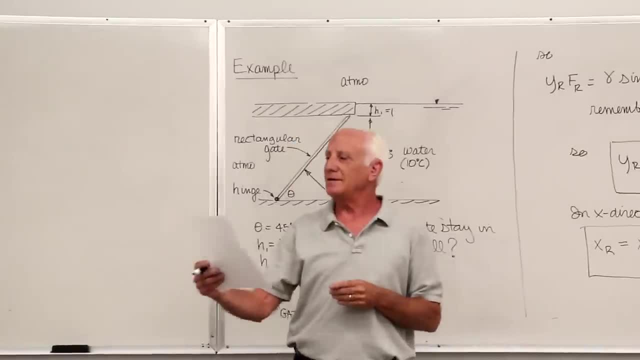 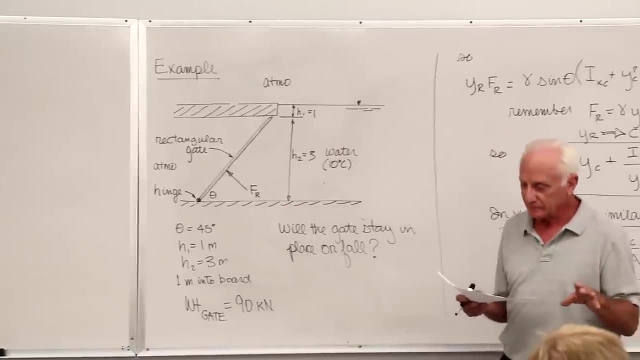 So I'll say where's set nine, Say right here: Oh yeah, I did check it, I'm sorry, So that'll help me and you if there's a grade problem with your homework later on, Okay, final thing. 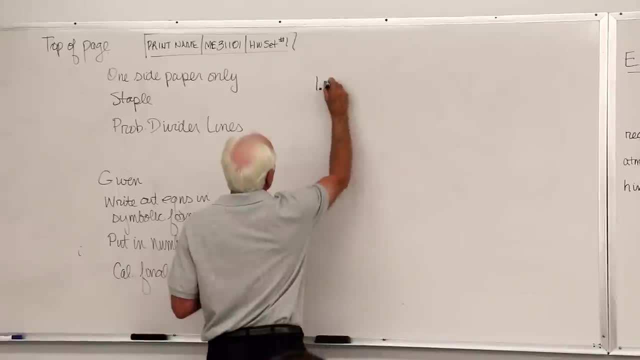 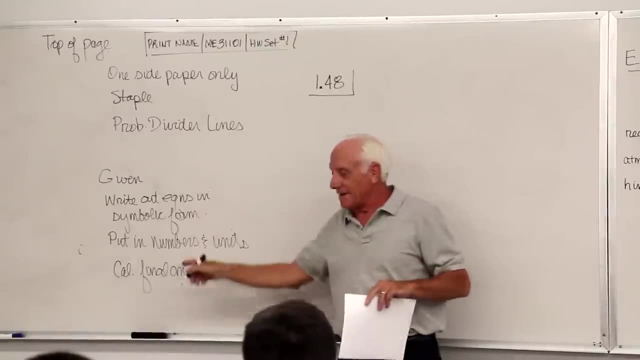 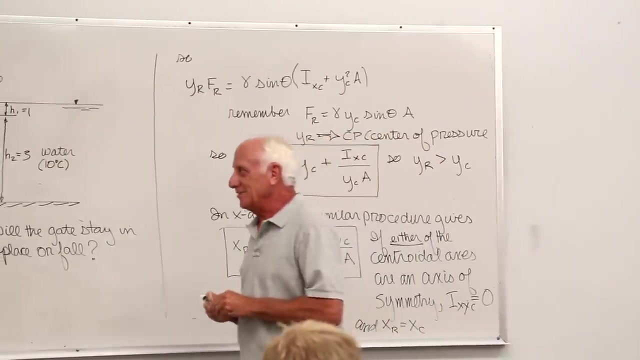 Let's just take as an example problem 148.. By the way, why does this stuff help? Oh, it helps dramatically. Number one, the main reason why it helps: I don't want to just make work stuff, But I'm trying to help you get ready for exams. 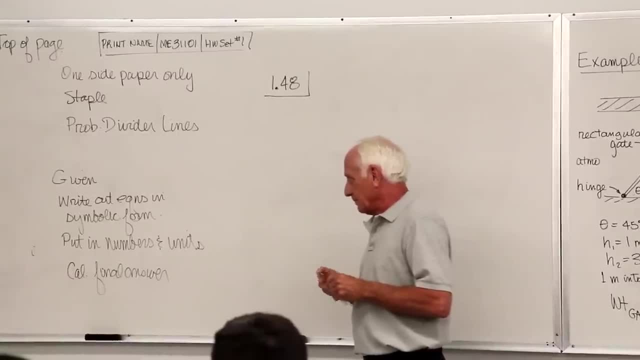 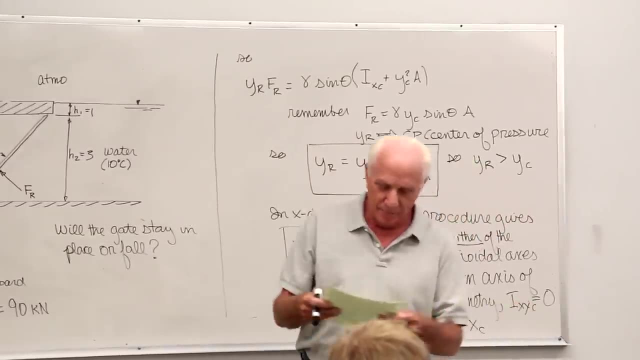 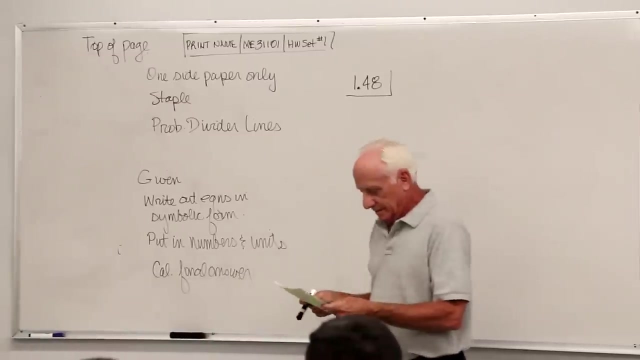 and especially the final. Because for the final, when you're trying to get ready for the final and somebody just starts putting numbers in without even realizing it And you're trying to write the equation down or what's given, What you're doing is you have to pull out the textbook. 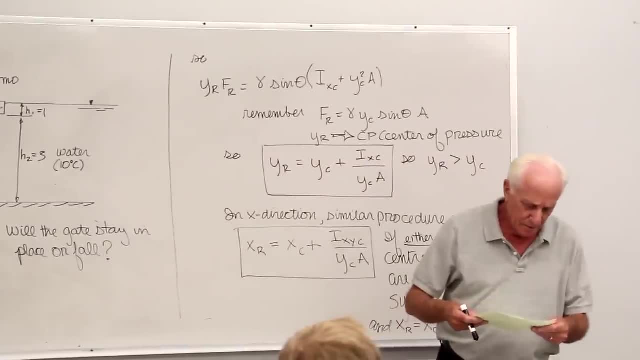 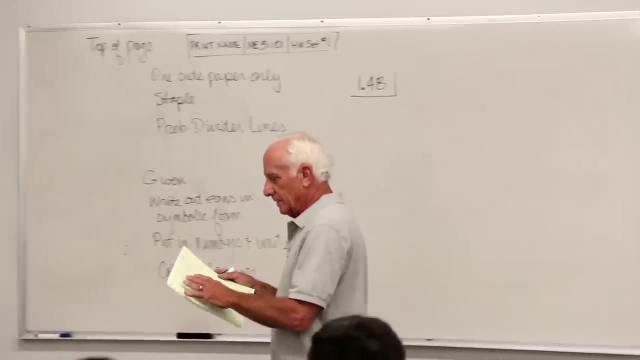 And you have to find problem 180.. If you put it on here, do you save time studying for a final? Why I'll say you do. And when's the toughest time of the quarter? The 9th and 10th weeks, of course. 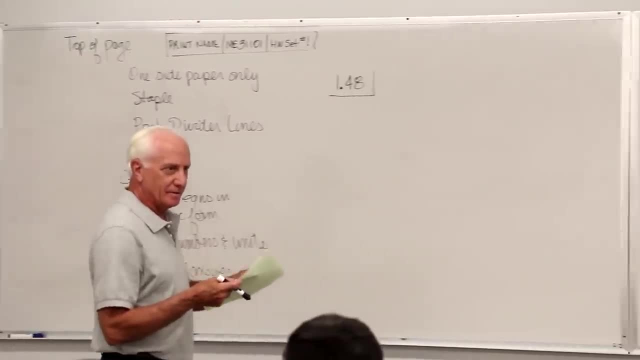 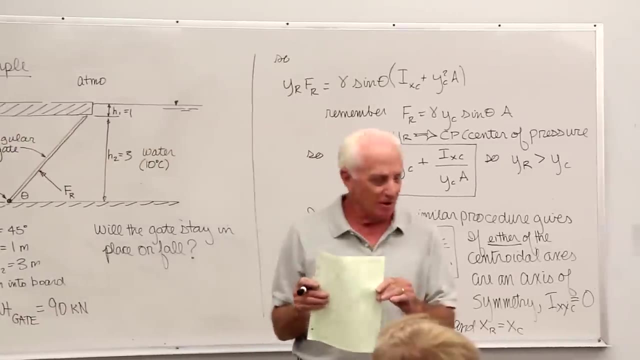 One of you is stressed out because your final's Monday, which yours, is the 9th and 10th weeks, of course. So the point being, if it's all here, you have saved yourself tons of time rather than frantically fumbling around here trying. 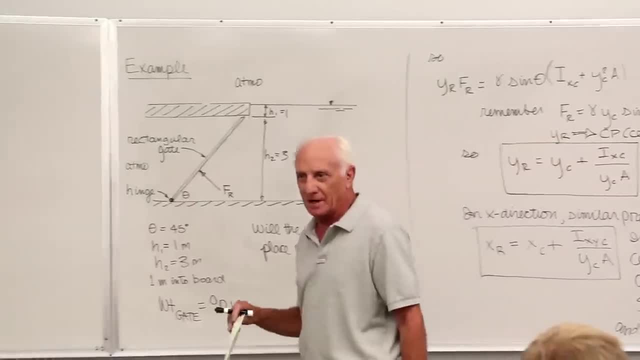 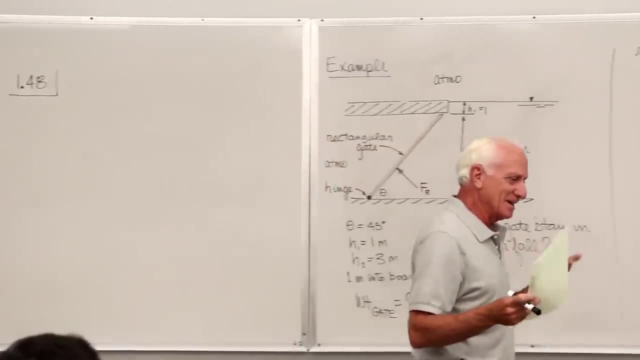 to find a particular problem on your laptop or on your smartphone, whatever. Okay. so it really pays big dividends to you. Me a little bit. I have to see neat work. that's what engineering's all about. You know, inventors can be messy. 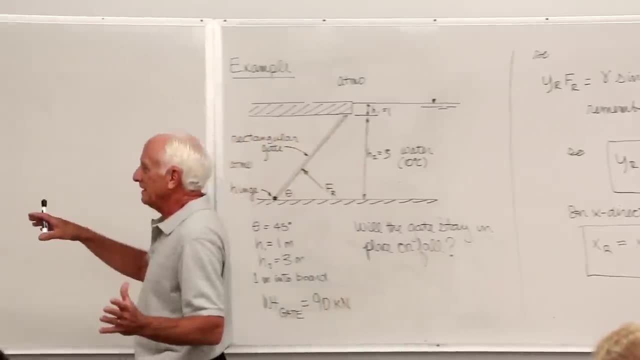 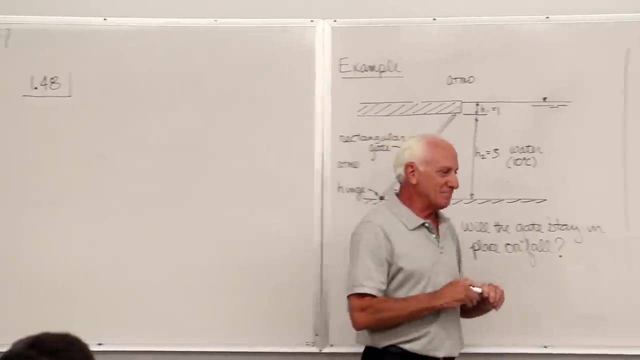 Engineers are neat in their work. So, yeah, it helps you study for midterm, but especially eight weeks from now, which is final exam time. Okay, problem 148.. I'm just going to go through one and show you what I mean by that. 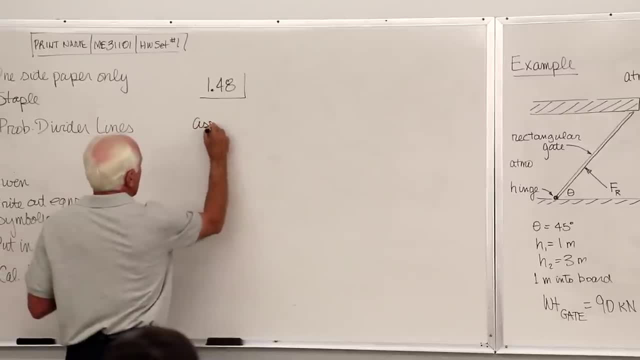 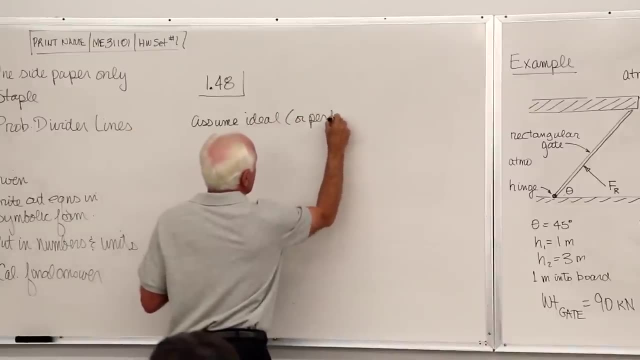 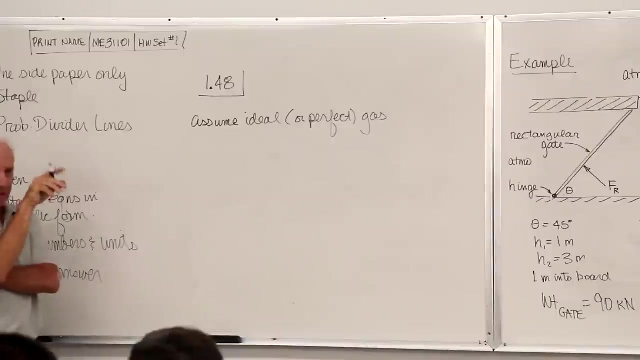 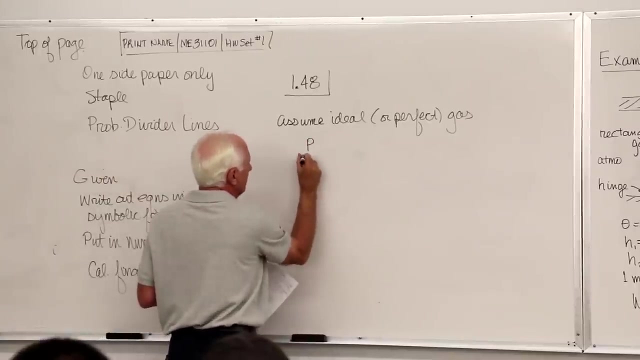 You say: okay, this is, I'm going to assume, an ideal gas. Our author uses both names. He does that. He said in chapter one: ideal parentheses are perfect gas. That means a gas that obeys this equation: P over rho, equal R, T. We're supposed to solve. 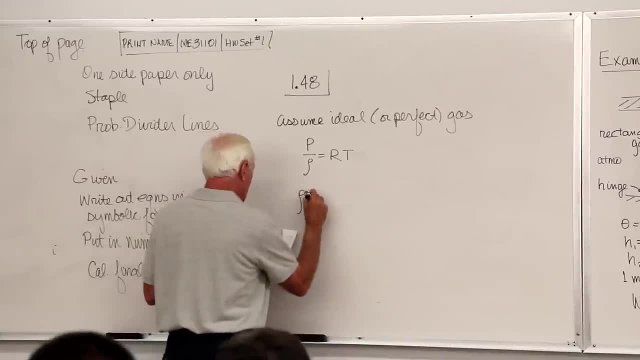 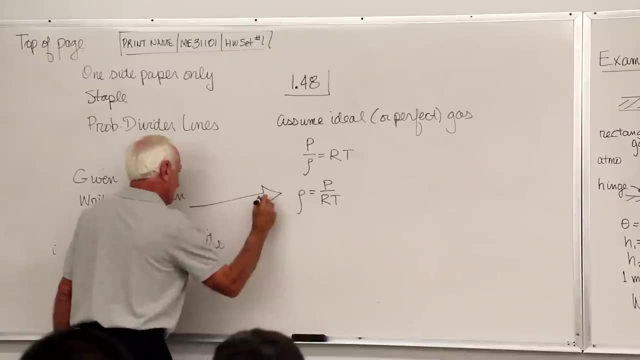 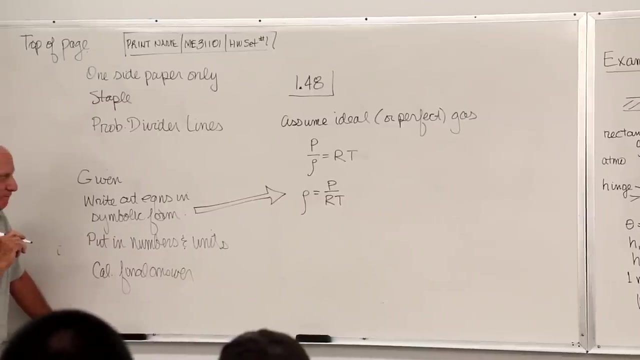 for the density of the problem. Okay, rho is equal to P over R T. That's what this means. Don't put any numbers in first. Write the equation out in symbolic terms: symbols, no numbers. Then you can write the given. 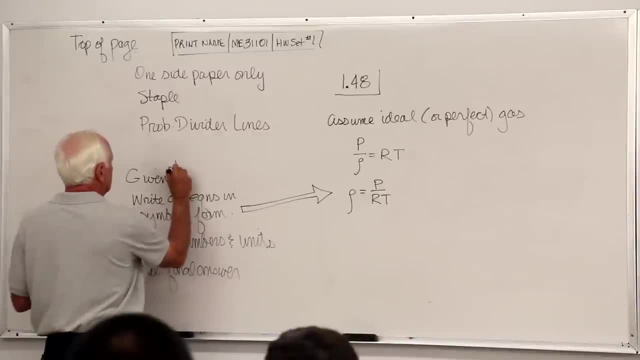 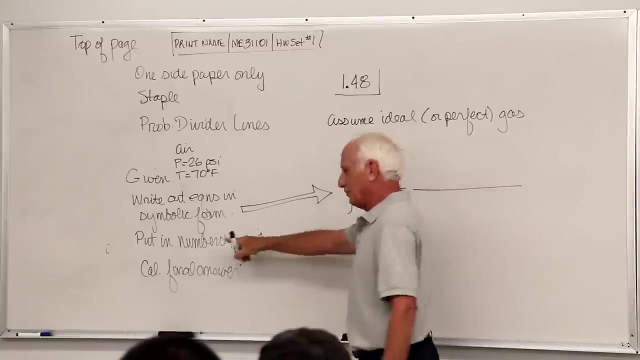 The given was pressure 26 PSI. The given was the temperature is 70 Fahrenheit, and et cetera. The gas was air. Okay, These are all givens. Okay, now we do what it says here. Put in the numbers in units. 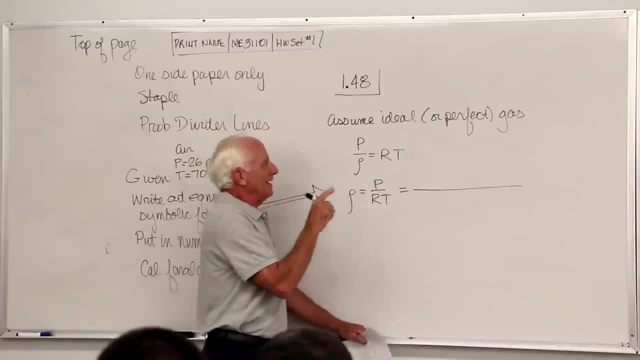 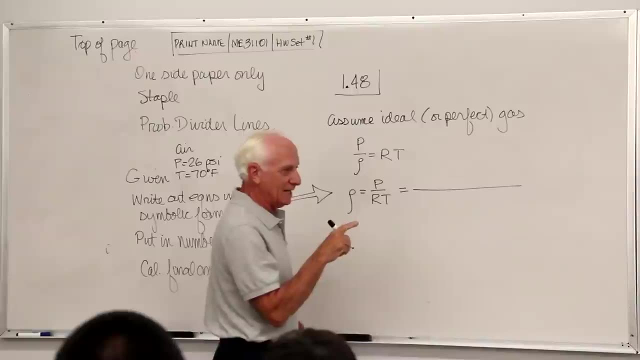 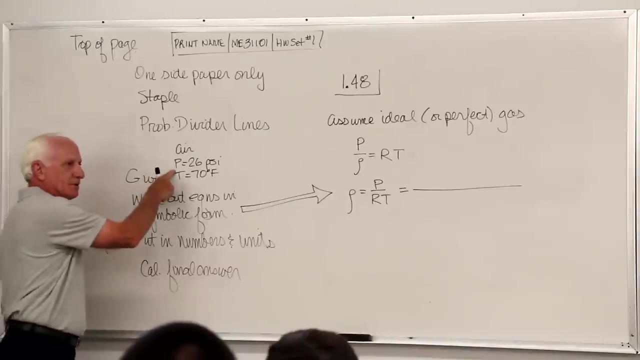 But be careful, because we know, you know, that the ideal gas equation state, the pressure and temperature, must be put in in absolute terms. Okay, what's that mean? It means if it's gauge pressure, add 14.7.. The problem said this pressure. it said the gauge pressure was that. 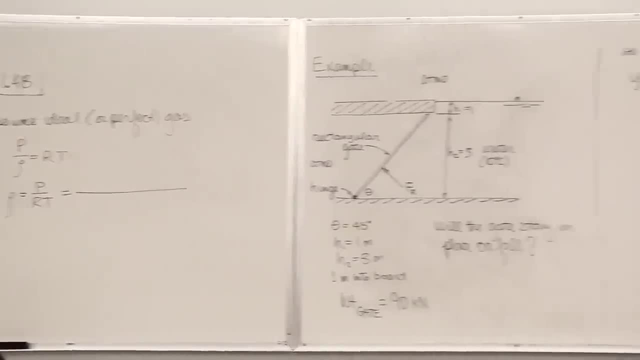 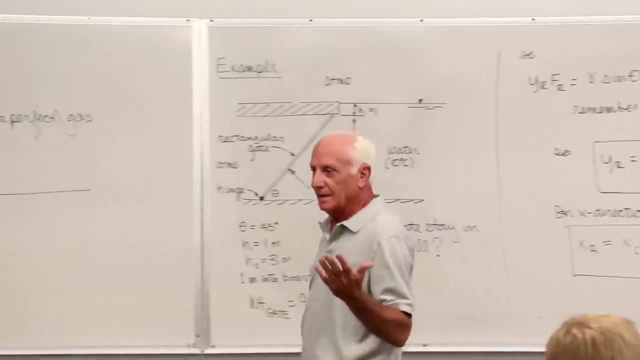 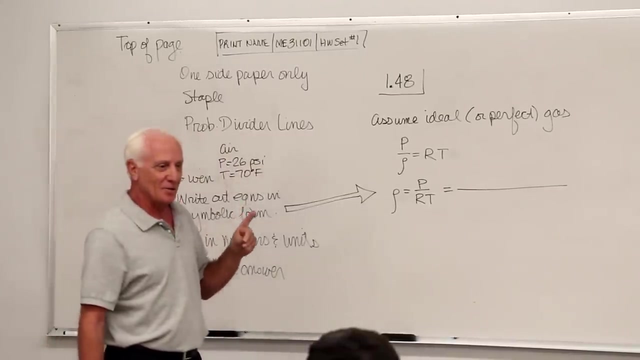 Let's just see Problem 148,. a tire has a gauge pressure. He said it. Now here's the problem. Here's the default rule. Remember the default rule? The default rule was we always assume the pressure is given or gauged and is otherwise specified. 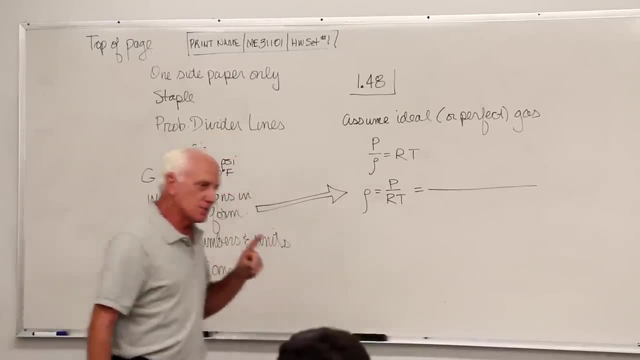 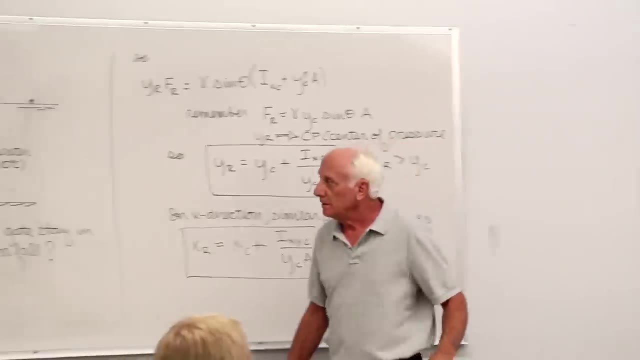 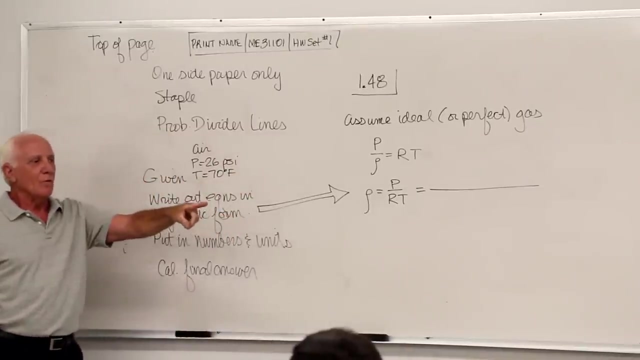 So even if he hadn't said gauge pressure, did he put PSIG or PSIA after it? No, he didn't. He said PSI. So how are you supposed to know if it's gauge or absolute? Well, he told you. 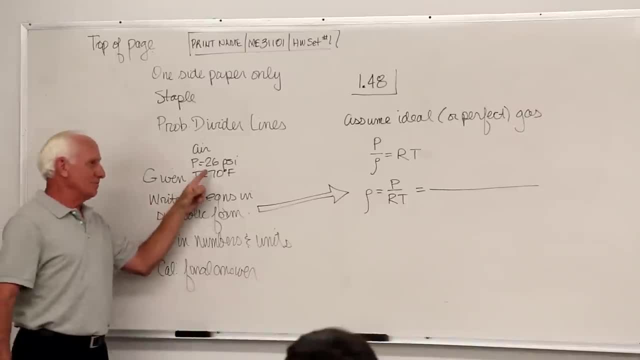 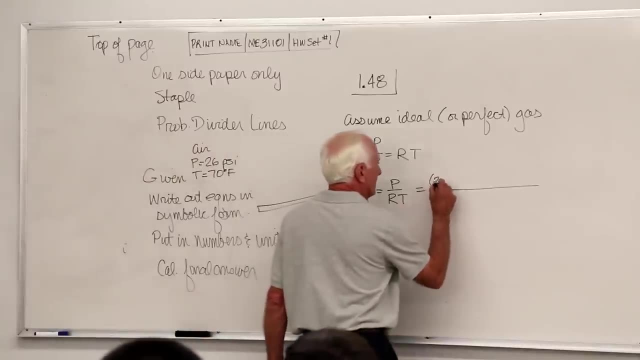 What if he didn't tell me: Default rule is always assume gauge. Default rule is always assume gauge, And thus told otherwise. Okay, so now you know how to handle that. 26 plus 14.7.. Units: pounds per square inch. 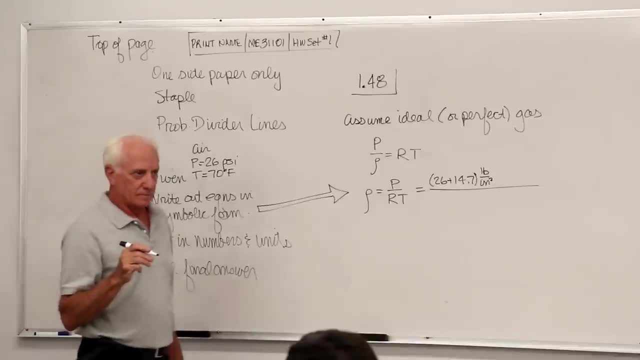 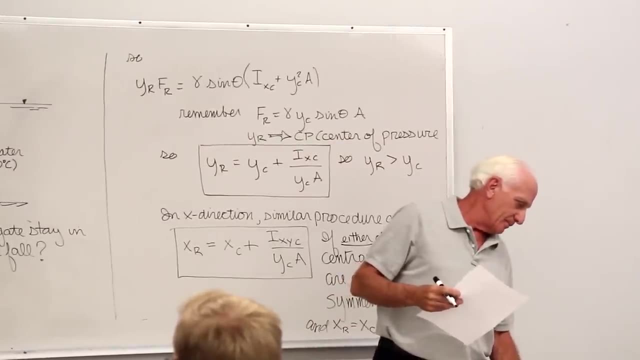 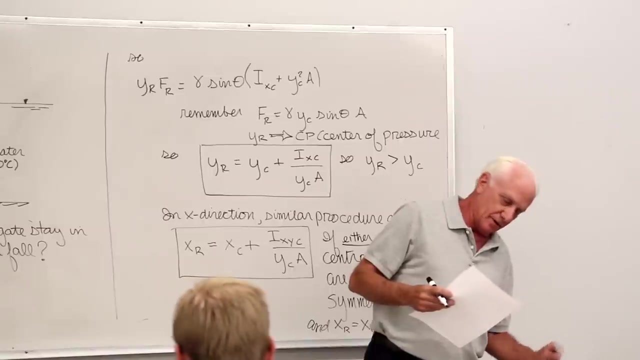 R. R is the gas constant. It's a constant. Where do you find it? Inside the front cover. Okay, There, it is. Okay, There it is R gas constant, Table 1-7.. Inside front cover. 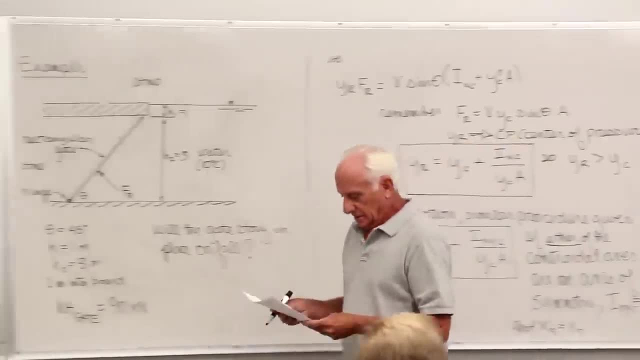 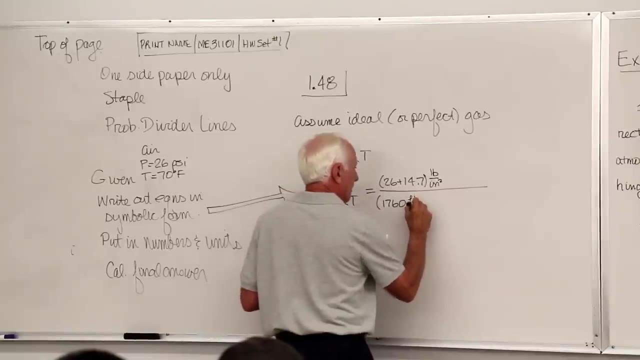 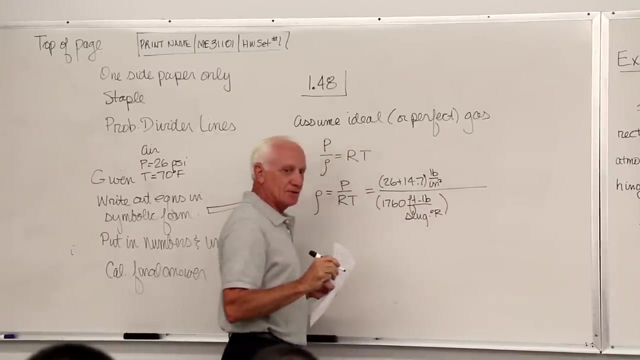 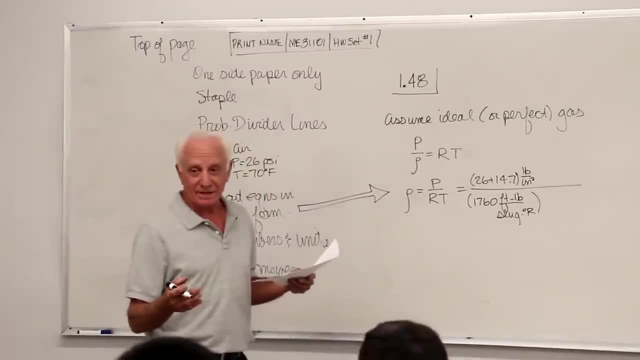 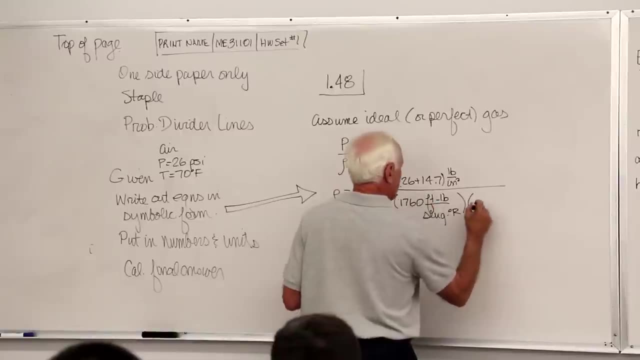 If it's degrees F, add 460 to get the degrees K. I agree with R, pardon me, 460.. Temperature: 70.. Don't go through, as some people did, an intermediate calculation and waste valuable time on a mid-term. 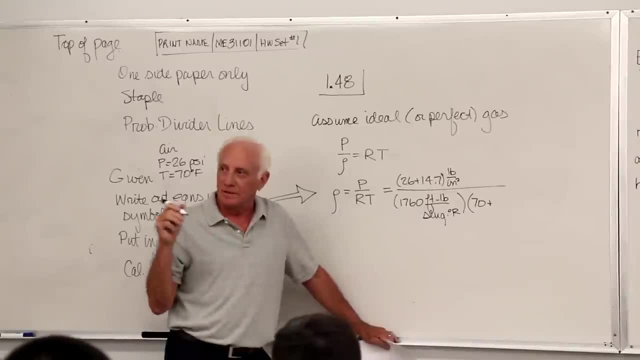 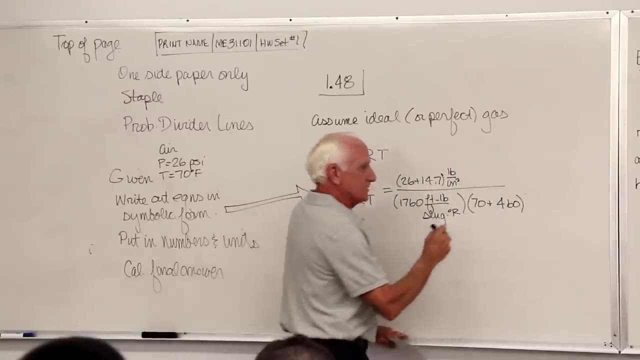 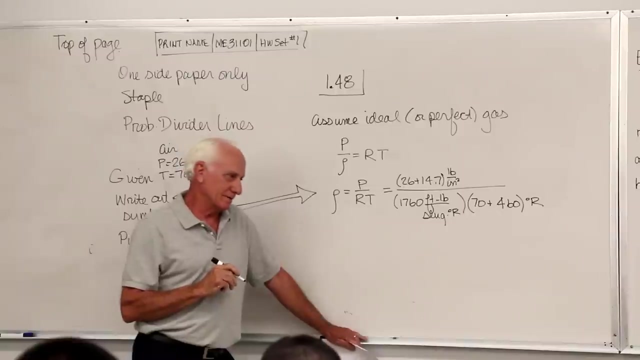 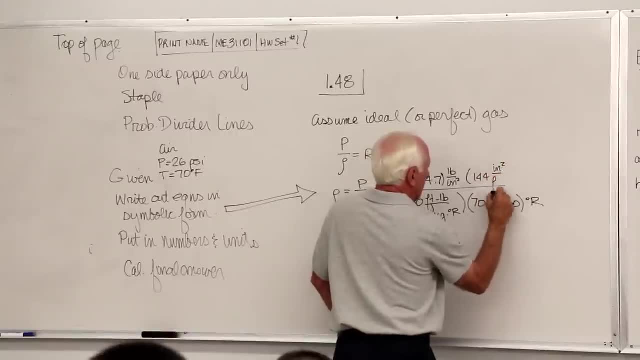 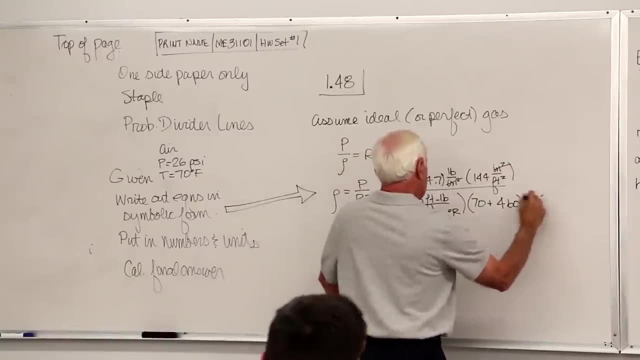 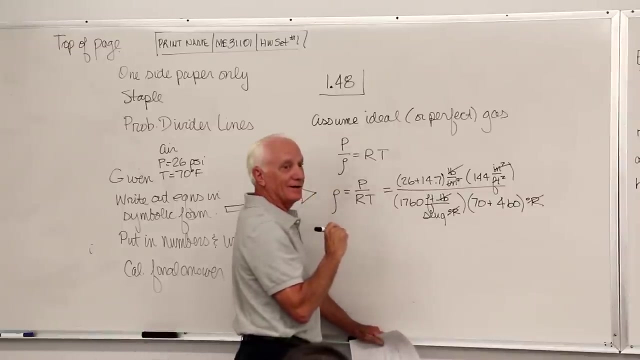 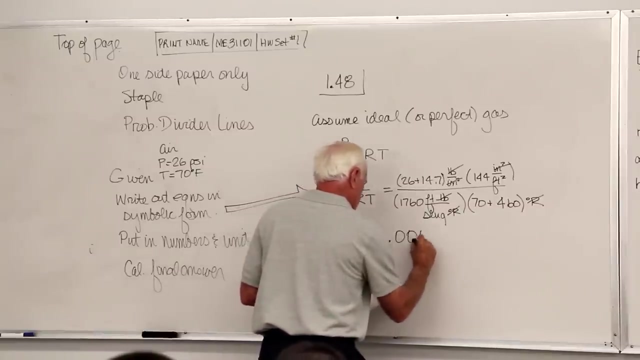 144 square inches per square foot. Cancel, Cancel. Uh, here we are. Cancel, Cancel, Pound, Cancel, Cancel. Ah good, Slugs per cubic foot. That's density 0.00644 slugs per cubic foot.